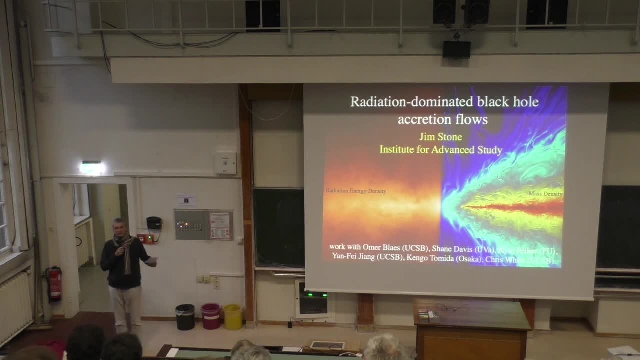 of two, or co-author of two, of the very prominent workhorses we all use in computational astrophysics studies. One is SUSE, and SUSE is a bit outdated, I would say, for many applications. I shouldn't say that- And the really new thing that he has been working on and developing for the 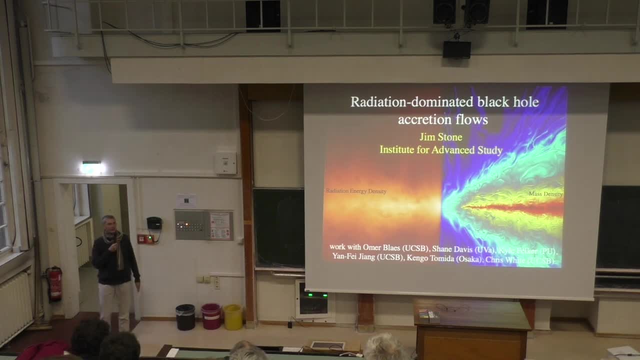 past decade, or maybe 15 years or so, is Athena, and the latest version is Athena++, which can do many, many things that we are all dreaming of with our standard codes, And I'm sure we will get a glimpse of what this code can be doing when applied to this. 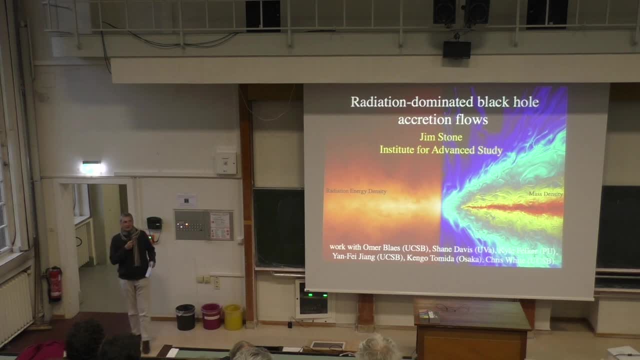 application. So, despite his prominence in this field, let me say a few words about how he came to be there. He started in Kingston, Ontario. He got his bachelor and master from Queen's University there. He then moved just south to the University of Illinois where he was working at the National 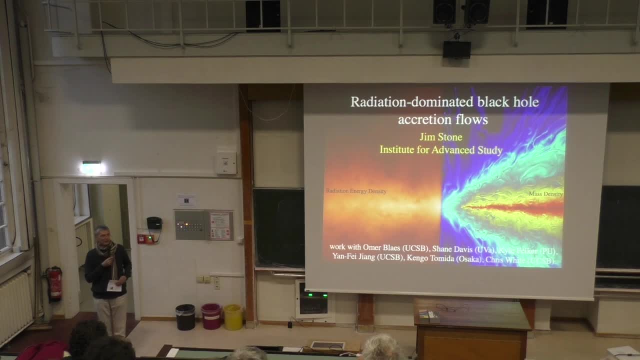 Super Computing Center with Mike Norman, So he finished his PhD there in 1990.. And then he moved to the University of Maryland where he became a professor of astronomy in 2001.. He then spent an interim's time as Professor in Kennedy University, working with former 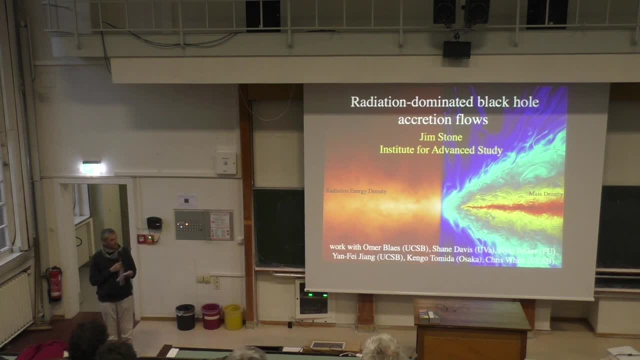 Professor of Mathematical Physics at the University of Cambridge. that was in 2002 and 2003.. And then he came back to the US where he went to the Princeton Institute for Computer Science and Engineering first, and then to Princeton University to the Department of Astrophysical. 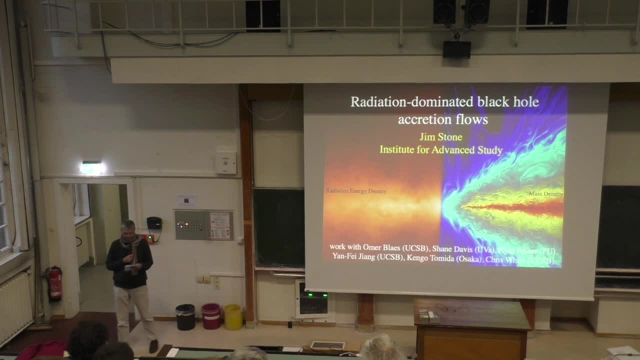 Sciences and he was Chair and Lyman Spitzer Junior Professor for Theoretical Astrophysics from 2016 to 19.. And since June or July 1st 2019 he moved a bit further out to the Institute of Advanced Studies in Princeton and he's now professor at this institution. 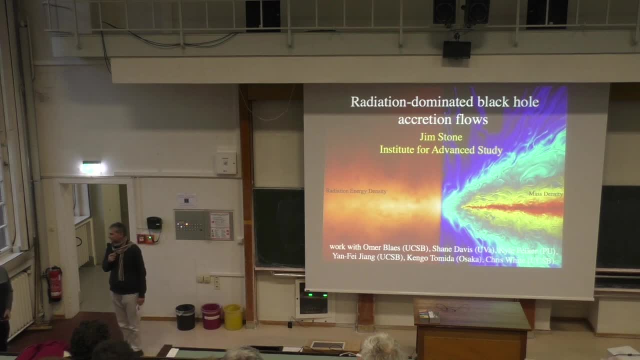 So I will now close and let's welcome again Jim- and look forward to learn about how black holes agreed. Thank you very much, Ralph. It's a great pleasure to be back in Heidelberg again, although this is the first time. I've visited the University- previously been here for meetings or other events- so it's a great. 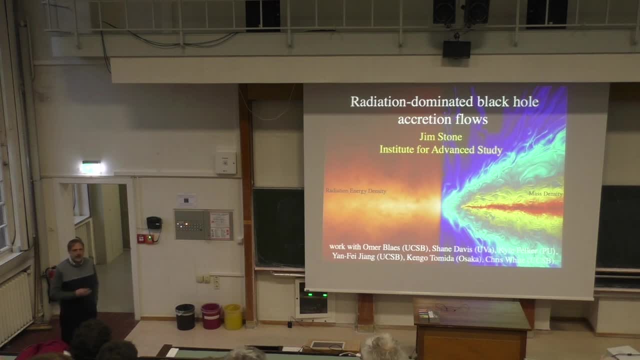 pleasure to be here. There's so much astronomy going on here with so many institutes. it's been a very busy couple of days catching up with people, but I've really enjoyed it. I think Heidelberg must be one of the centers for astrophysics. 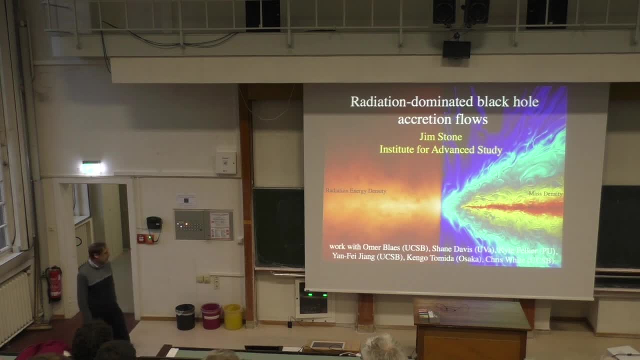 Astrophysics in Europe, given the activity going on here. so it's been really, really enjoyable. They warned me the lecture hall was very steep. the chairs are uncomfortable. It is steep. I'm getting a little motion sickness here. looking way back up here to, in fact, the youngest 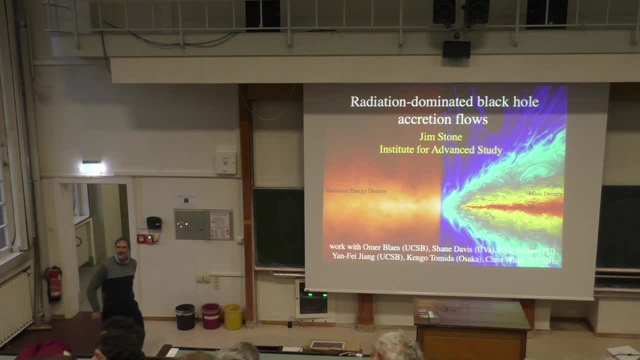 member I've ever seen attend one of my colloquia Must be only a year and a half. so that's fun. There we go. I'll try to keep it simple so that everyone can understand it. So I wanted to tell you a little bit about 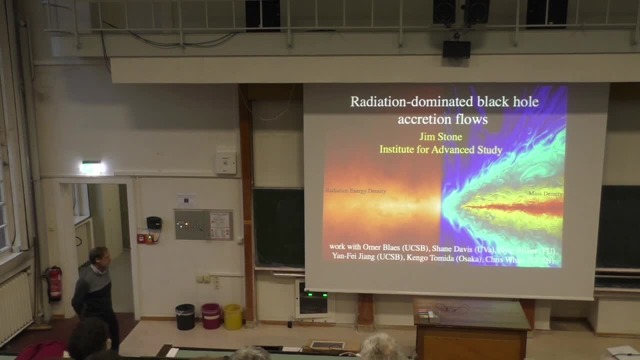 Some recent work we've been doing on black hole accretion flows. This, to be clear, is work I've done with a large number of collaborators, including some very, very good students and post-docs who have been at Princeton. So, for example, Shane Davis was a post-doc, Kyle Falker was a student in the applied math. 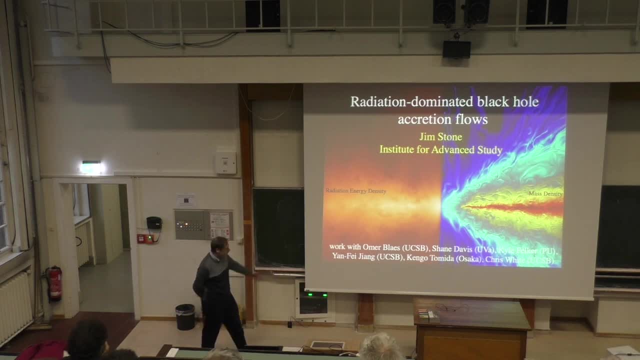 program. Yanfei Zhang and Chris White were also both students, and Kengo Tomita is now a professor in Osaka University and was a post-doc at Princeton. So they've all contributed very, very significantly this work And I'm going to try to explain. 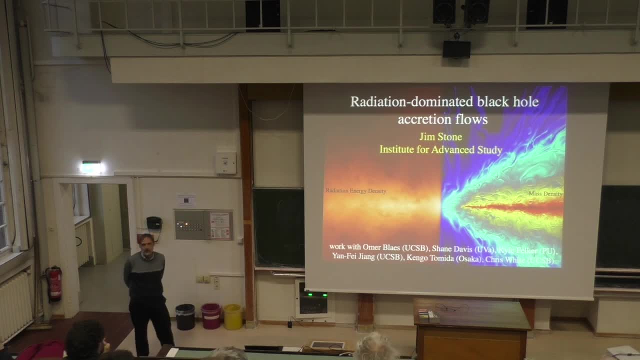 I'm going to try to explain to you the image that's on the background here, which is a snapshot of a time-dependent black hole accretion flow in which the radiation field is very dominant and contributing significantly to the dynamics. Please feel free to interrupt me if I'm going too fast or if you have questions. 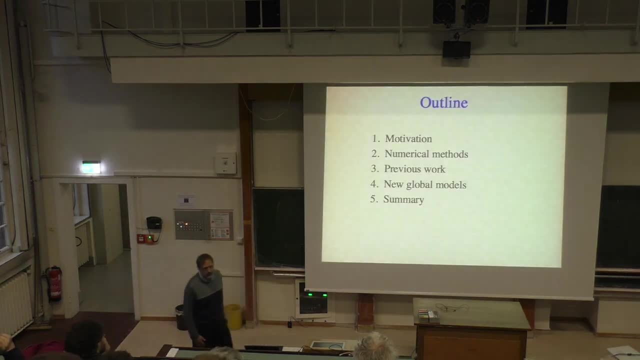 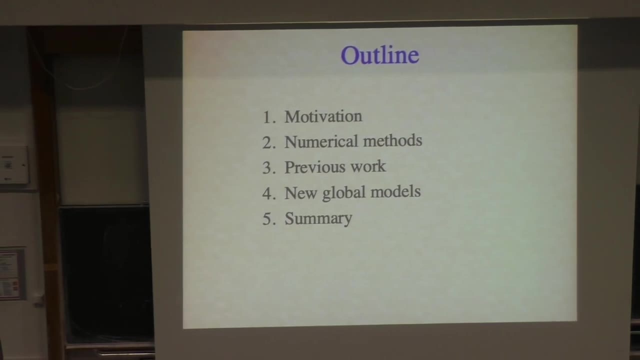 I would be happy to answer questions as we go along. So let me start with the motivation of why we want to study this problem. Let me tell you a little bit about the numerical methods. indeed, as Ralph said, these calculations can only be enabled using numerical methods. 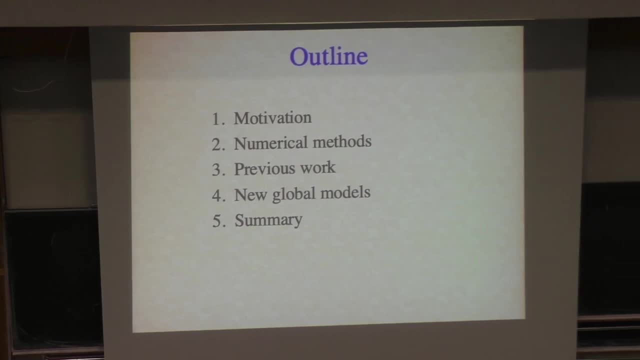 And I should at least tell you what we're doing there. I'll briefly tell you a little bit about what's been done previously and then move on to the new results we have on fully global models of accretion flows in this regime. 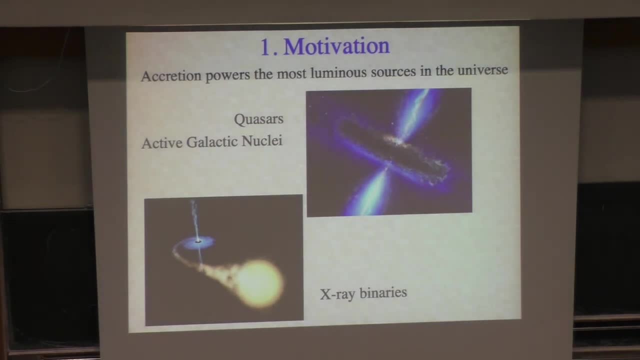 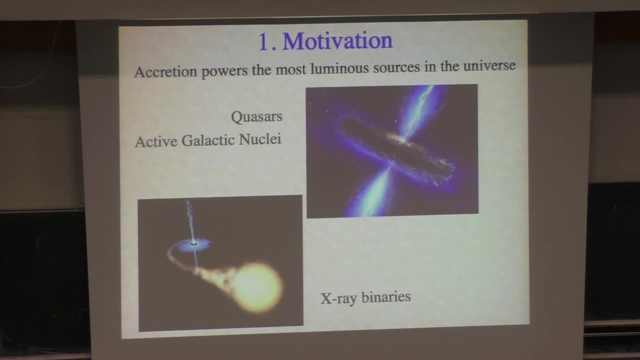 So, of course, the simplest motivation for why study these flows is because they're so important in astrophysics. All of the most luminous sources in the universe are powered by accretion, and accretion onto compact objects like black holes is a much more efficient way to release energy than 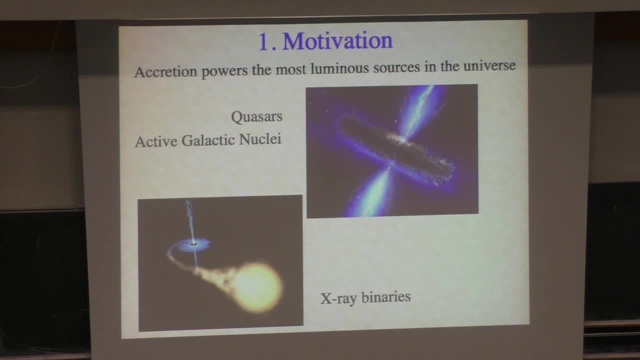 say nuclear fusion, Which is what powers most stars. So things like quasars are powered by accretion onto supermassive black holes, Or X-ray binaries is powered by accretion onto stellar-mass black holes. So if we want to understand these sources and we want to understand their evolution, 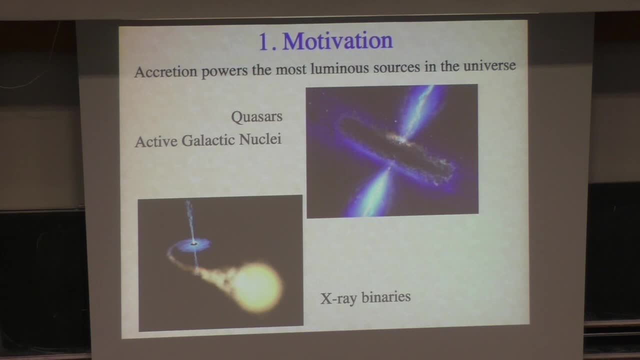 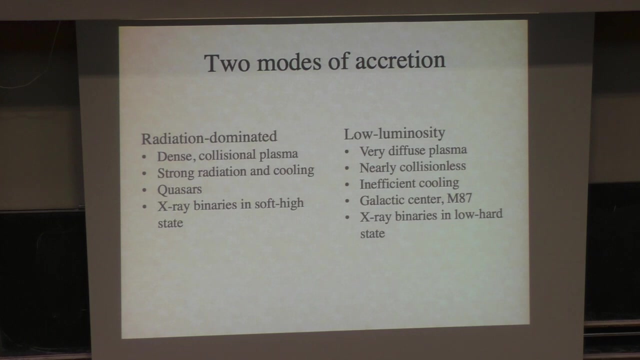 and the evolution of black holes in the universe, how they grow from seeds in the early universe into the supermassive objects we see today. we need to understand these accretion processes which can significantly change their mass over time. There are two modes of accretion I think that most astrophysicists talk about today. 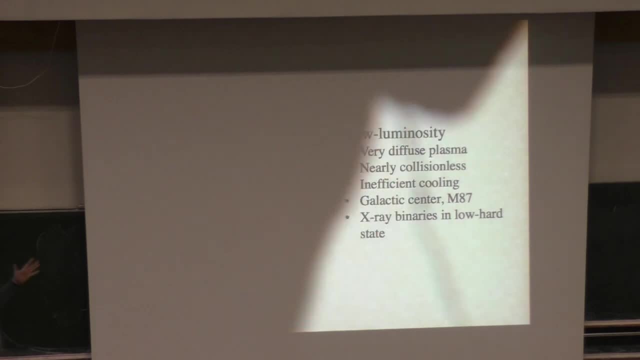 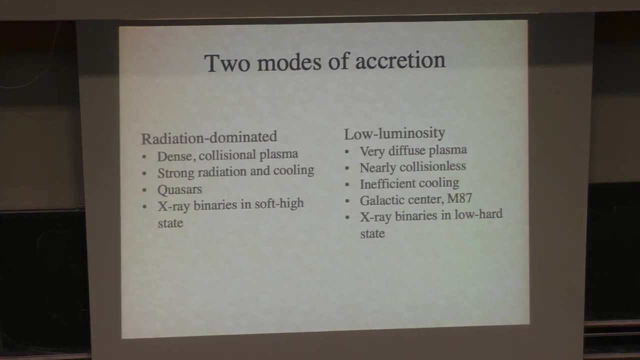 One is a radiation-dominated mode where the plasma is very dense, fully collisional, so that you can treat it like a continuum, so you can treat it like a fluid. You can use the equations of magnetohydrodynamics to describe it in this regime. 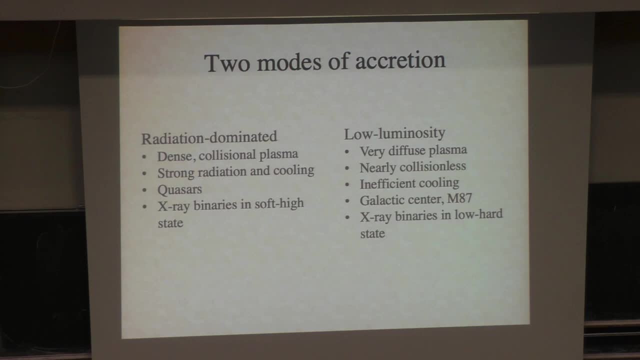 Their strong radiation is very important. The energy density in the photons greatly exceeds the energy density in the thermal particles, So modeling the radiation is absolutely crucial. And in this regime are quasars and X-ray binaries in their so-called soft high state. 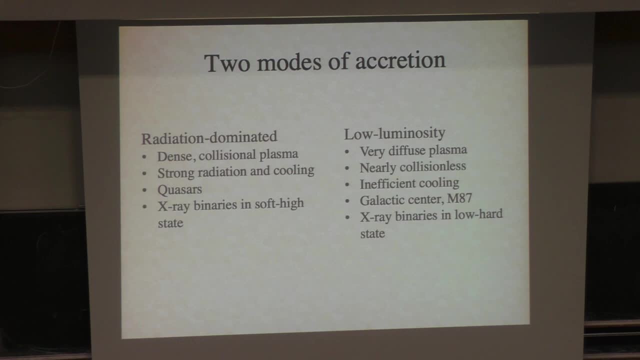 A very different regime is the so-called low luminosity accretion flows. Those are powered by very, very diffuse plasma. So in that case the mean free path of the particles in the plasma may be comparable to the size of the event horizon of the black hole at the center. 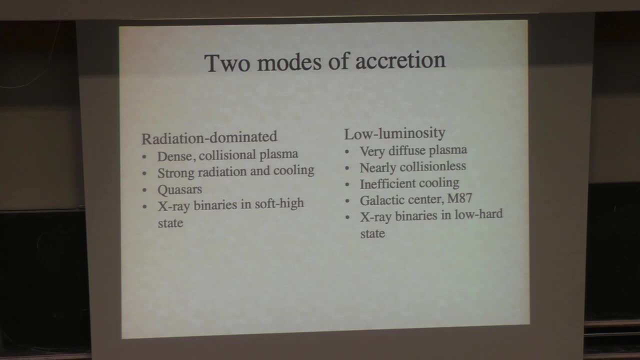 So it's very weakly collisional, nearly collisional, Less you need to include kinetic effects in the plasma. You may need to even treat it as a completely collision-less plasma in that regime, Because there's so few collisions, there's very little radiation generated. 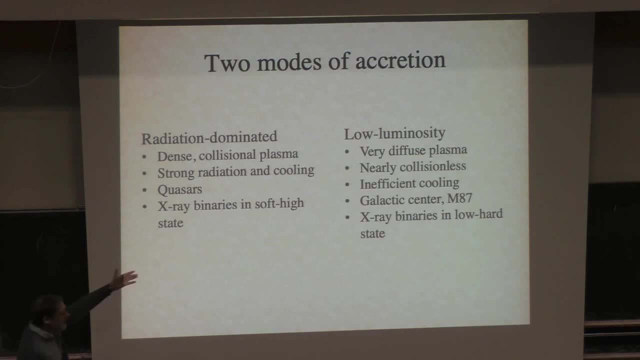 So there's very inefficient cooling And objects like the galactic center and M87, nearby supermassive black hole and external galaxy are in this regime. So luminosities- for those astronomers who know Eddington units, so luminosities are. 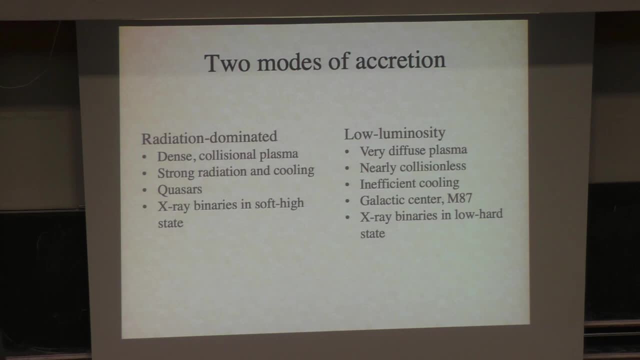 10 to the minus 5 Eddington or smaller. So I'm really going to be talking about this radiation-dominated regime today and not so much about the Loon-Lossy now. Unfortunately, the Event Horizon Telescope, which recently reported such a beautiful image, 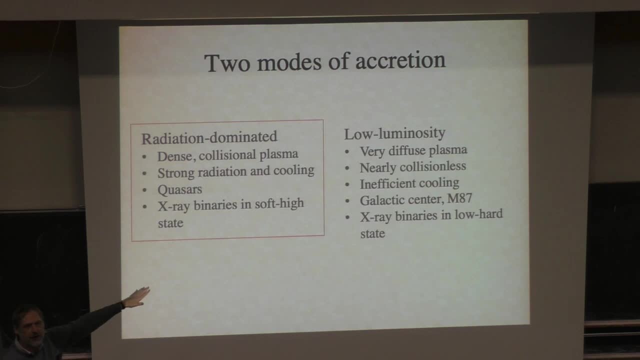 was for M87. And so it's in this low luminosity phase. I'm not really going to say anything about the image taken of M87.. I'm going to be focusing more on the physics in this high luminosity phase And there's a bunch of motivating questions from the observational side as well. 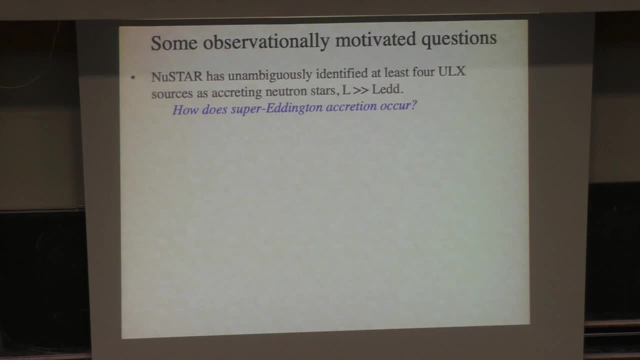 So, for example, a recent satellite mission called NuSTAR, an X-ray telescope, has identified so-called ultra-luminous X-ray sources, ULXs, as being accreting neutron stars, meaning that their luminosity is much bigger than Eddington. 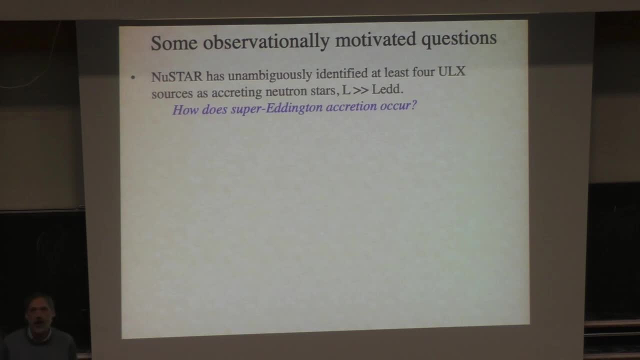 Again. I'll define this Eddington luminosity in just a minute. But basically it's the highest luminosity that a spherical accretion flow could have. So nonetheless we observe these flows at higher than that luminosity. How is that possible? 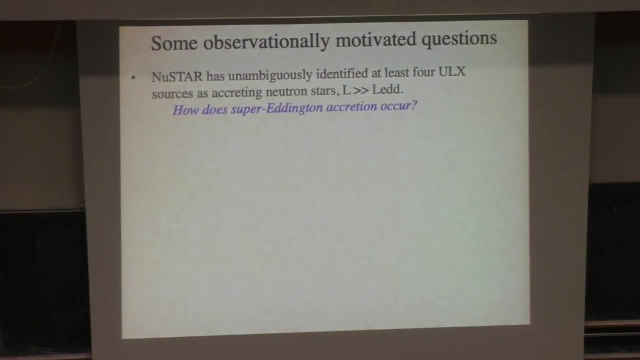 This is truly a breakthrough, because previously it was thought that these sources were much more massive black holes and therefore their luminosity was not super-Eddington, But the discovery that they're actually neutron stars unambiguously shows that many of these 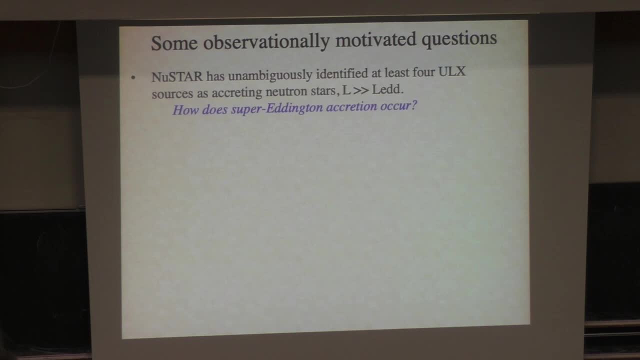 sources are accreting at super-Eddington, And so just how does that happen? How can you accrete matter when the radiation force is exceeding the force of gravity? Secondly, we know from spectra that disks do not just have a thermal spectrum. 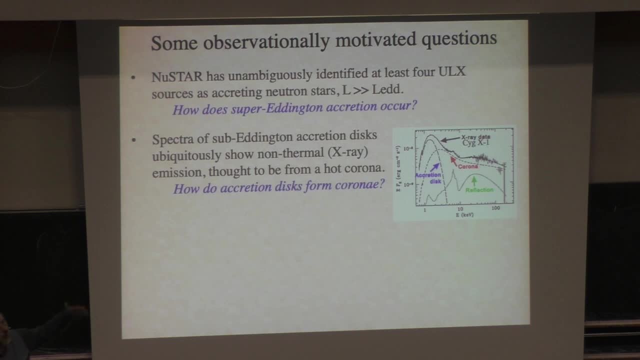 In fact they have this very significant contribution from non-thermal radiation elsewhere in the flow. So, for example, the spectrum of a classic accreting stellar mass black holes, the so-called Cygnus X1 source in our own galaxy, shows this nice thermal radiation bump marked by 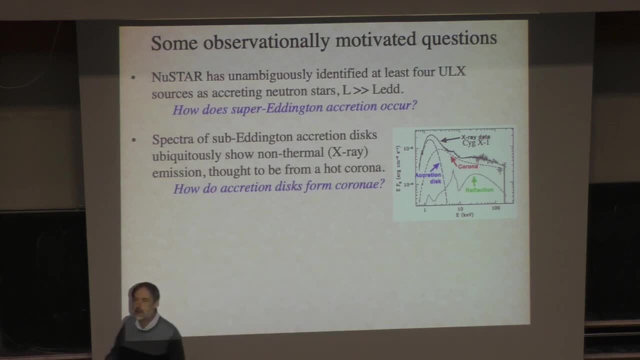 the blue curve there. That's just the accretion disk itself, the dense part of the disk. But in addition there's a component at high energies which is sort of a power law tale. at high energies, Due to very, very hot plasma thought to be in a corona, again, in sort of analogy to 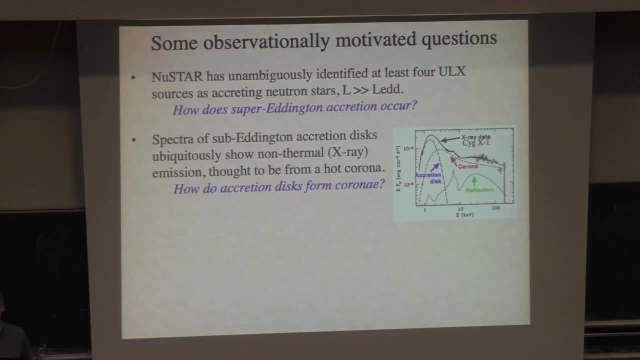 the sun, which has this very hot plasma, a million degree plasma, above its surface. somehow the accretion disk is forming extremely hot plasma above the midplane and generating this mixed spectrum of accretion disk plus corona and also reflection of the coronal photons. 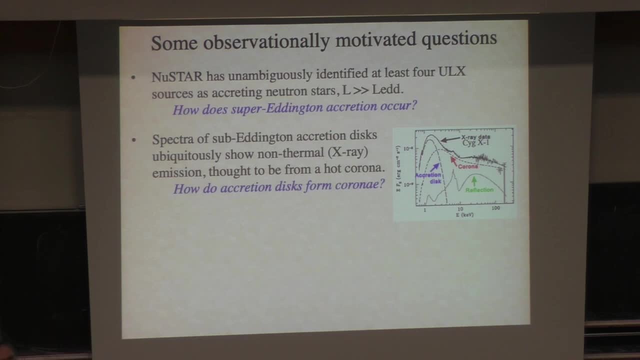 off. the disk itself is very important. So how does that work? How do accretion disks form corona? This is already a complicated question for the sun. Is this the same mechanism? Is this the same mechanism that works in accretion disks as heats the solar corona? 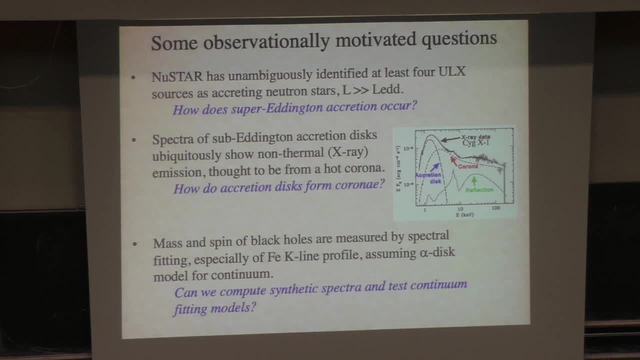 We'd like to understand that. And then, finally, these spectral modeling is extremely important because if we want to measure the actual properties of black holes, we can never really observe them directly. All we see is the plasma that they're accreting. 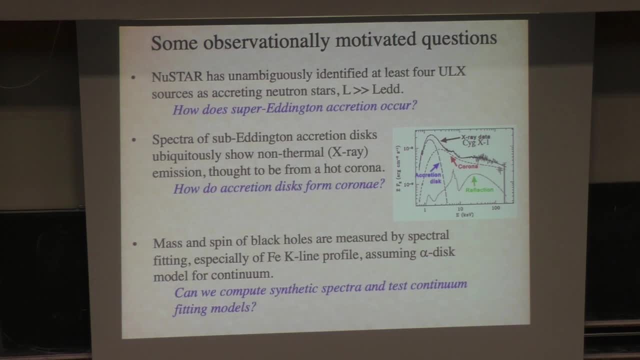 We see the plasma as it's falling into the black hole And therefore we need to understand what produces the photons there very accurately so we can take a theoretical model. We can take a theoretical model of the infalling spectrum or the spectrum of the infalling. 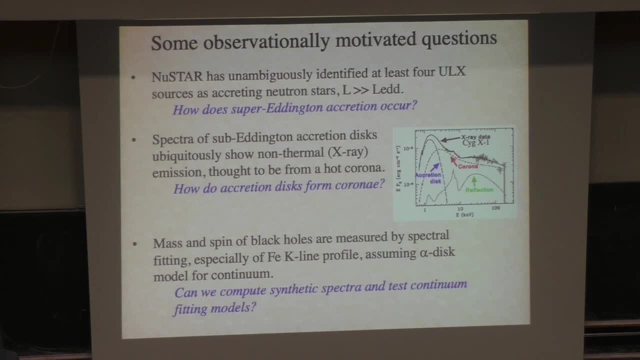 plasma and extract things like the properties of the black hole, its mass, its spin and other things, And this requires a very, very accurate sort of prediction for what the spectrum for an accreting black hole should look like. Right now our predictions, I would say, are not so necessarily accurate. 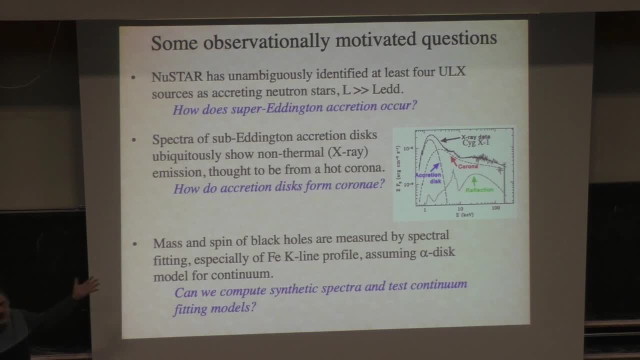 They're based on so-called alpha disk models with a very simple model for the continuum. We'd like to try to improve that. Can we do better? Can we do better? Can we predict these spectra from first principles in order to be able to use the spectra of? 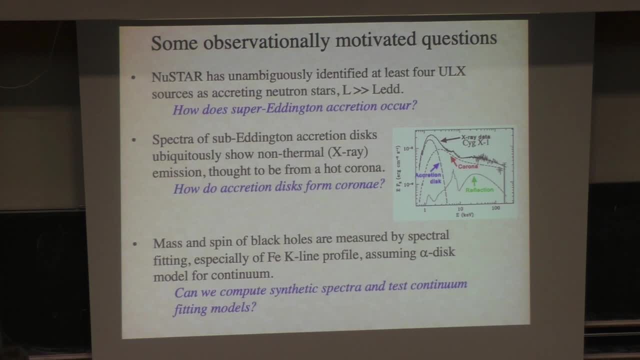 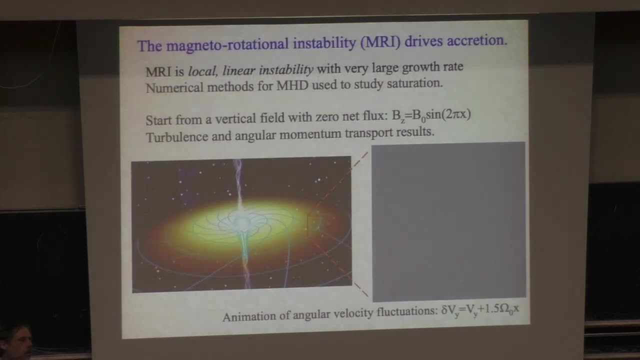 accreting black hole to measure directly things like spin, mass and other properties. So those are some of the motivating questions that we're trying to address. So suppose we want to study this problem. We want to study theoretically accretion on the black holes. 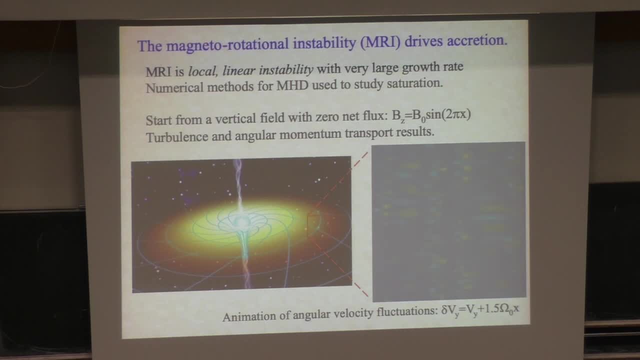 What do we need? The first thing we have to remember is that accretion itself is being driven by magnetohydrodynamic processes, In particular the so-called magnetorotational instability, the MRI Right. So a magnetized plasma that's in orbit around a central object and has a background shear. 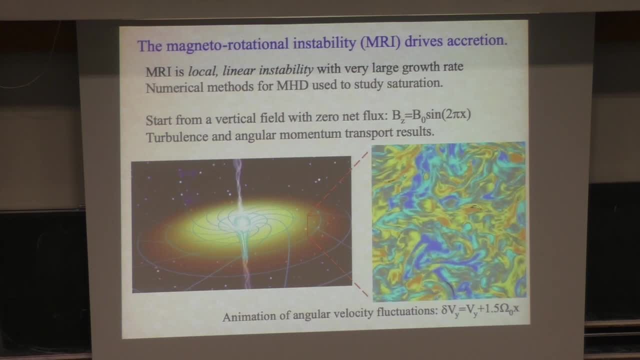 profile like Keplerian. a rotationally supported Keplerian flow is known to be linearly unstable to small amplitude perturbations in MHD, And those small amplitude perturbations grow into turbulence And this is known for now 20 years through nonlinear MHD simulations of the growth and 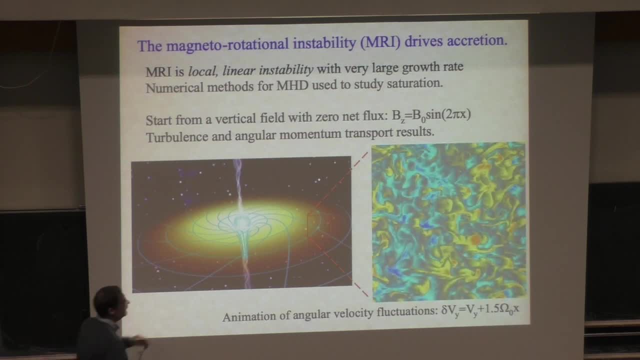 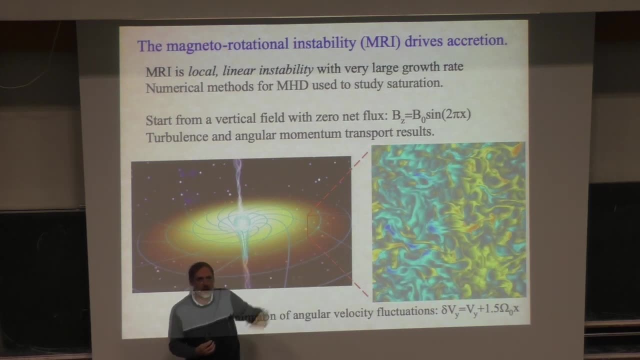 saturation of the MRI Right. And this movie shows an example of taking a small little patch of a much larger accretion disk, simulating the MHD or solving the MHD equations in that small little patch and watching the MHD modes emerge. 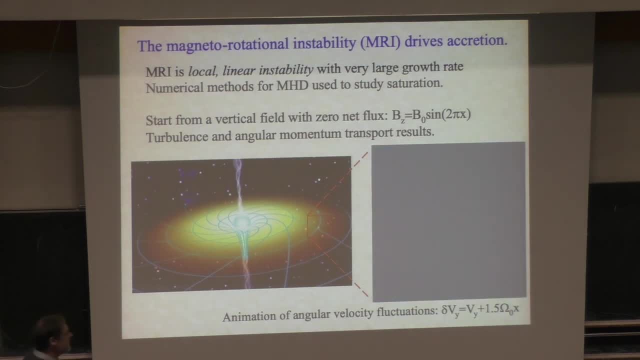 So let me just sort of play it again one more time here. What you're watching are the angular velocity fluctuations in the background flow. So initially there's zero, Everything is Keplerian. And then you see the linear modes of the MRI pop out from small amplitude perturbations. 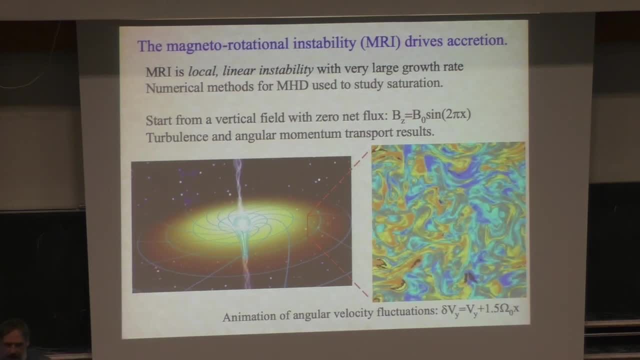 And then it transitions into turbulence, And this turbulence has a large Maxwell stress associated with it, And that stress transports angular momentum outwards, And so the MRI is now recognized to be the mechanism that transports angular momentum outwards and allows matter to accrete inwards in fully ionized plasmas, like accretion flows. 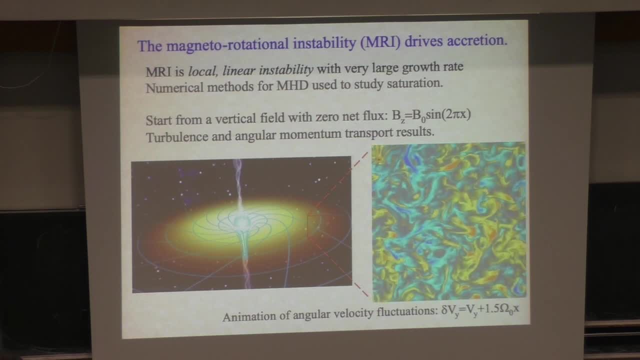 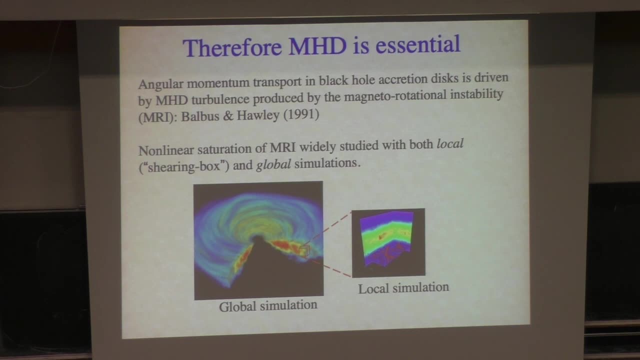 around black holes. So there's been a huge amount of work and I could give a whole conference on what we understand about the MRI today, But there's been a huge amount of work. But the point here is that if you're going to study black hole accretion flows, you need 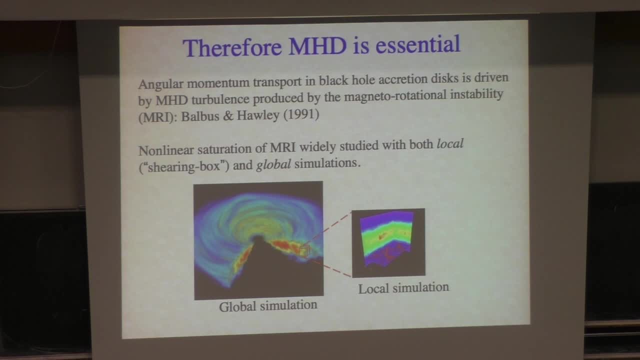 to include MHD, Or you're not going to capture the most basic dynamics, which is what drives accretion in the first place. So the very first thing you need to at least include is a magneto-hydrodynamical model. 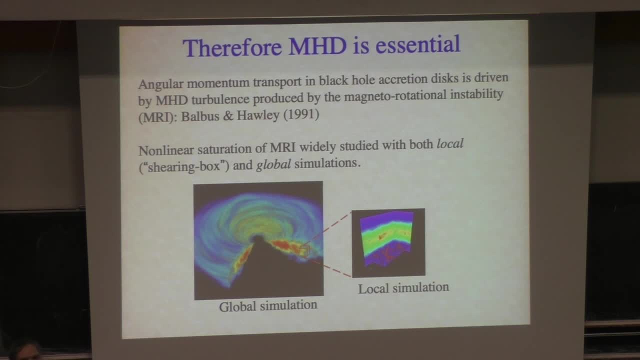 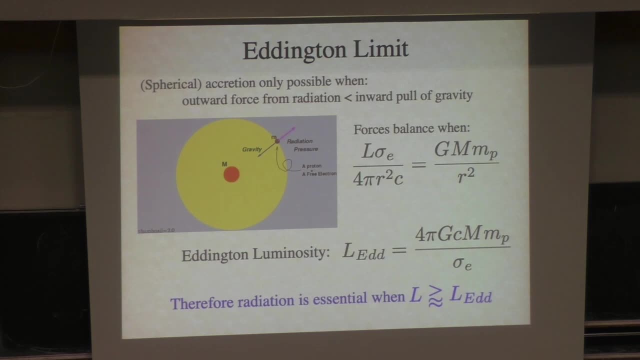 at least in the high accretion rates, where it's really an MHD model and you don't have to do collisionless plasma physics. So that's the first thing you need to include. Of course, the other thing is radiation, And the reason why is because of this so-called MHD. 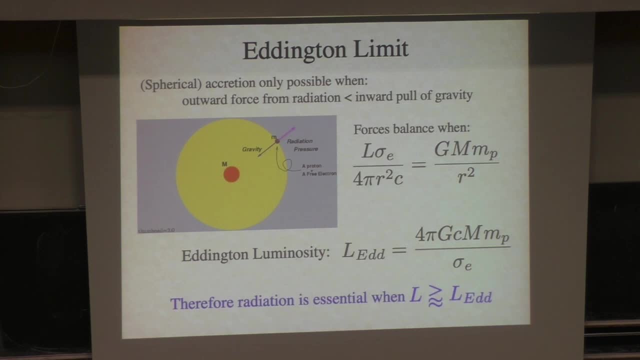 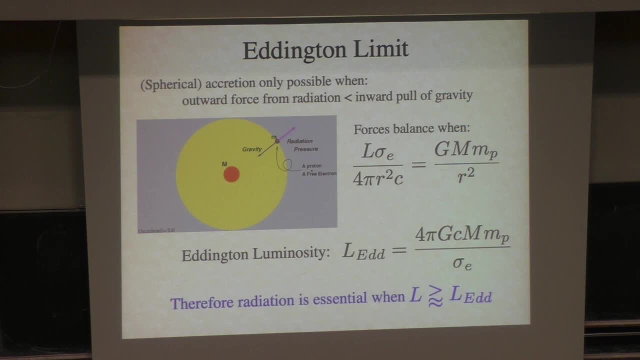 accretion flow. it's the limit where the radiation force on electrons due to photons scattering off electrons, when that outward push of the radiation field is equal to the inward pull of gravity. So for pure Thomson scattering off of three electrons, then it's straightforward to calculate the. 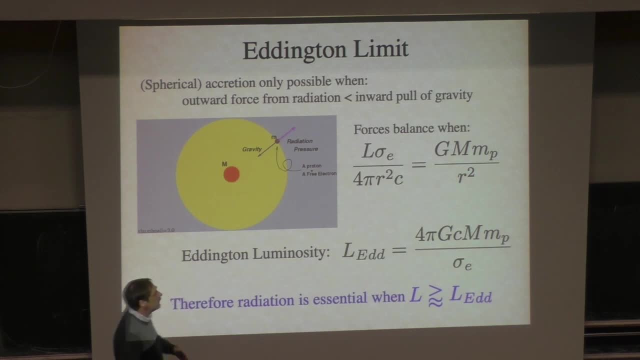 radiation force, luminosity, times, cross-section And of course, the gravitational force. you could just use the Newtonian limit in the far field limit from the black hole And you set those two things equal to each other and you calculate a limit on the luminosity, so called Eddington luminosity, Any. 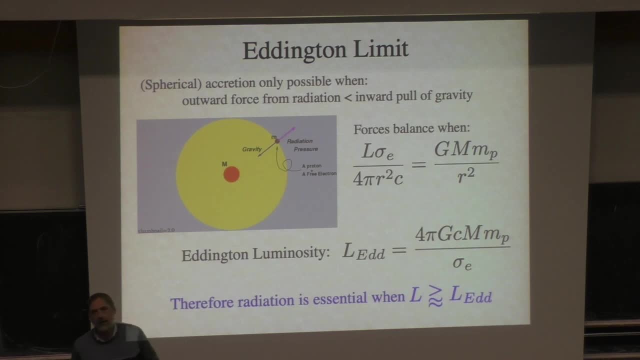 higher luminosity than that, then the radiation force will exceed gravity, and you should be blowing a wind. you should be producing an outflow and not an inflow. Now, of course, this is only for spherically symmetric flow, and so the answer to that question is: is that the radiation force will exceed gravity, So 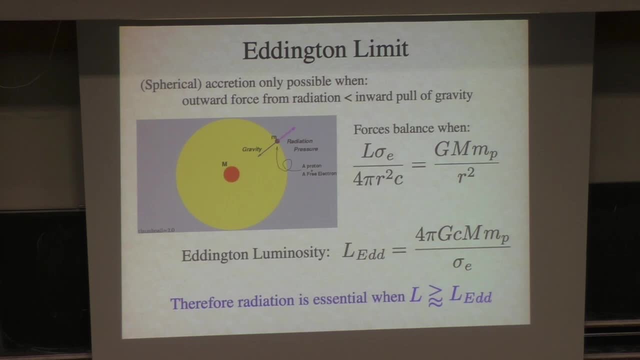 is going to be in, you know, multi dimensions. you might be able to break this, but for spherically symmetric flow, the basic sort of scaling here is: there's a special luminosity, the Eddington luminosity, and when flows are at or near, 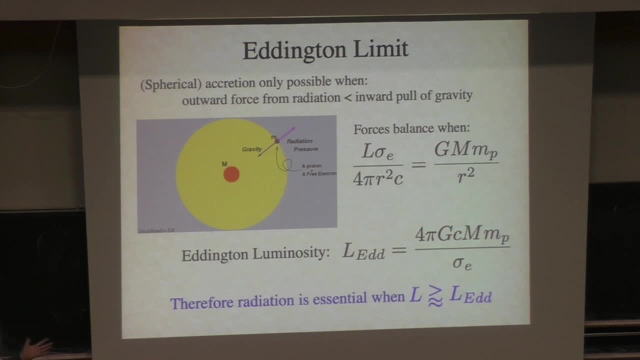 the Eddington luminosity. you clearly need to include the radiation forces or you're not going to get the dynamics correct because the radiation forces are completely dominant or can be dominant, and so we're in that regime. and studying these sources- ultra luminous x-ray sources- are well above this limit, so we 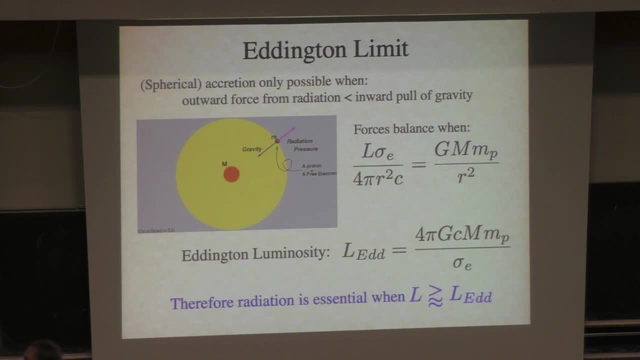 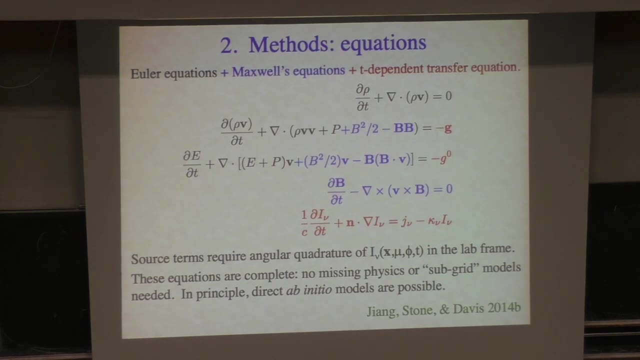 know we need to include these radiation forces. okay, so now we think we know the mathematical model that we need to solve. it's the equations of hydrodynamics, compressible fluid dynamics. so those are the black terms and equations: continuity equation expressing conservation of mass, additional momentum and energy equations expressing conservation of momentum and energy. and 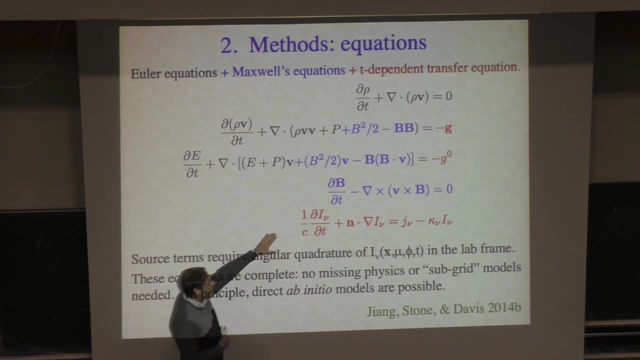 then in addition you need to add in the induction equation to evolve the magnetic field and pointing flux and the energy equation and Lorenz forces and the momentum equation to account for MHD processes. So the black and blue together gives you MHD, ideal MHD and the limit to plasma. 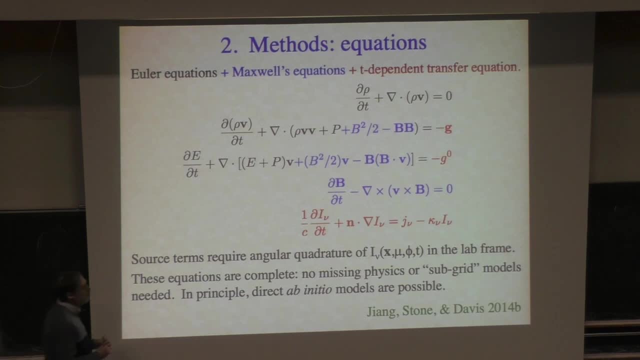 is fully ionized. And then, finally, you need to solve the rate of transfer equation for the specific intensity at each frequency and each angle in the flow, everywhere, including the absorption and emission processes- absorption, emission, scattering processes- And then, given this radiation field, you can then calculate the net heating and cooling rate in the energy. 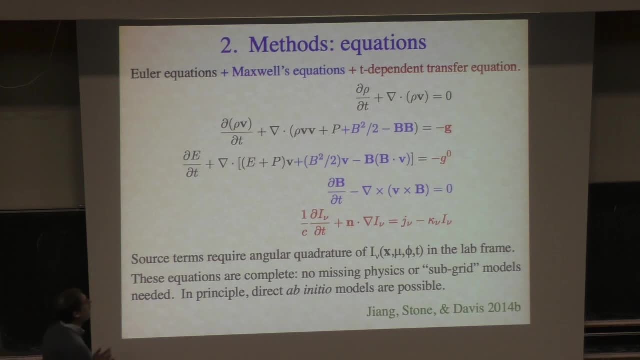 equation due to the interaction of photons and matter and also the net force on the matter, this vector G in the momentum equation, Again, that's the net exchange or momentum between the photons and the matter which comes directly from taking angular quadratures of the radiation field. 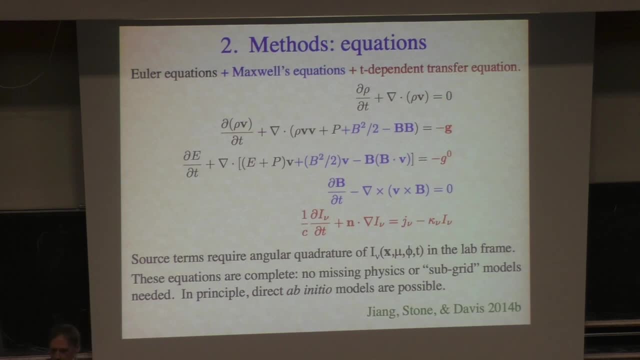 of MHD And the flux in order to calculate those forces directly. So this is the basic mathematical description of a fully ionized plasma, including the effect of radiation fields, and that's what we need to solve: Simple, straightforward, at least the equations. they look simple, Of course. 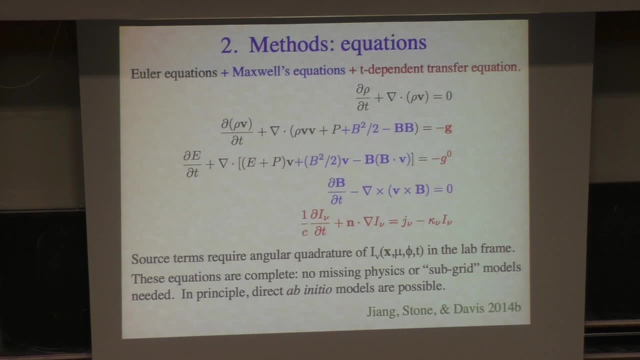 they're a complicated coupled system of hyperbolic PDEs. They're very expensive to solve in multi-dimensions but fortunately, you know, over the last 20 years we've developed numerical algorithms now that have become reliable enough to be able to solve these equations directly. 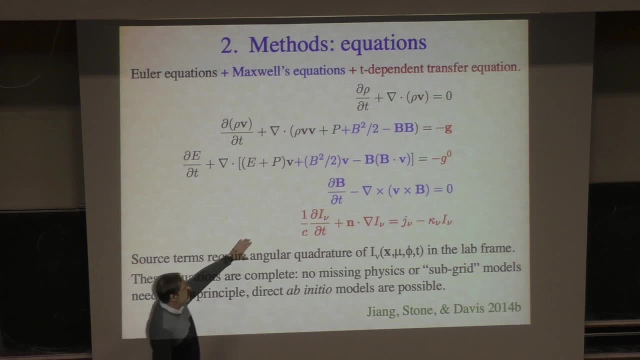 And so you know we're going to be able to solve these equations directly. What's new is the radiation field. This adds a tremendous amount of complexity. It's a highly high dimensional object, and so solving this equation is a bit challenging. I'll say a bit. 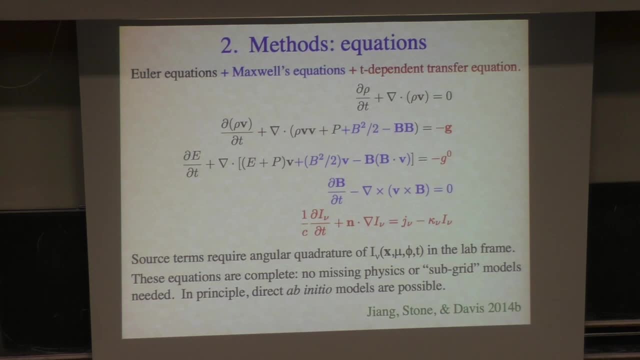 more about that, But I would just make the point that, in fact, if you think this is difficult, I think it's actually very simple, in the sense that we think this is a complete description of the physics. We think this is a complete mathematical model to understand black hole. 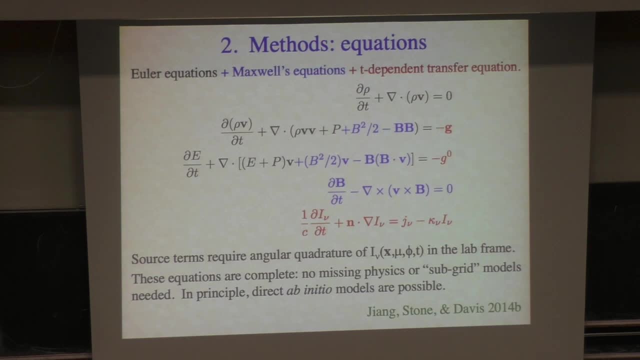 accretion flows. There's no missing sub-grid physics. There's no missing processes that are not represented in this mathematical model. So, for example, in cosmology, you might need to include star formation feedback or AGN feedback at very small scales to study galaxy. 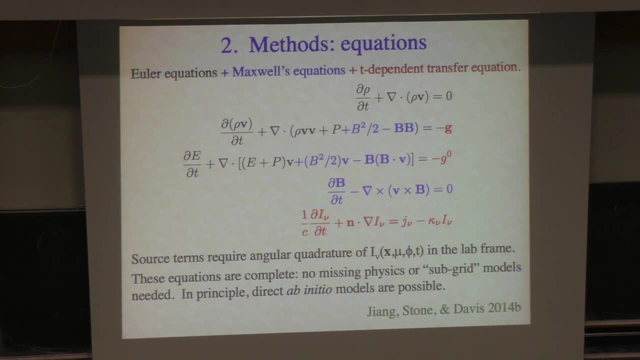 formation evolution. We don't quite know how to do that, so we have sub-grid models. None of that exists in this issue. There are no sub-grid models required, And if we can just solve these equations accurately, we should be able to learn about black hole accretion flows. And if we 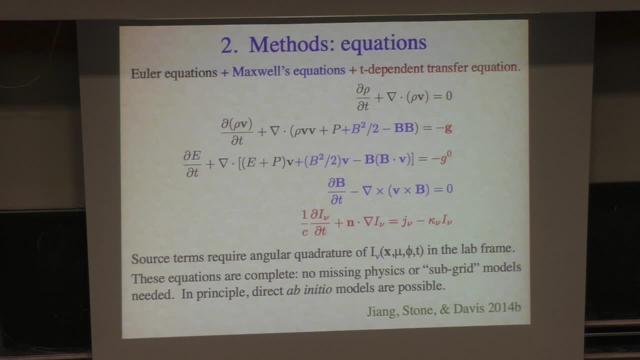 can't model existing flows. that'll tell us something very fundamental about their physics. That'll teach us something very, very important. Yes, Sorry, this n here. that's a direction vector, so that the transport of radiation occurs only when there's a gradient along each direction. 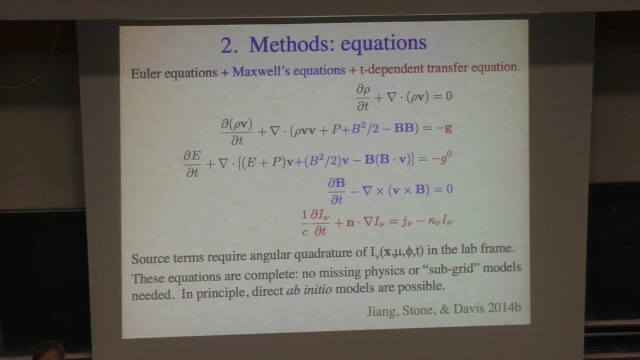 you know, if you like. So it's a directional vector, It's a unit vector on each dimension, Right? So I certainly apologize. I know I'm flashing up equations and if you haven't seen them before, this is going to be complicated. But I want to make two points. One is that they're 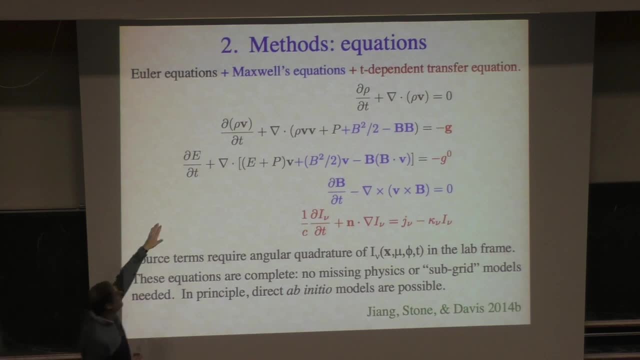 you know. hopefully, by inspection you see they're time derivative plus divergence of something equals a right-hand side, so they're all hyperbolic conservation laws. And then, secondly, they are a complete system that you know. we hope, if we solve these equations, there's nothing more that we need to. 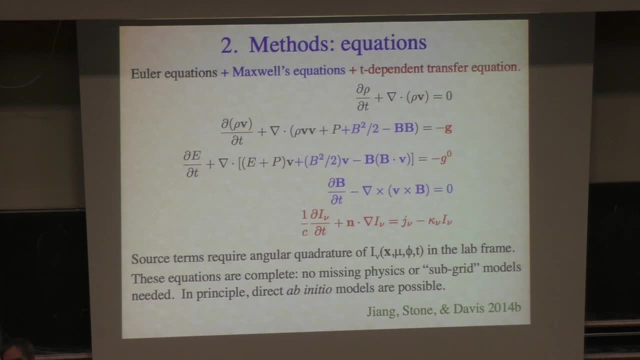 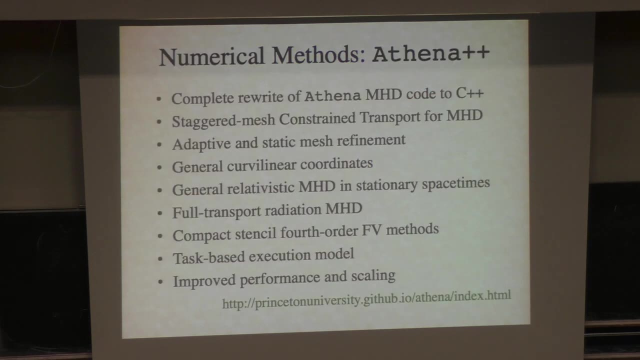 do here, And so I would argue that we're actually in a simpler circumstance than many of our colleagues studying other problems in astrophysics. So that's my optimistic view. So we're using, you know, new methods we've been working on, as we're all. 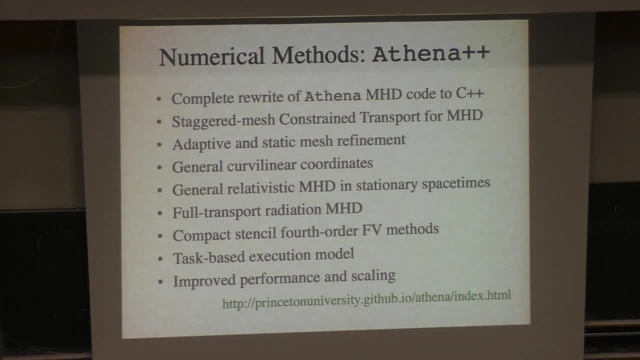 working on this. So you know we're using a new method called Athena++. It's a code that's called Athena ++. I'll mention a code called Athena++. Surprise, surprise, it's a rewrite of a code into C++, This so-called Athena code, which was developed about 15 years ago. So rather than trying, 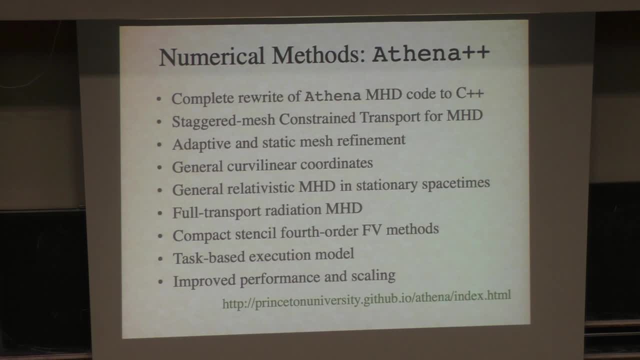 to modify it to include radiation and other techniques that we needed for modern HPC stems. it was much easier just to start from scratch and rewrite the code from scratch than trying to port the code to, say, modern architectures. It uses a so-called staggered mesh constrained transport algorithm for MHD. This is very 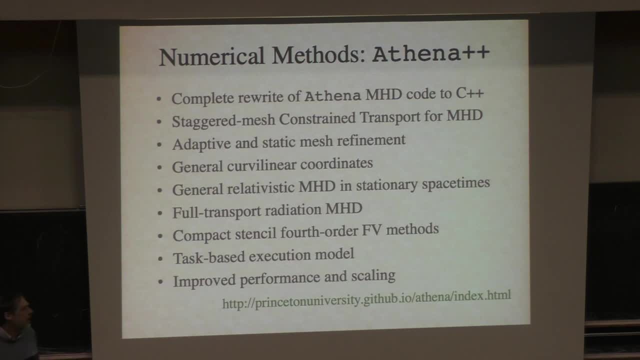 important for keeping the divergence of B0. Another of Maxwell's equations we must satisfy. It's not an evolutionary equation but it's of course fundamental to the physics. So this algorithm guarantees that you keep the B0 to machine precision. We're using adaptive. 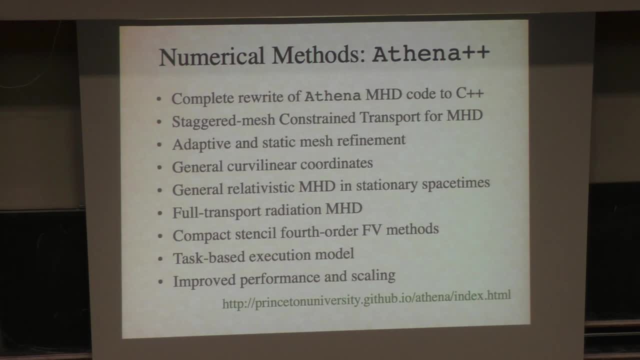 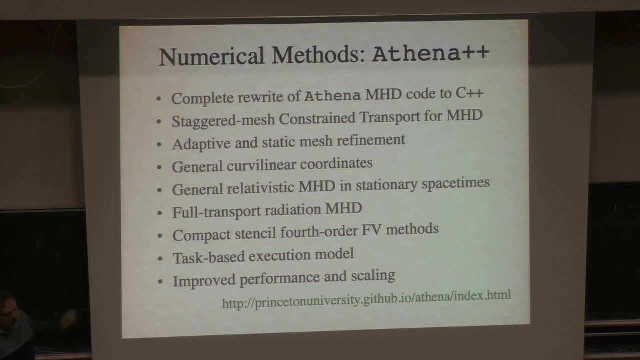 transfer of radiation, the MHD that I'll describe in a little more detail, and various other bells and whistles that help make these calculations possible. And the things that are really important for today's talk are the MHD algorithms, because that's crucial for doing plasma dynamics. The adaptive mesh refinement is crucial for 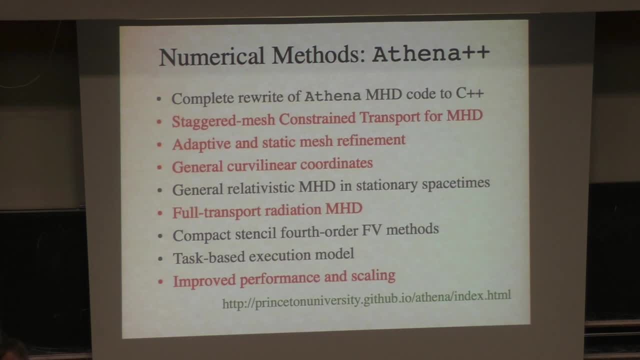 being able to do large dynamic range in space And the curvilinear coordinates is crucial. Finally, the radiation transport is absolutely crucial. So, for example, let me just give you some sort of more examples. You can see some more details in some of these features, So, for example, the mesh that we 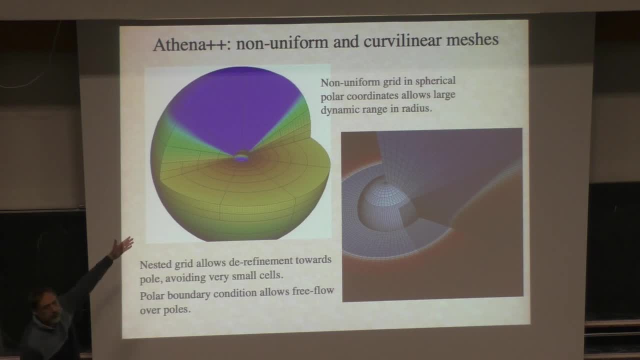 choose is generically a curvilinear, spherical polar mesh, So ideally suited for an accretion geometry flow around a compact object. But in addition we use this mesh refinement to resolve small scales at the midplane, where we know the accretion flow is densest, where 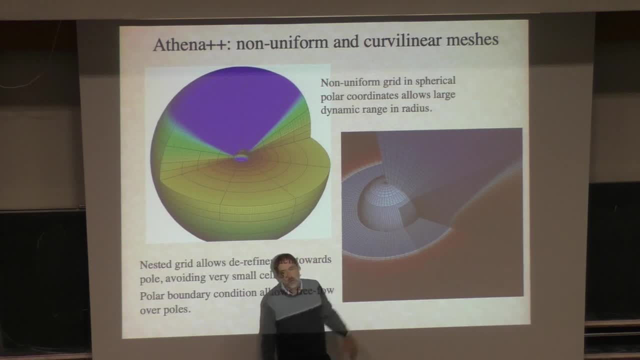 the disc will form, And so we can have very small cells towards the midplane, to be able to resolve turbulence there, and much larger cells towards the pole, where essentially essentially there's no plasma. Plasma is excluded by an angular momentum barrier and never really. 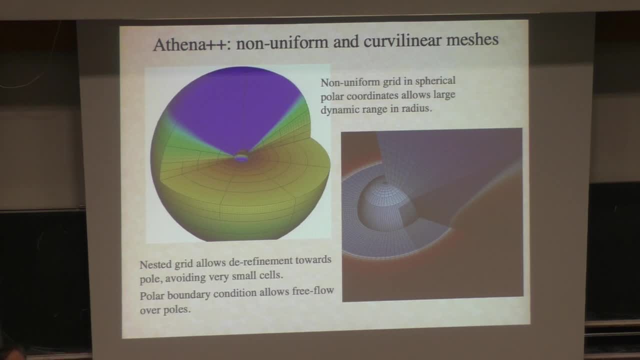 gets to the poles, so you really don't need a very, very fine mesh there. And so, in order to concentrate your computational effort in the regions you need it, you can use these adaptive meshes, And that's a very standard and very powerful technique used in astrophysics. 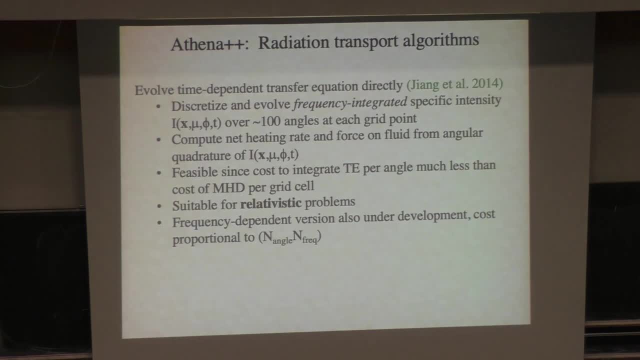 and other kinds of fluid dynamics. For the radiation transport algorithm there's various approximations that many people have adopted over the years And our approach has been to just try to solve the equations ab initio. So in this particular project and for the 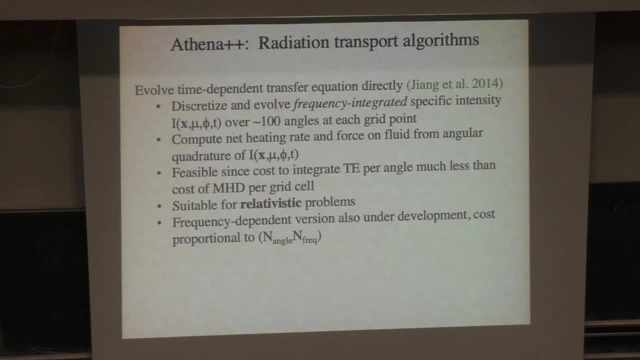 results I'll show today. we solved the time dependent transport equation directly using basically finite volume methods, like the same way we solve all the other PDEs in the problem. It's challenging because the specific intensity this eye object at the top bullet there is. 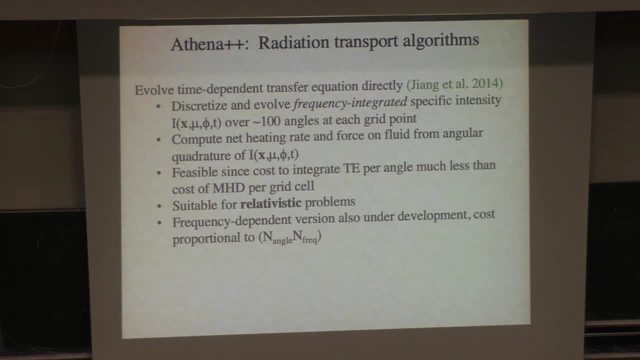 a function not only of position, but also two angles to describe the intensity of radiation in all different directions at each point in space, as well as frequency and time. Now, in principle, well, in practice, what we're doing is integrating over frequency and only solving for the continuum radiation field. So at these, 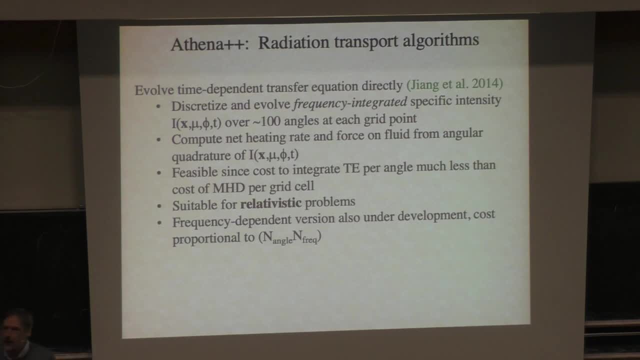 temperatures. the opacities are basically just scattering opacity, gray opacities, and so we can just choose one frequency bin That gets rid of one dimension, but we're still left with a six dimensional PDE that we have to solve, which is two. 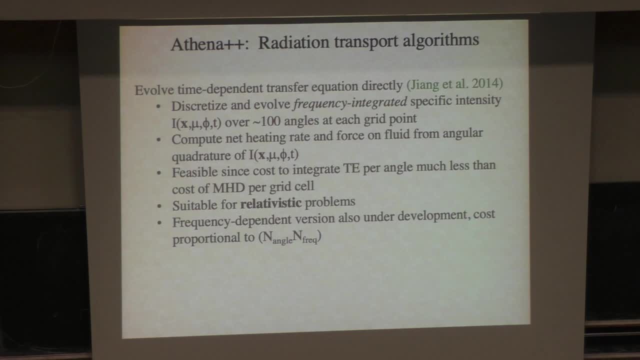 times or two more dimensions than the other equations, if you like, because we have all these angular bins And that means we need, you know, every single spatial grid point on the mesh. we need a hundred angles to represent the spatial or sort of the angular variation of the radiation field, And so that's but. 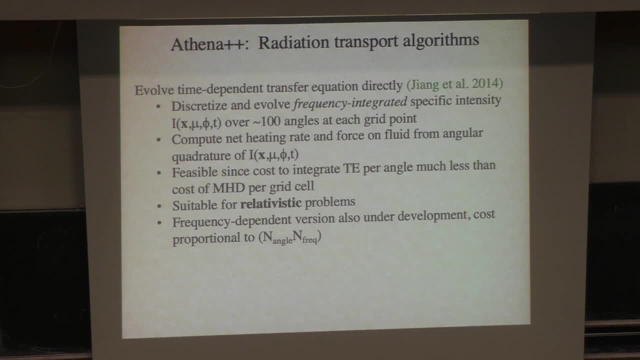 that's a lot of memory, in principle, a lot of calculating A hundred times. sounds like it's a hundred times more expensive to evolve a hundred times more variables per cell. In fact it's not, because the transfer equation is actually very simple compared to the MHD equations, And so the number of actual 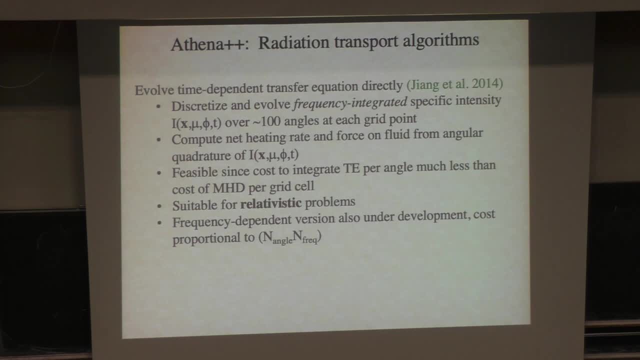 floating point operations you need to update. the transfer equation is probably ten times smaller per variable than it for the MHD equation, So we can get away with what many, many more angles than we do. the other conserved quantities per cell just because solving the transfer equation is a lot cheaper And modern computers now. 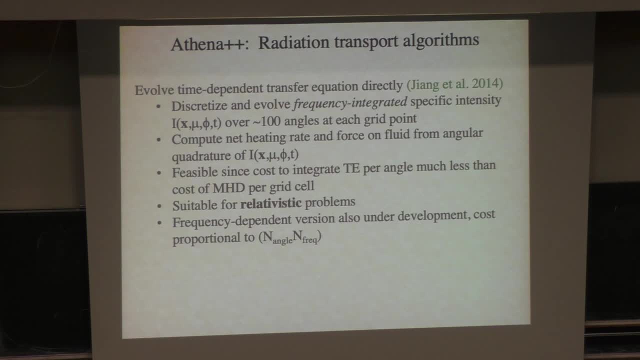 are really very, very impressive, I'm sure you all know, and so it's really quite cost feasible just to simply solve the transfer equation ab initio directly and not make any approximation about how you solve the equations. But we're solving the time-dependent. 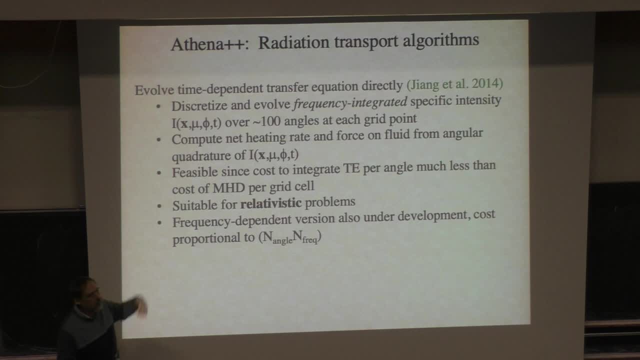 transport equation, which means we're limited by the light crossing time. So really only works well for relativistic problems where the flow speed is comparable to, or at least closer to the speed of light And there's a frequency dependent version that we're working on. The cost, the total cost of the algorithm. 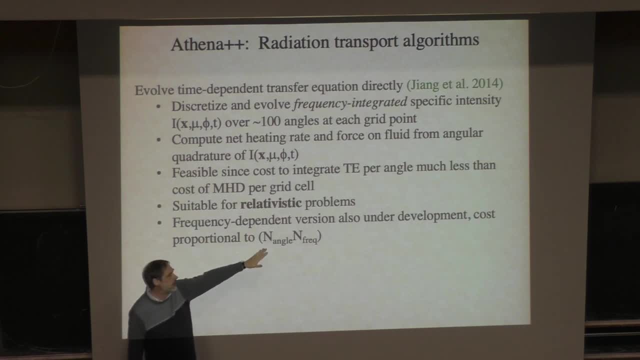 is just simply the number of angular bins times the number of frequency bins. right now we're using one, but we can always, you know, adjust those two numbers any way we want. So we could do some frequency dependent transport- an and now the other. so we can always adjust those two numbers any way we want. So we could do some frequency depending transport. 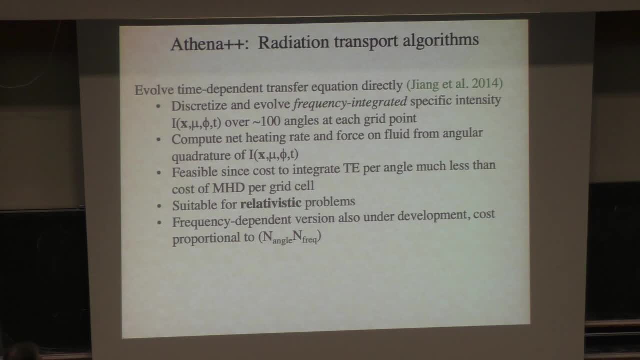 the cost of lower angular resolution. if we, if we chose, and as computers get faster and bigger, inevitably we're going to be able to use much, much larger values here. Yes, How does that also scale with the number of resolution elements? Like it's not linear in number of gas cells, right? 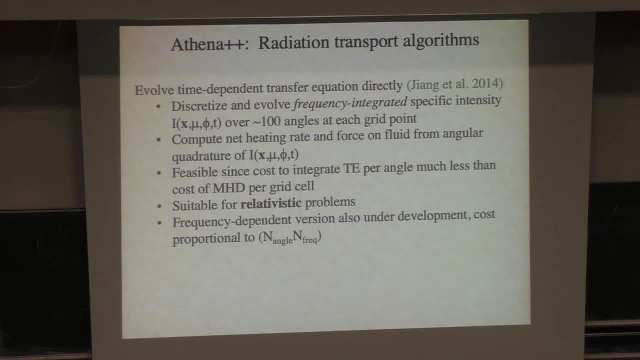 It actually is, because these are all explicit, I mean. so the total cost of the algorithm is the number of cells you know, times these, these factors here. yes, Right, so, but that's, I mean, it's actually very good, it's an order n method. 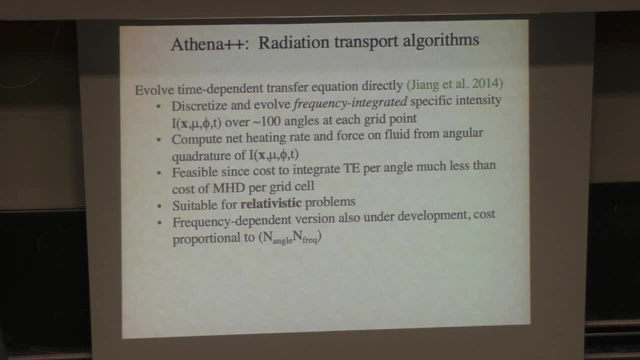 which is probably best you can do so. so not so bad, Yeah, Okay. so so why do we go to such expense? This brute force kind of approach seems crazy, but in fact, for our applications, we know for a fact that it could be very important. 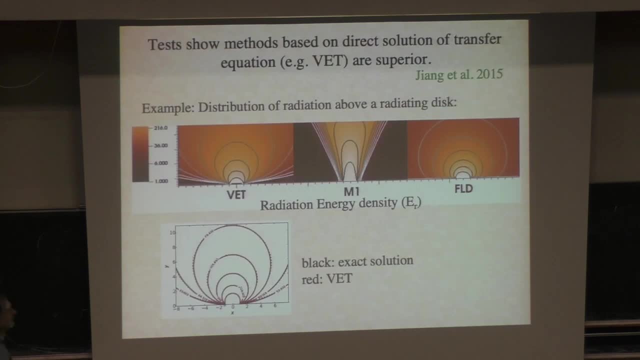 so, for example, we've tried testing more approximate methods, so so-called flex-limited diffusion, where basically you just solve a diffusion equation everywhere rather than solving the transfer equation, and you modify the coefficient of diffusion to try to account for optically thin regions and optically thick regions. 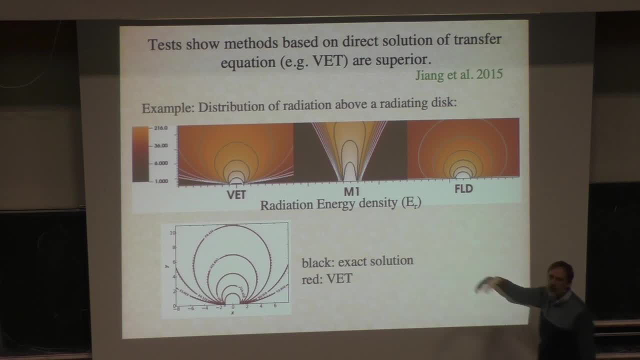 or the so-called M1 method, which does one level of of complexity higher than that. I won't get into the details, this is more for the expert. but if we just do a simple test problem where we have a flat plate of some fixed temperature distribution irradiating free space above it, 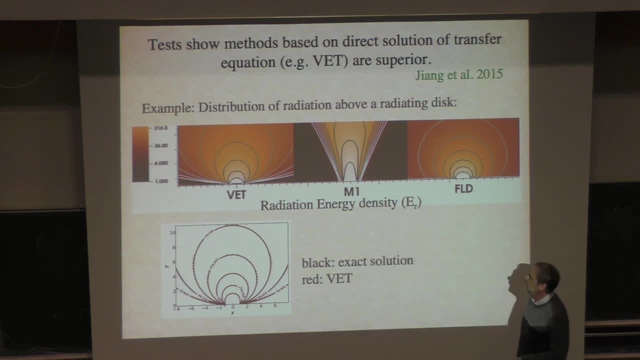 so it's just emitting photons into free space above it. and you ask: what is the radiation field look like in this region, above this flat plate? this is a relevant problem for us because this is our accretion disk and in the middle is a black hole and we're trying to calculate the radiation. 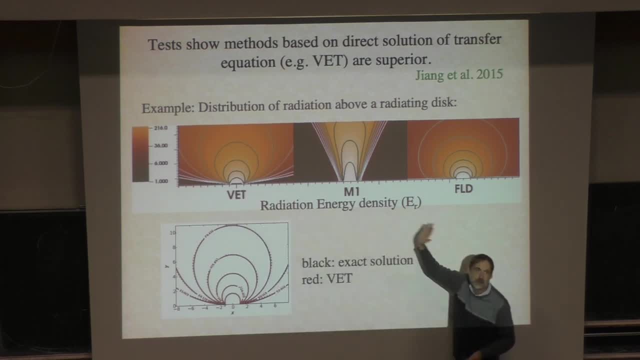 forces above the accretion disks. so we want to know what the radiation field above the disk is. well, you can see that these three methods, so VET is very much like what we're doing now. it's a direct solution to the transfer equation. you can see that VET, M1 and FLD give you very different answers for this problem. 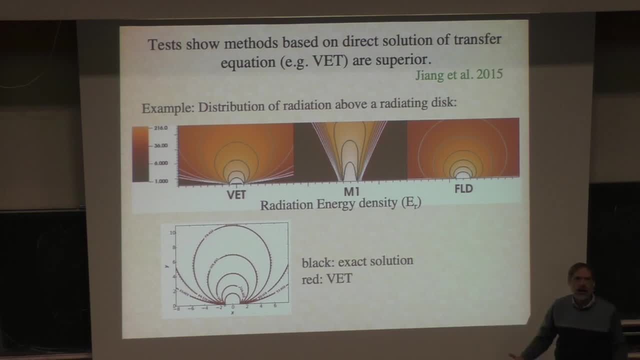 and, moreover, you can compute the solution analytically, you can just calculate, you can just integrate the transfer equation along every line of sight, and that's this comparison here. so the, the solid lines are the contours of the radiation energy density computed analytically in the dashed lines of the VET solution. 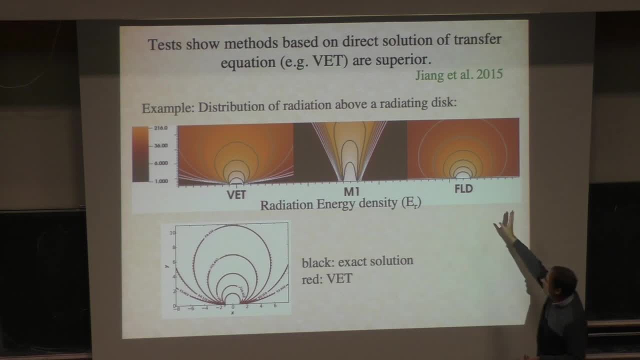 so it's the VET solution that's correct, and the other ones. M1 is significantly overestimating the radiation forces in the vertical direction and that could be problematic for the flows that we're looking at. and FLD is just two diffusers. it's filling in the corners, although, to be honest, it does better than M1 in this. 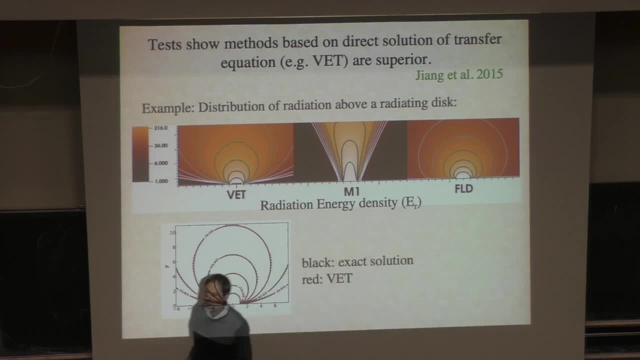 particular application, if you, depending on how you, what metric you have. so my point is that there's true differences between these methods, and figuring out what works and what's important is really very important here, and so because we're not smart enough to know whether or not M1 and FLD is good enough, 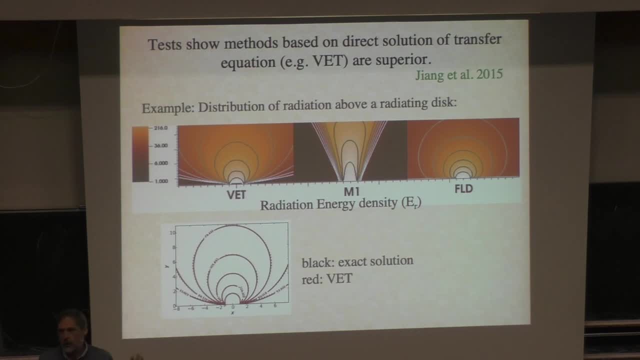 we're just going to do the safe thing, which is solve the ab initio equation, or solve the equation of ab initio and not have to worry about whether approximations are working or not. how else do we know these are methods are working well. we can couple the radiation to the fluid dynamics. unfortunately, there's very 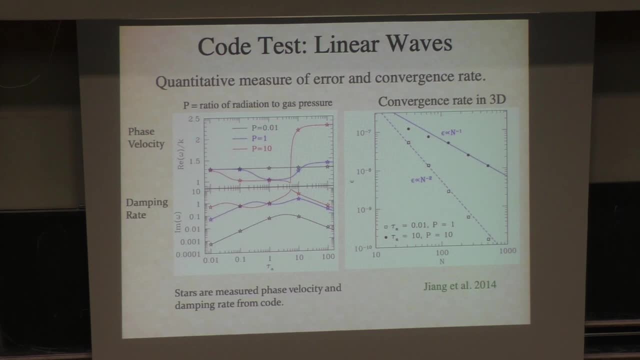 few analytic solutions for the full equations of radiation hydrodynamics. one set of solutions are given by small amplitude, linear perturbation, so linear wave. the dispersion relation for linear waves and radiation hydro that's could be computed analytically. so such waves have a phase: velocity, propagation speed. 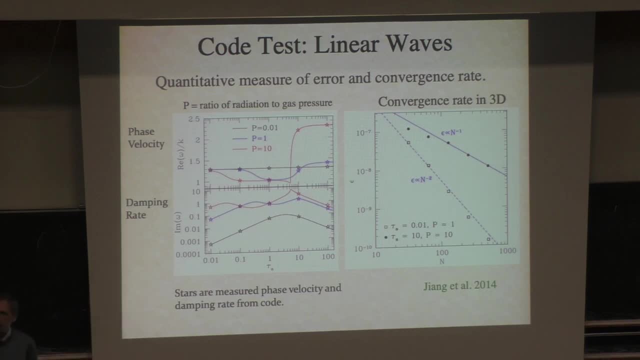 and also a damping rate. so they, these ways, damp because of either diffusion of radiation out of the, out of the wavelength, or because of cooling, and so you can solve that analytically. those are the, the lines of the, the lines of each of these plots, or this is the optical depth per wave length varying. 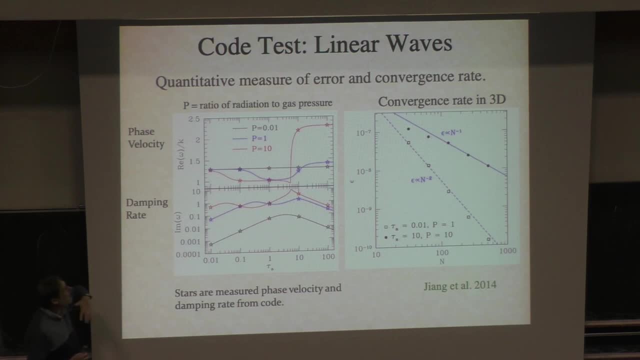 over four orders of magnitude and this is the resulting in real and imaginary parts of the frequency. so the damping rate and dispersion are phase velocity and the different colors correspond to the ratio of radiation to gas pressure. so from very, very weak radiation to a very, very strong radiation, radiation dominates. 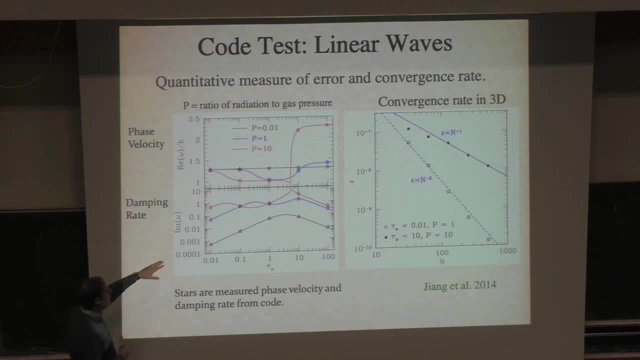 that's the red curve, And then the stars are the numerically measured values. So we set up an exact eigenvalue for this wave on a periodic domain. We propagate it around the box ten times. We then measure its phase, velocity and damping rate, and then 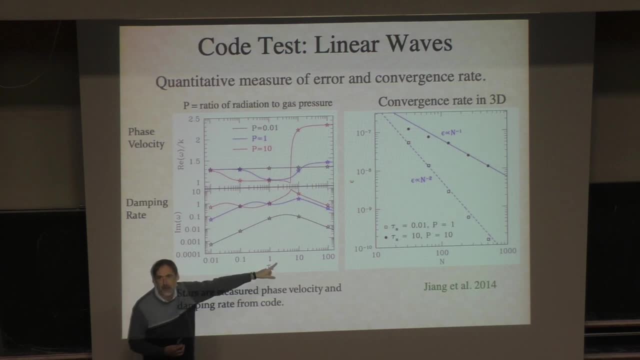 we have one point on this curve. We do that for many different optical depths per wavelength and many different ratios of radiation to gas pressure, And you can see that we reproduce the dispersion relations extremely well. So our methods are indeed working in the linear regime and we can even measure quantitatively. 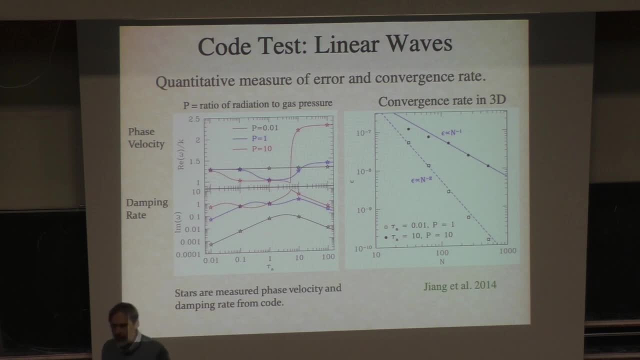 what the errors are and show that our methods are convergent, At least at first order. and since it's an operator split method, that makes perfect sense. So we not only know we have accurate, but you can even measure the convergence rates. Those are linear solutions. What about nonlinear solutions? That gets to. 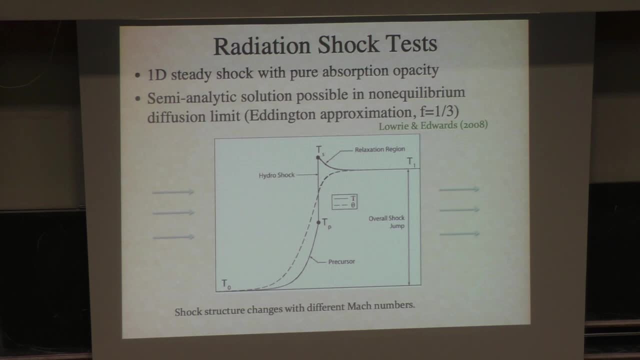 be very difficult now and the only solutions I'm really aware of are for radiation dominated shocks. This is the case where you have a plasma moving in from the atmosphere- freshman to sophomore grade- And you have some the upstream direction supersonically. you're probably used to a normal hydrodynamic shock. 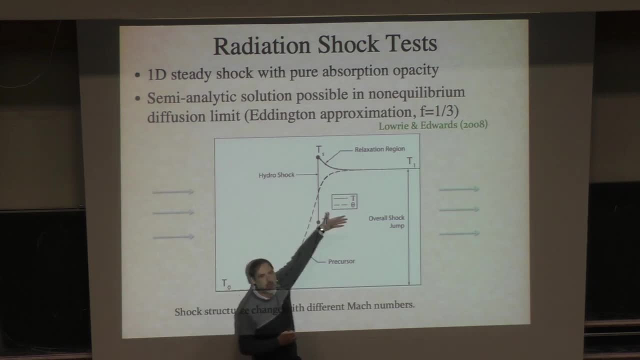 where it goes through a discontinuous jump and then has a constant post-shock state. So the shock solution is just a true discontinuity and you have an upstream and a downstream set of quantities that are related through the so-called Rankine-Huguenot jump conditions. 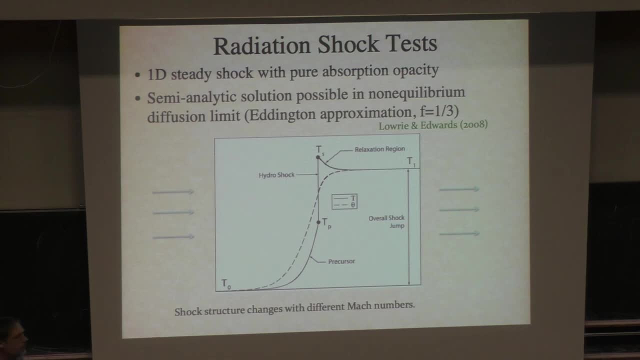 But when you have radiation then you greatly increase the complexity of shocks because photons can propagate upstream of the discontinuity. They can preheat the gas. that changes the temperature and density upstream before it ever hits the shock wave And certainly then it has to cool down in the post-shock region. because if you're emitting 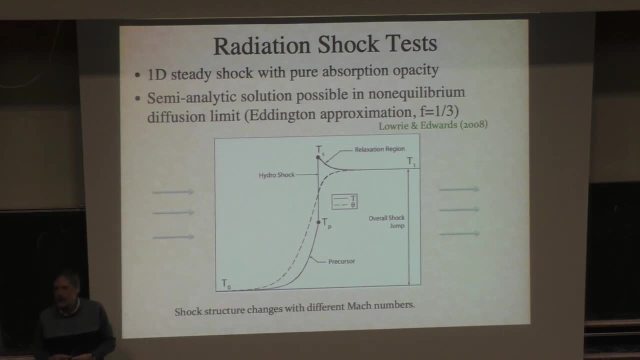 photons that propagate upstream, they must be taking energy away from the post-shock flow, And so in a radiation-dominant shock you get a much more complicated structure. So, for example, this is a plot of the temperature, the radiation temperature, theta and the. 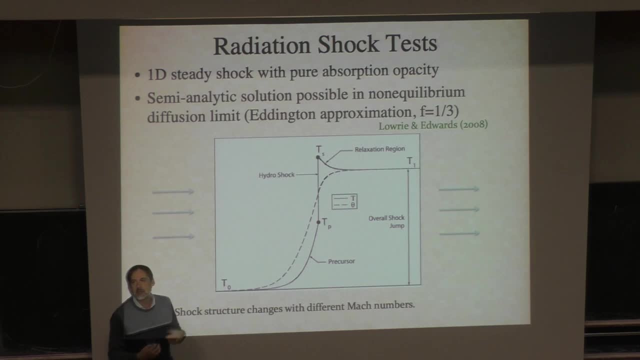 gas temperature, T For a particular molecule, shock number for a radiation-dominated shock, showing you how you have this upstream precursor, this big spike, so-called Zeldovich spike- and then its cooling zone right behind the shock front, where then it settles into the post-shock flow. 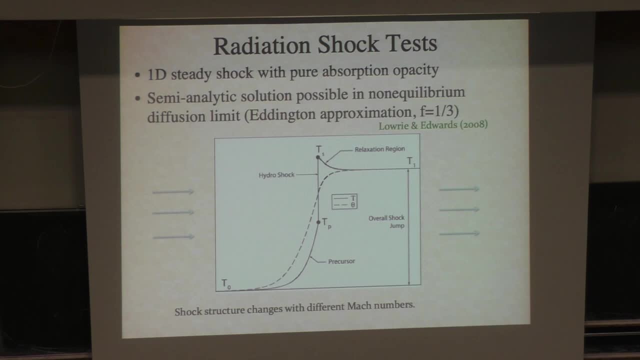 So how do you calculate this structure? Again, you can't do it analytically, but you can solve ordinary differential equations to compute this structure. That's a much easier problem than solving partial differential equations. So we trust the solutions that come from the ODE solvers. 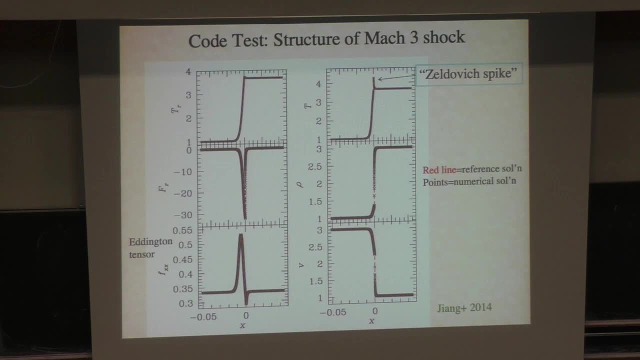 We then compare those directly. They come from our code. We then set this problem. We inject plasma supersonically, We study the shock front, We evolve it for many, many, many shock crossing times until it settles into a steady state. 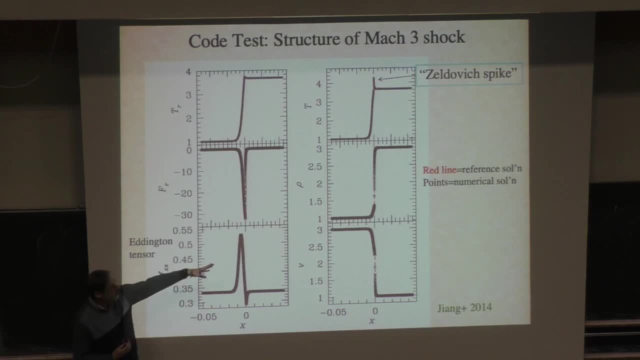 And then the crosses are the solution from our code versus the dashed red line, which is the semi-analytic solution from solving the ordinary differential equations. And once again we have excellent correspondence between the code solution and the analytic solution, including the Zeldovich spike very, very, very, very thin. 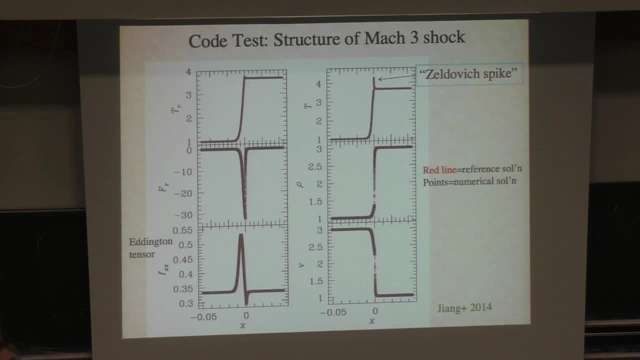 Very thin layer of cooling right behind the shock wave. So we think that we're getting these solutions correct between these linear and nonlinear tests, but we're always looking for more test problems to be able to confirm that we're working. This is only for strong shocks. 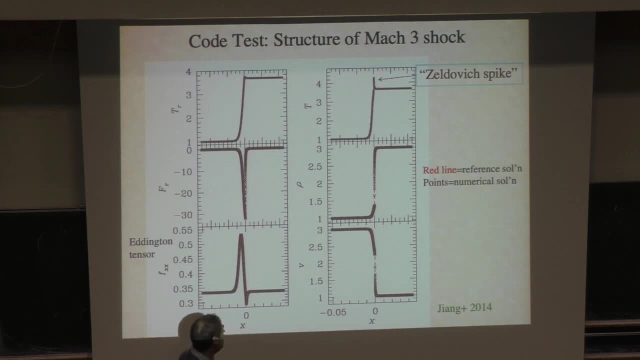 This is only for strong shocks, That's correct. That's correct. So you need to have radiation fields in the post-shock flow, So temperatures where sigma T to the fourth is significant compared to just NKT. So only for strong shocks. 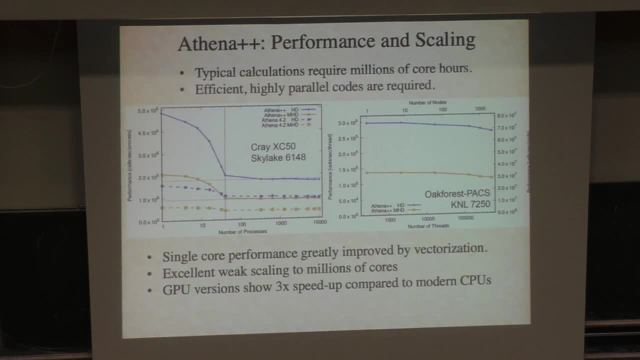 Exactly Yep. So, finally, in order to enable these calculations, you've got to run them on big computers, because it's going to be expensive, And so being able to have not only good single core performance, but also very good scaling over many cores is important. 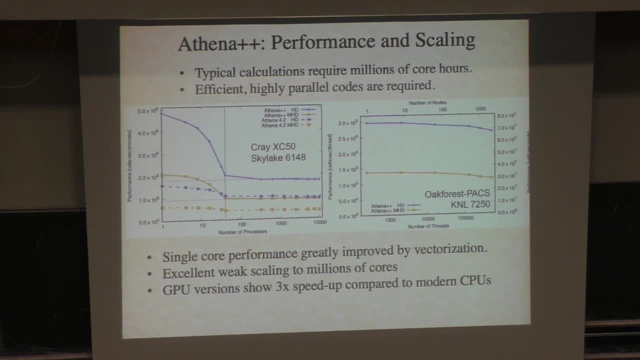 And that was another reason for the rewrite into Athena++ and the C++ is to try to optimize the code on modern architecture. So here's our weak scaling plots. It's the performance per individual CPU and measured in cells, Updated in cells, updated per second, which is a standard measure of performance for grid. 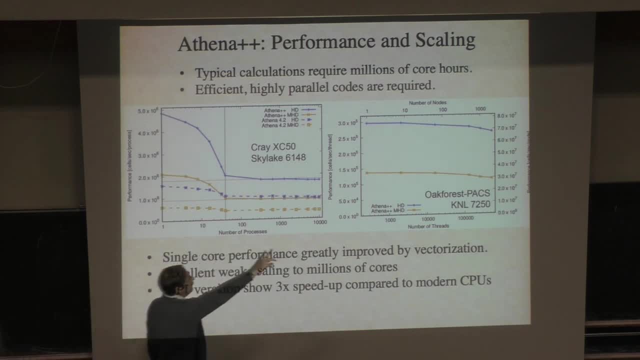 codes versus the number of CPUs that we're using, And you can see that different lines correspond to whether it's hydrodynamics or MHD, or the old version of Athena, which is the yellow lines, and the new version, the blue lines. 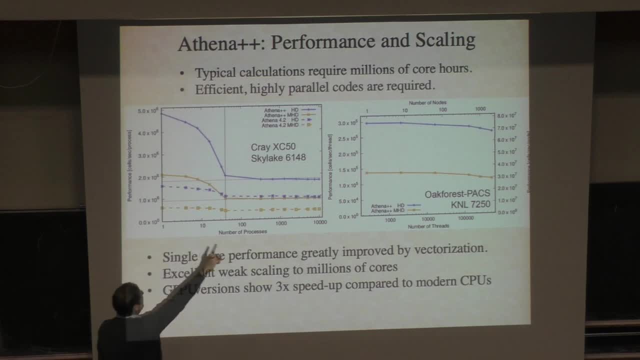 So the first thing you notice is this big drop from one to about 40 cores. That's because these are Intel processors with up to 40 cores per CPU and they all share the same memory bus, And so when you're maxing out the CPU performance, you're getting memory bandwidth limited. 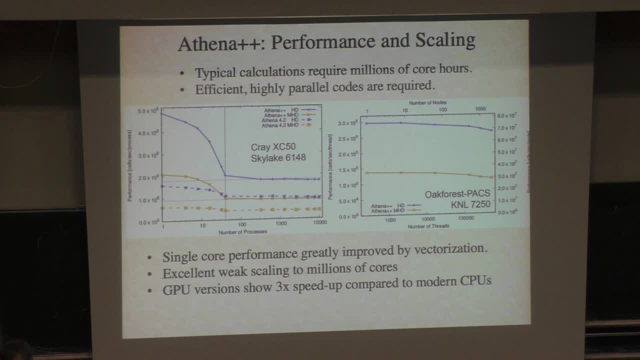 That was half the problem. The other half the problem is a feature that Intel doesn't tell you about, which is that if you actually run vectorizations on these chips, if you actually use the AVX instructions, then you can't have all 40 cores running AVX instructions. 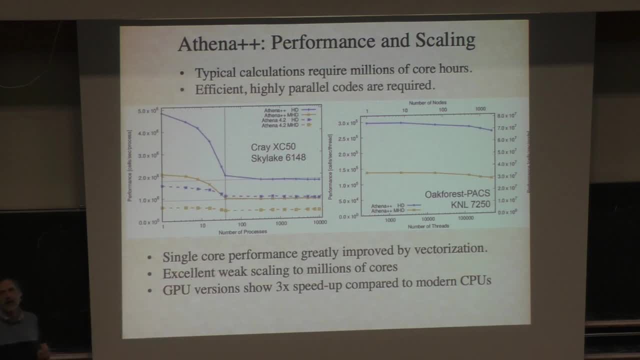 The CPU is unable to handle thermal load, And so it automatically dials down the clock speed in order to give you better performance- so-called smart throttling. Any time a vendor tells you anything is smart, you should be very worried about it. 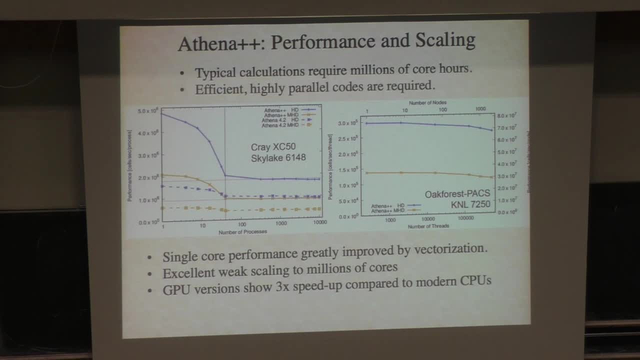 And so it automatically loses 25% of its performance, just because, if you're using good vectorization, the CPU can't actually handle that. So that's just built into the hardware. There's nothing we can do about that. Once you're on the full chip, then after that our weak scaling is very, very good, nearly. 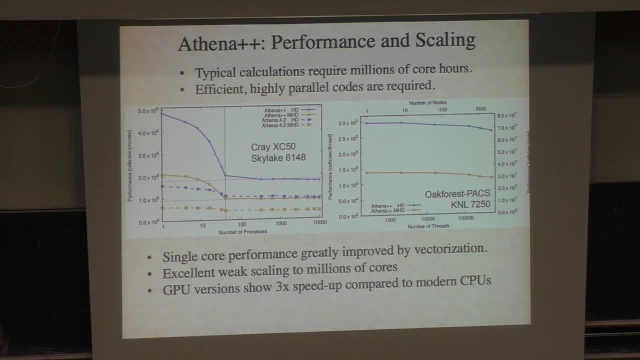 perfect. It's about 95% efficient on up to about 40,000 cores on this particular machine. We also run on this so-called Knight's Landing architecture, Where we do similarly well- up to half a million processes. we're getting about 85% efficiency. 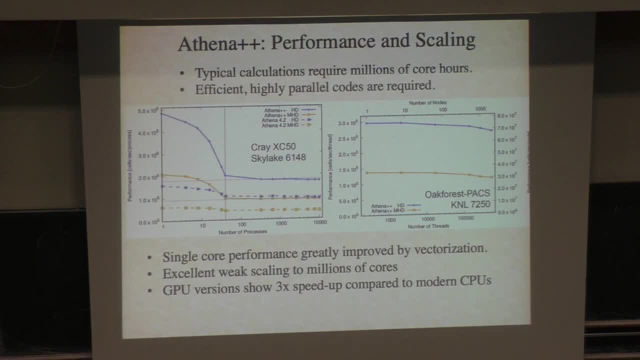 So these methods scale extremely well on modern, highly parallel systems and they really enable you to do very, very large calculations. I should also mention that you work very hard to get the performance better. It's about a factor of two better between Athena and Athena++. 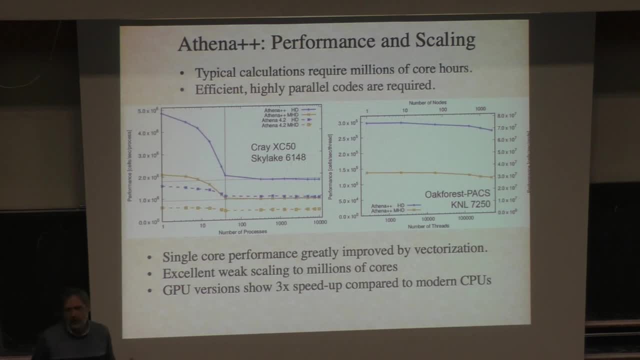 And it's running at about 2 million zone cycles per second per core for every calculation. That's really quite enabling. So on a 10,000 cores, you're doing many trillions of zone updates per second, which means you can do very, very large meshes. 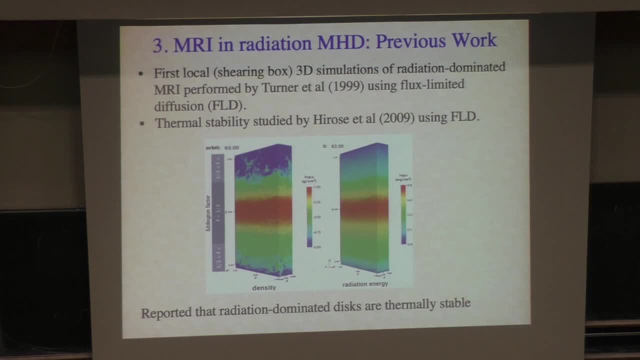 So let me turn to some of the results that we've gotten, And so let me give you a quick summary of what some of the other results have been found in the past. So we're not the first people to look at radiation-dominated flows in this regime. 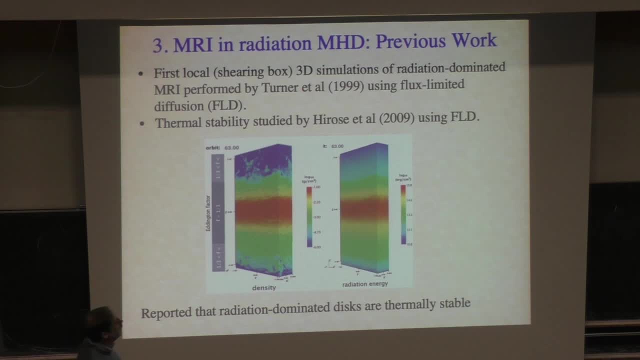 I think the first paper we're aware of was by Turner et al, who used flux-limited fusion and one of those algorithms for radiation hydra that I mentioned, in local shearing boxes, like the movie I showed you earlier, the MRI. 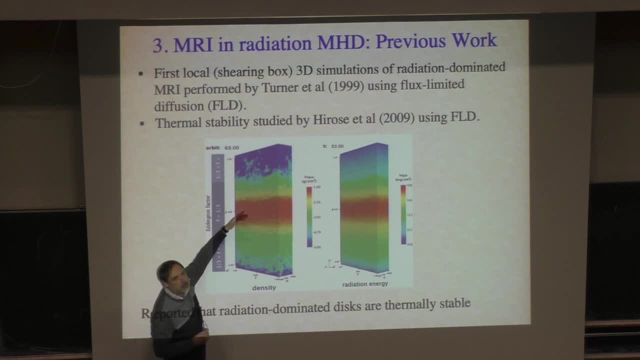 These were 3D stratified boxes looking at turbulent dissipation, balanced by rate of cooling, to look at the steady-state structure of these accretion flows in the local shearing frame. These flows were predicted to be thermally unstable that a radiation-dominated accretion 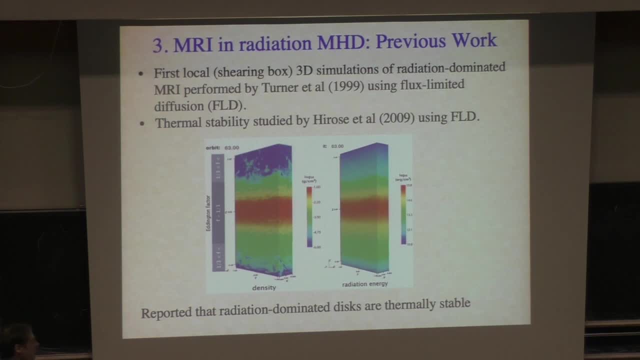 disk back in the 1970s was predicted to be thermally unstable. They found them to be thermally stable in these calculations. It turns out we repeated this work with our- Yeah, With our- full transport method, in fact found that they actually are thermally unstable. 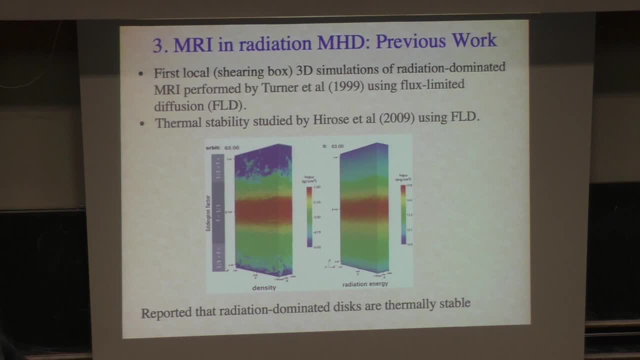 They do show thermal runaway and the differences because of using FLD. this made a difference to this problem, as well as differences in the exact parameters of the calculations that we're doing. So we now know that radiation-dominated thin disks are thermally unstable and do show. 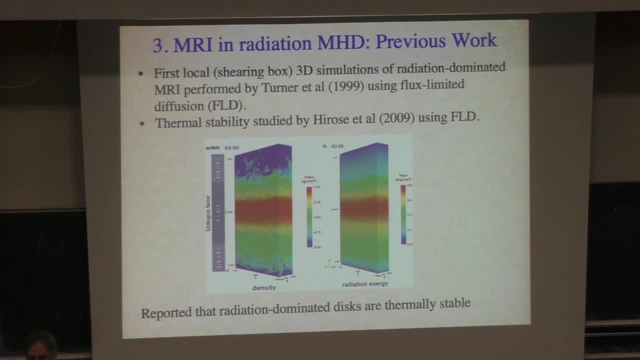 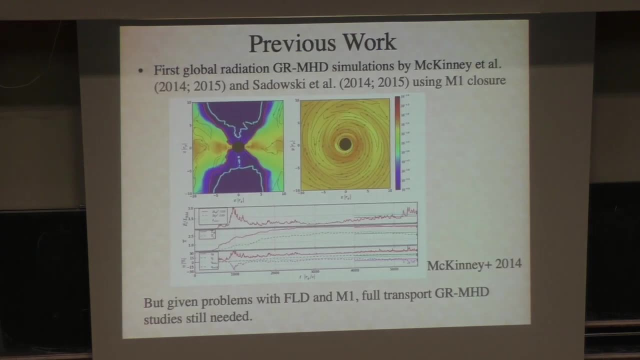 thermal runaways, although the exact details of the instability are very different than what Shakur and Snyayev predicted back in the 70s. All right, Thank you. The most recent global simulations for black hole accretion flows, including radiation. 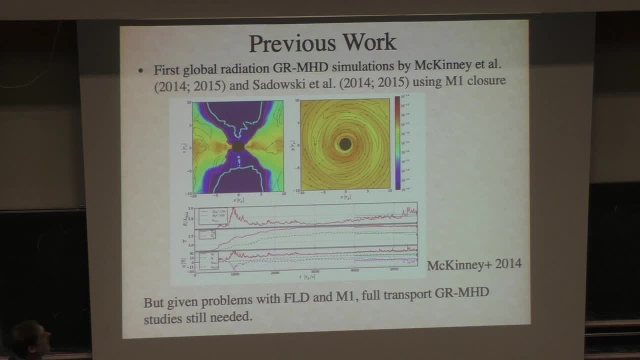 include work done by John McKinney and Oleg Sadowski about five years ago using the so-called M1 closure, And here's an image from one of their calculations showing you the poloidal flow and the equatorial slice, And I'm sure there's no way you can possibly read these axes, probably even in the front. 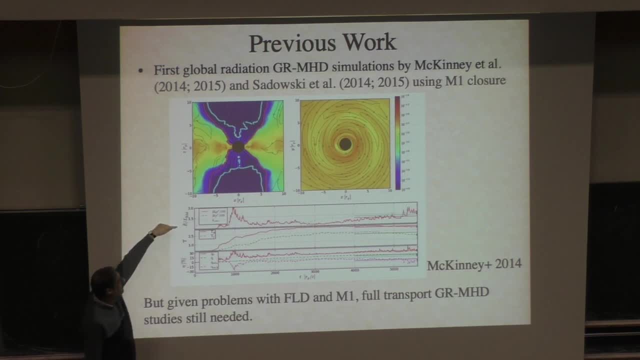 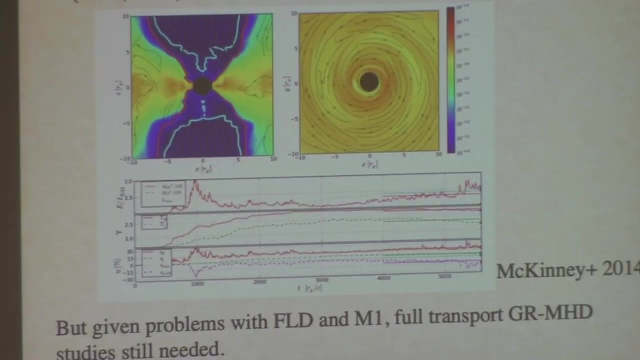 row. But important is the mass accretion rate. Sorry, this is the output energy divided by the Eddington luminosity, so it's in some sense an efficiency. And this blue line here is what they measure from the simulations and they're getting. 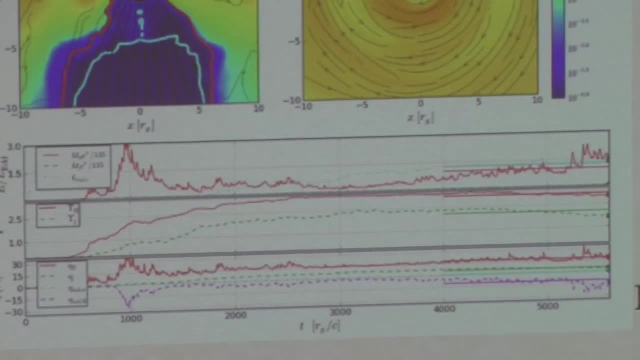 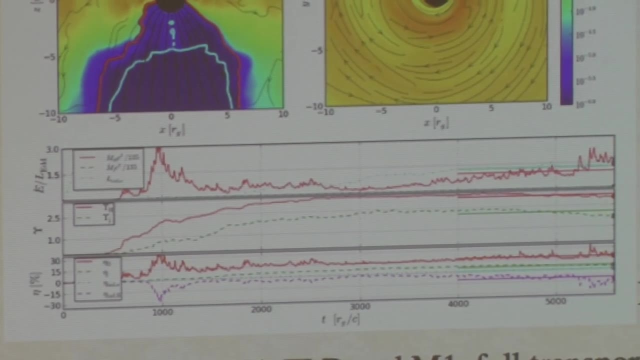 a ratio- a little bit less than one, and a ratio in efficiency that's about a couple of percent. So the amount of energy coming out in photons is about a couple of percent of the energy going into the black hole from the accretion. 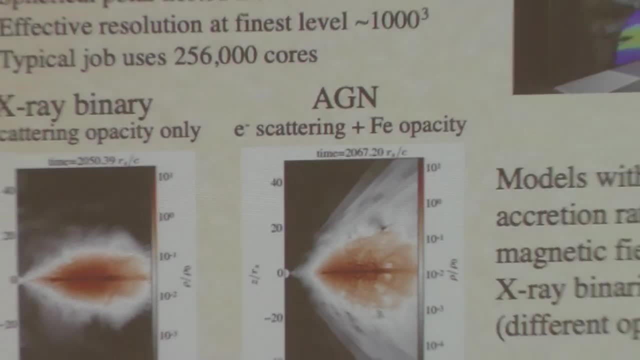 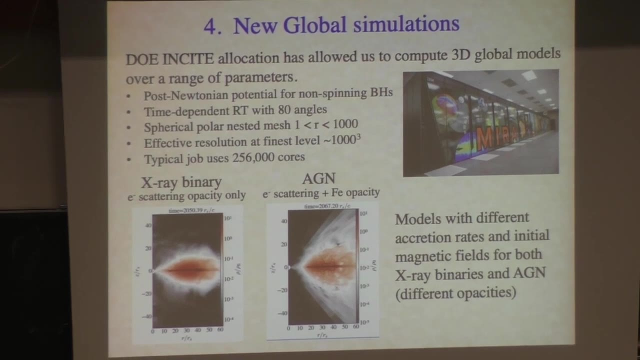 And that's an important number to remember because we're going to try to look at that one ourselves. And so we've done a whole new series of global simulations, following on the work, for example, of McKinney and Sadowski. This was enabled by an allocation of computer time by the Department of Energy, for which 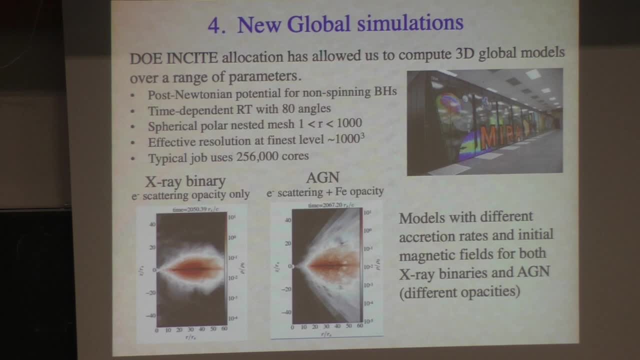 we're very, very grateful. They're typically using 250,000 cores for each one of these calculations. They take 10 to 20 million CPU hours. We have a dynamic range of roughly three orders of magnitude and radius. We have roughly a billion gridlines. 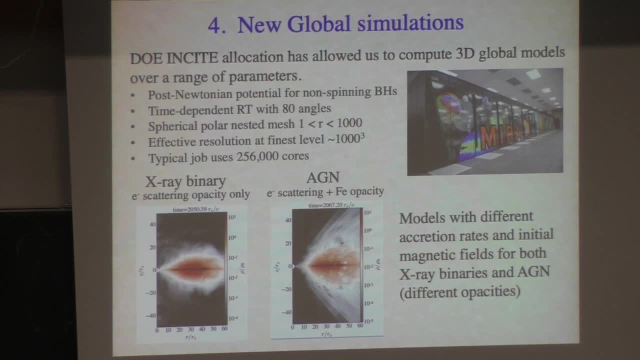 That's a lot. We have billion grid cells with 100 angles in every single cell And we're evolving these for several thousand orbital times in the inner part of the disk to let it settle down to a steady state. And then we're trying to measure the properties of the steady state, accretion flow, including. 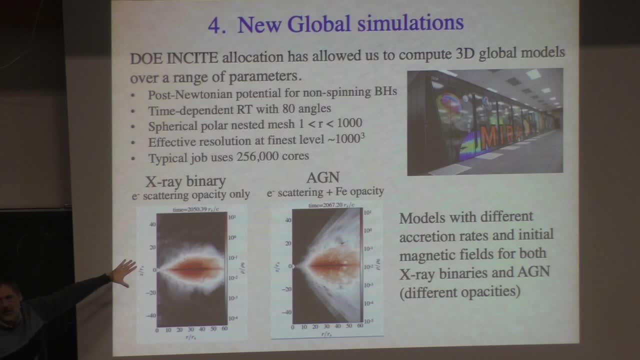 radiation dynamics for two systems- x-ray binaries, which I mentioned earlier, and AGN, And the difference between the two is the sources of opacity. In x-ray binaries, the plasma is so hot, typically 1 to 10 million degrees Kelvin, everything's. 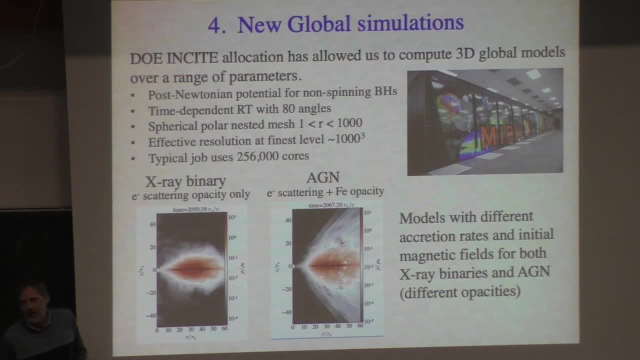 completely ionized and you only need to include electron scattering opacity. But in the supermassive black hole case AGN, the disks are somewhat cooler: only maybe half a million degrees Kelvin or maybe 300,000 degrees Kelvin. In that case there's a few remaining iron ions left around. 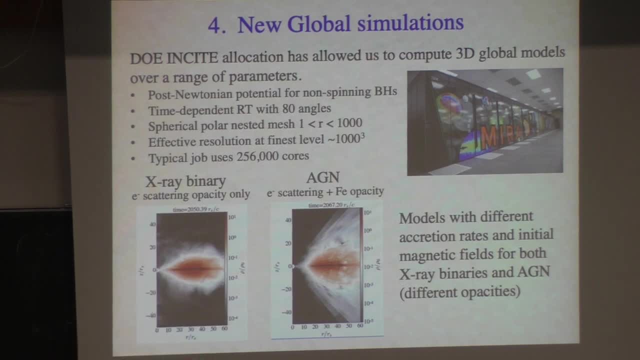 They have so many spectral lines that they contribute significantly to the continuum opacity. This is the so-called iron opacity bump, known to be very important in hot stars, for example, And so we've included that in the models of AGN. So, unfortunately, radiation hydro breaks the dimensionality or the non-dimensionality of 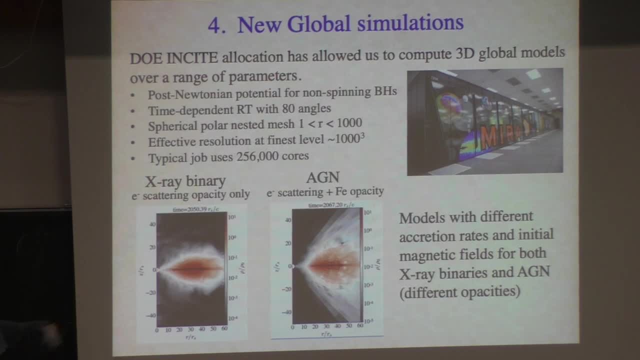 the problem, meaning you can't run one model for any mass black hole. You have to scale the models, compute models individually for each black hole mass, because opacity cannot be scaled dimensionlessly, because the sources of opacity depend on temperature and that's a dimensional quantity. 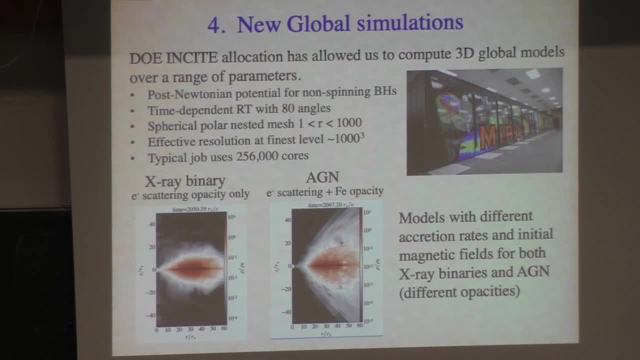 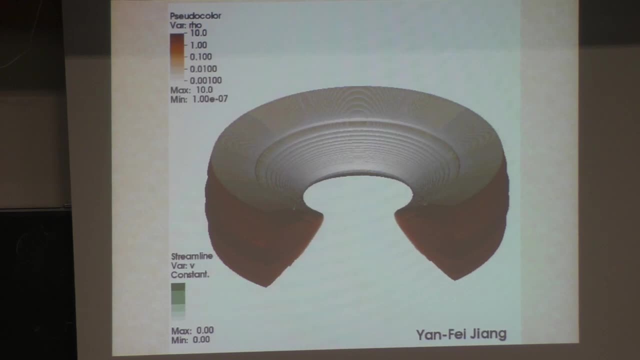 And so just the way it is. it makes things much more complicated. So how do these calculations work? We start with a donut of plasma in rotational equilibrium around the object. There's a weak magnetic field embedded in the donut. This makes it MRI unstable. 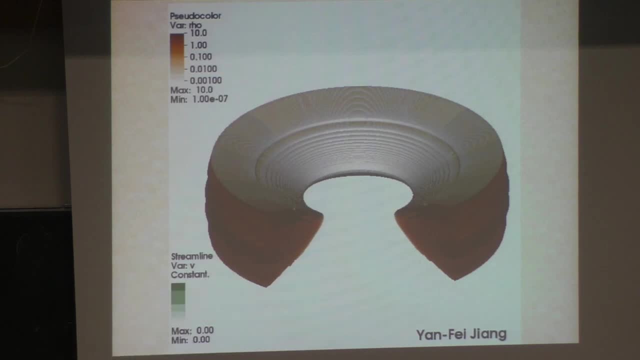 The MRI will grow and produce turbulence and then we follow that turbulence and the accretion that results from itself consistently. You see, quickly the inner regions fill in. You can see the turbulence being generated. It's saturated throughout the domain as the MRI saturates. 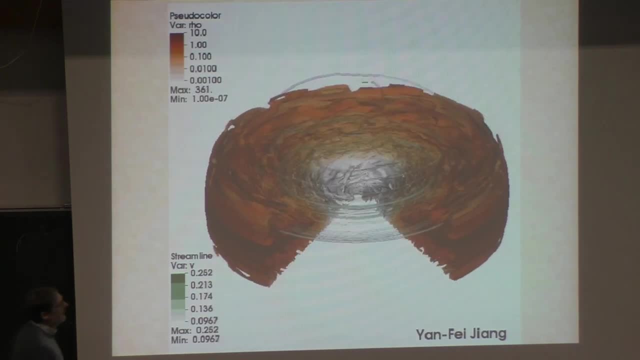 And now we evolve this now for many orbits, at least a couple of orbits at the outer edge, in order to look at the steady state properties of the flow in the inner parts. We have no control over the mass accretion rate That's set self-consistently by the MHD. 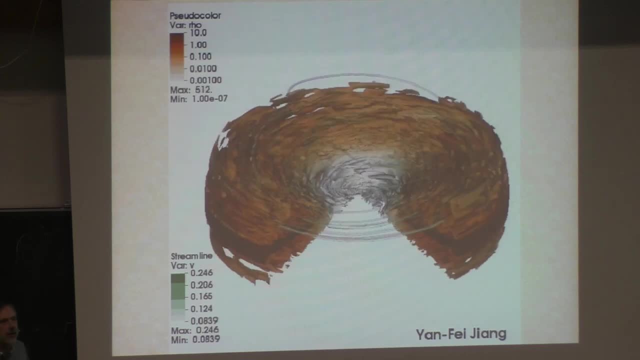 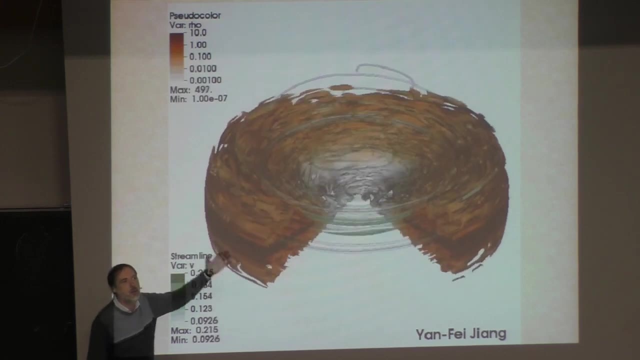 It's not a number that we enter into the code, It just happens. The only thing we can control is the initial surface density of the torus. by changing the total amount of mass in the torus We can affect the total mass accretion rate, but not to an individual number. 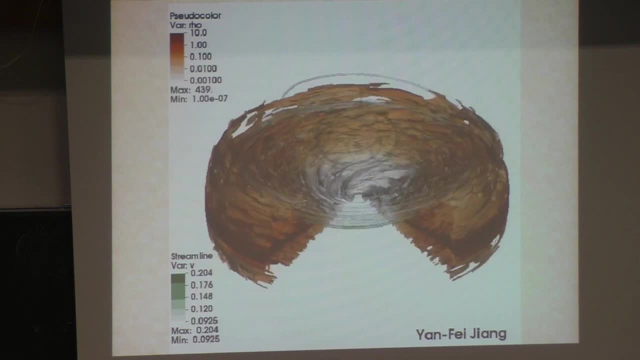 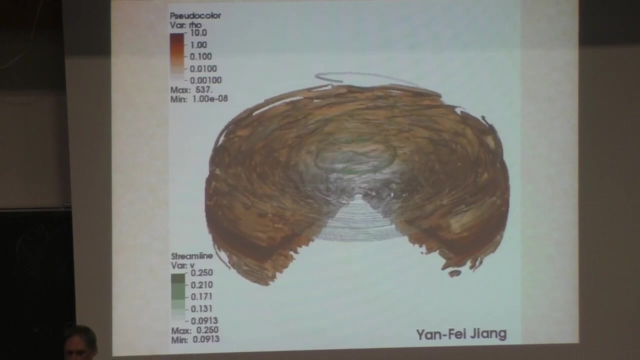 We can only just make it big or make it small by moving a lot of mass or a small amount of mass in the initial torus. The wire lines, you see, are the streamlines in the flow, and so you do see outflows coming from the pole, but it's completely dominated by the rotational motion generally of the 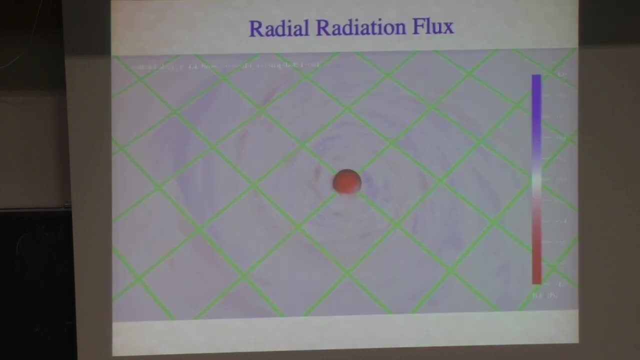 disk. Another way to look at this data is to plot the radial radiation. This is the radial radiation, This is the radiation flux, so the outgoing, or the radial component of the radiation flux, with outgoing labeled as blue and ingoing labeled as red, and this is an equatorial. 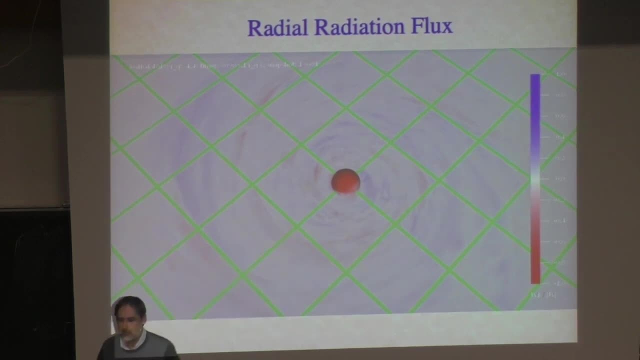 slice and then a hemisphere, and this hemisphere will move slowly out through the domain to show you the structure of the radiation flux and then it will open up like a pie so you can see inside. So you can see how the flow is largely contained to the midplane, that there's a large outward 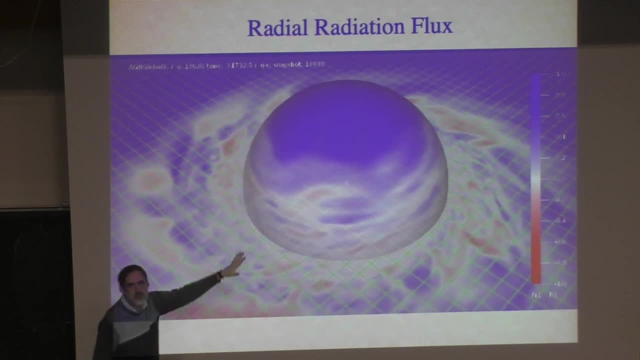 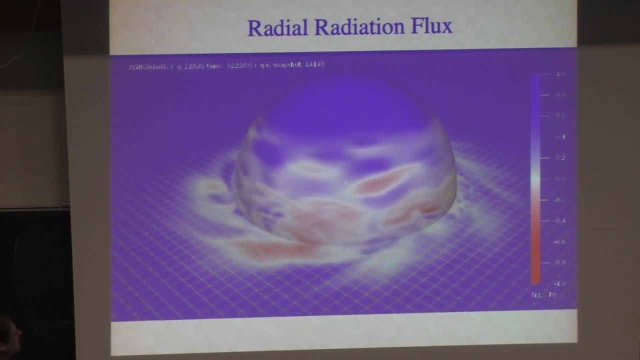 radiation flux towards the pole There's not so much material. Therein lies the solution to the superlinked accretion problem. Most of the radiation comes out the poles where there's not much material. You can see turbulence producing inward and outward fluxes of the radiation field at every. 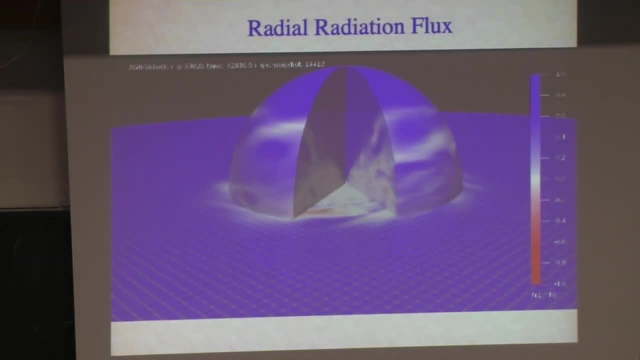 radii. We're now at 300 RG, 300 times the black hole radius. Open it up and now you can see the poloidal structure and the turbulence as this evolves, as this bubbles and boils along, all driven by MRI turbulence. 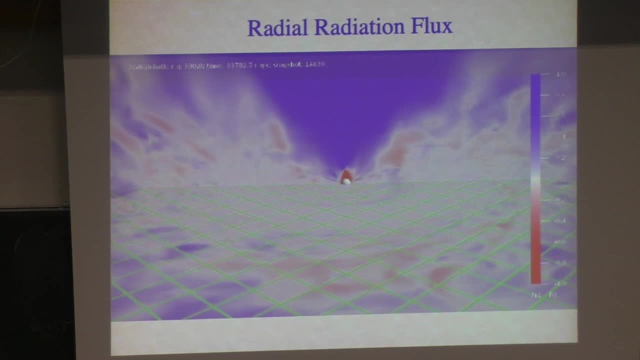 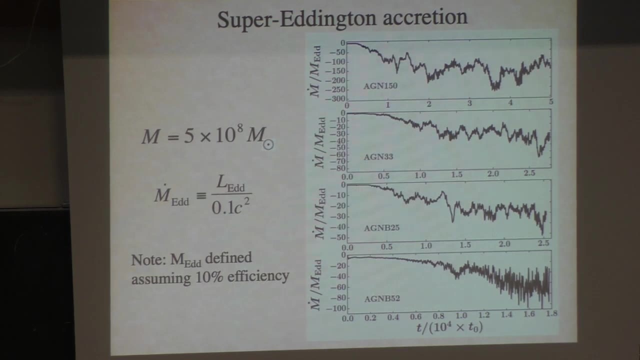 Okay, Thank you. So what are the properties of these flows that emerge from these solutions? So, first of all, we do get super-Eddington accretion If you measure the mass accretion rate divided by the Eddington value, where the Eddington 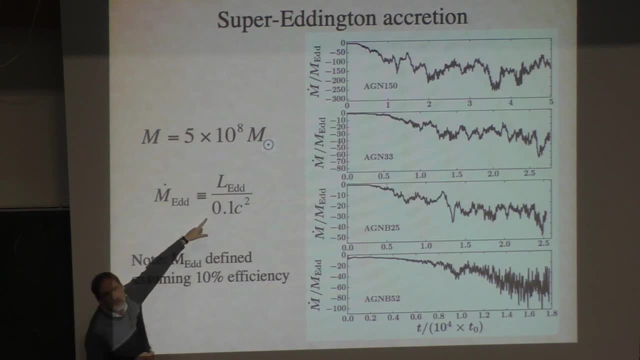 value is defined by an efficiency of 10 percent. it would be the energy released if 10 percent of the energy went into thermal photons. That's defined to be the Eddington ratio and the standard value used for the mass accretion rate. 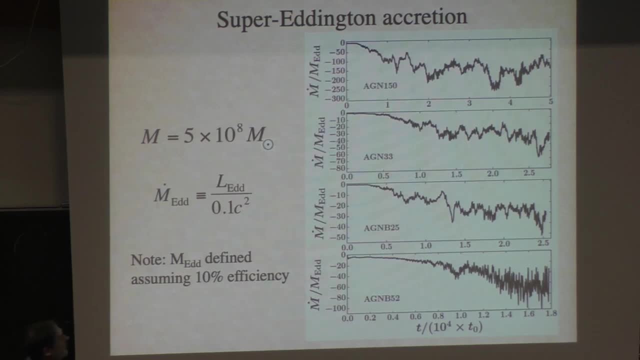 So in this Eddington units we're getting accretion rates. It's that in the top panel in the time average the accretion is 150 times the Eddington rate. So the number at the end of the name is the mass accretion rate in Eddington units. 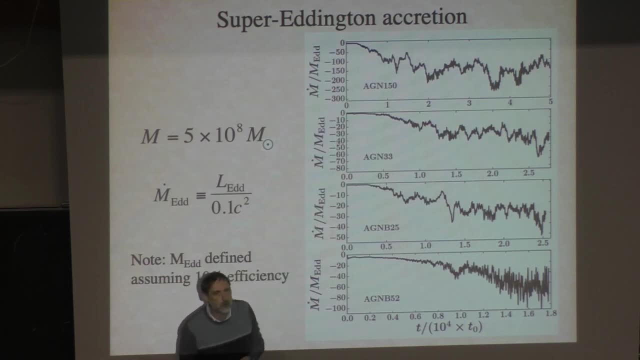 So everything from 150 at the top to 33 and so on, The differences between the models are the initial magnetic field geometry, or the initial density and the surface density in the flow. So first of all, you know, after a transient period each model tends to settle into a 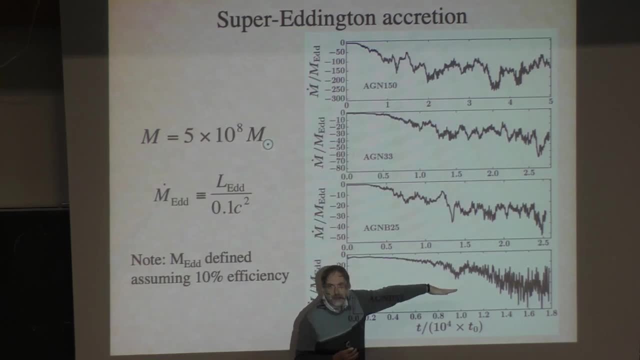 steady state, Although of course there's a finite amount of mass. so if you run it for long enough, eventually this will die away again, And that steady state accretion rate can be much, much higher than Eddington. 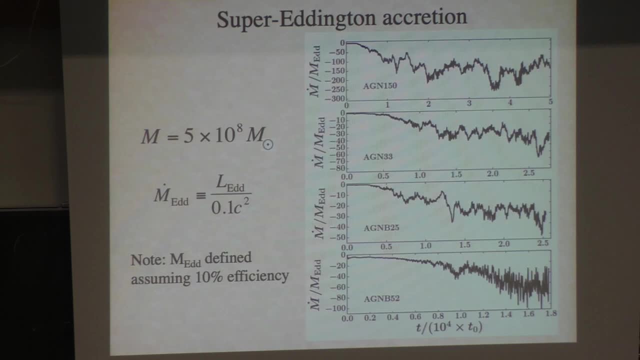 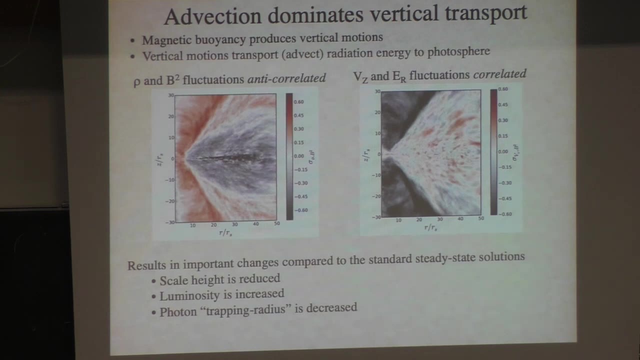 You get super Eddington accretion flows And one very important result that came from that accretion flow is, so you know. let me highlight a few selected results, And here's one highlighted selected result: the role of turbulent transport of radiation. 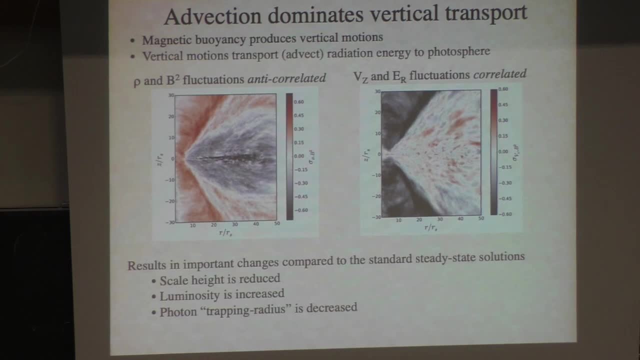 energy in the disk. It plays a huge role in determining the global structure of the flow. So it's shown here in two ways or two sort of steps. First of all there's an anti-correlation between density and magnetic energy fluctuations. 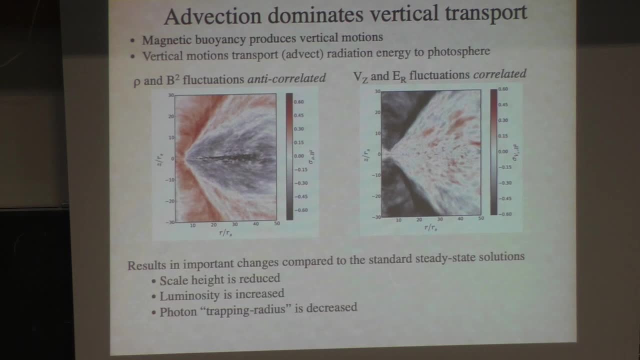 So this is a turbulent flow, MHD-driven turbulence. Wherever the magnetic field is strong, that's a very strong magnetic pressure And the gas density there is a little bit lower on average. So where B squared is high, rho is small. 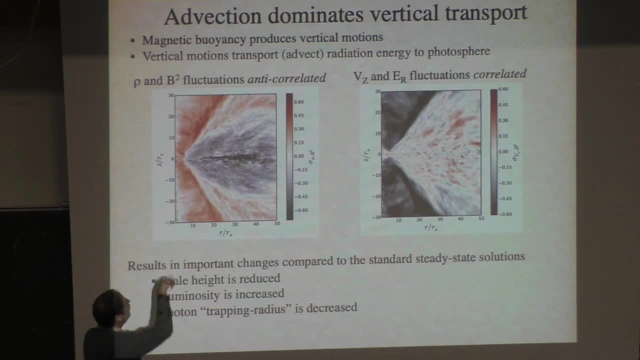 And that shows up by plotting the correlation function between rho and B squared: The black is negative. You see negative correlations in the poloidal plane and the disk mid-plane. So density and magnetic energy fluctuations are anticorrelated. Why does that matter? 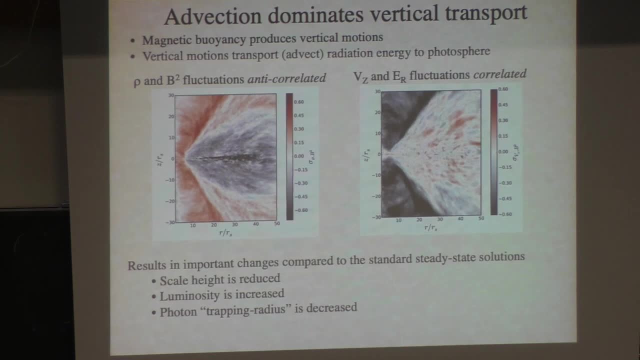 Because these low-density bubbles, magnetic bubbles in the flow, are buoyant, They want to rise out of the disk because they are slightly, they're under-dense compared to the mean, And so that generates outward radial motion, And so there's a correlation. 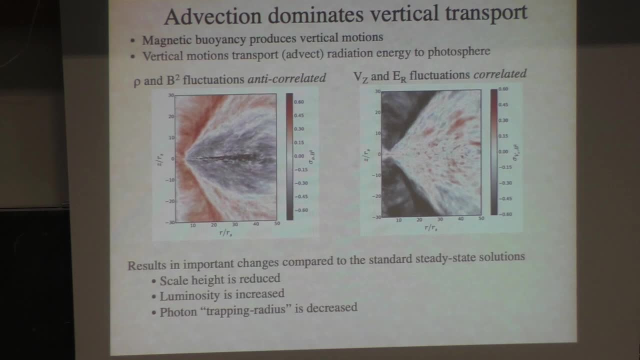 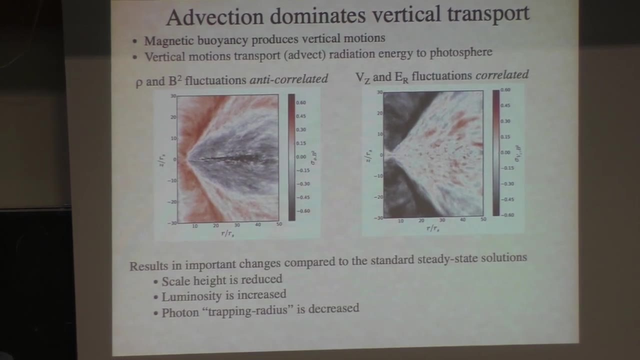 between these density bubbles and their outward radial motion and, moreover, there's a correlation with the radiation energy density, because these low density bubbles fill with radiation. they are a lower opacity. there's a higher radiation energy density inside the bubble. they're rising out and you can see that because 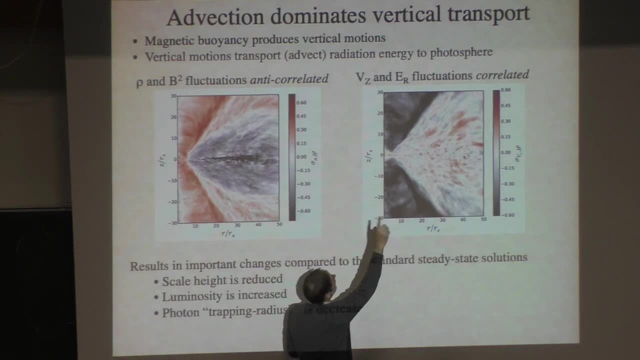 there's a correlation between the outward V Z radial velocity and the radiation energy density that's positively correlated in the volume, and so you have turbulence with the appropriate correlations that you have a net transport of energy by the turbulence outwards, a net advection of energy. it's just like convection where the radial velocity fluctuations are. 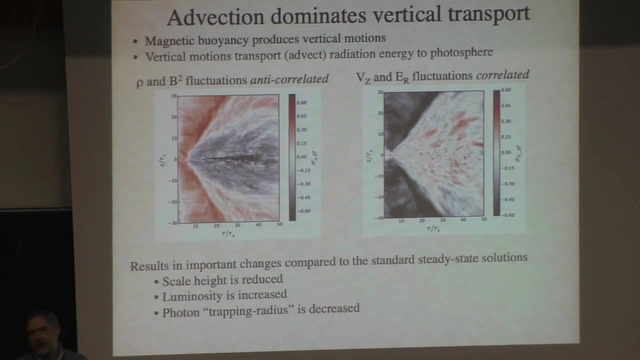 correlated with the entry fluctuations in such a way as to carry heat outwards. same sort of things are happening with through very different physical processes, but the same correlations are emerging. you're carrying heat out and so this convective, advective cooling is very important in cooling down the disk and getting radiation out of the. 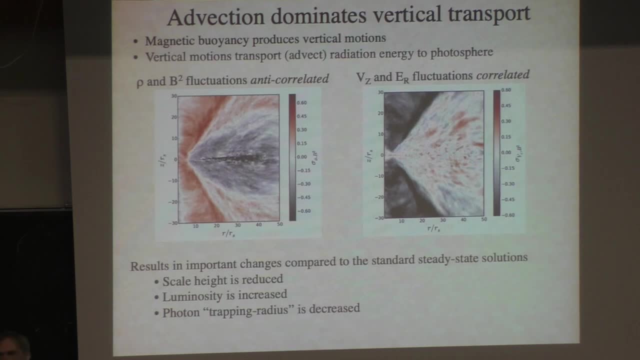 disk. and this is not included in the standard slim disk model where people only consider radiative, of radiation diffusion, and in fact this radiation and convection is actually significantly larger than the rate of diffusion flux. so this is a very important result. that in hindsight is sort of obvious, but in 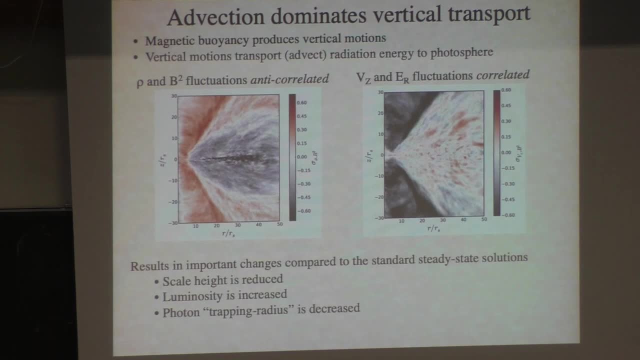 in practice. we weren't smart enough to think about all that. of course, radiation-dominated disks should have a very large advective component to their heat flux, and it needs to be modeled in incorporating the global model of the disk. so the other thing we've done is 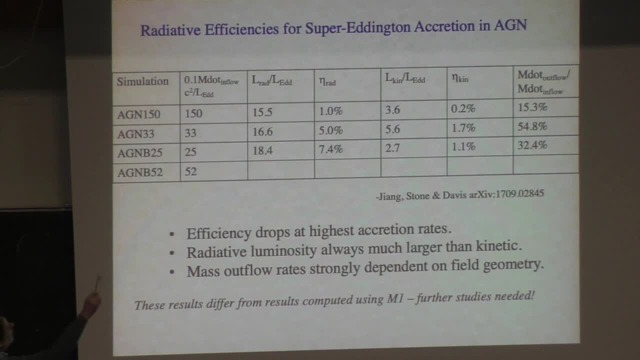 measure the efficiency, as I mentioned. so here's our different super editing simulations. the first column is their mass accretion rate in Eddington units, as I mentioned. the second column is the radiative output in Eddington units and you take the ratio between the two and it gives you an efficiency and you can. 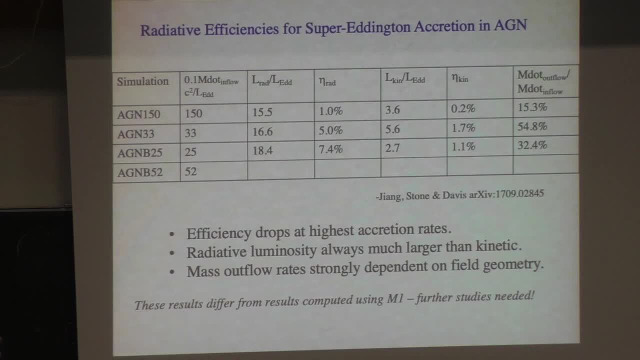 see it varies between about 1% and 7.4%. so the efficiency is very low, the higher the mass accretion ratio. so in such a way is to keep the ratio between radiation, luminosity and anything about constant, no matter what mdot is you sort? 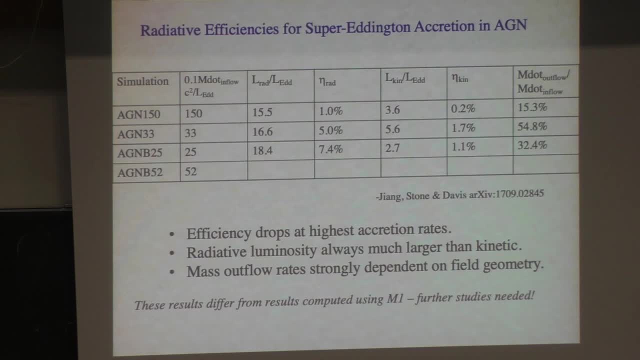 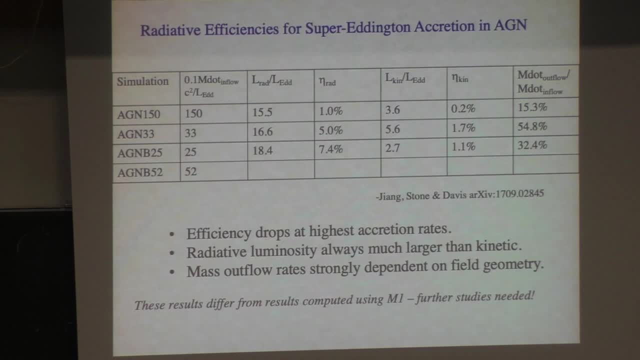 work and how they're going to work and how they're going to work and where those differences lies- the differences in our initial conditions, differences in our resolutions, or what? what's the difference? because these numbers are very important for astrophysics, right, this is what's predicting the luminosity. 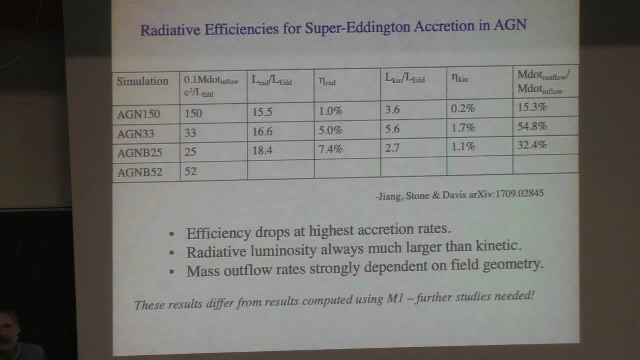 of the sources, and so we need to understand what these rate of efficiencies are very well. so we only have, you know, three models here, and so we need to do a much larger parameter survey really to understand the range of possibilities. but we're at least off to a start in understanding that these. 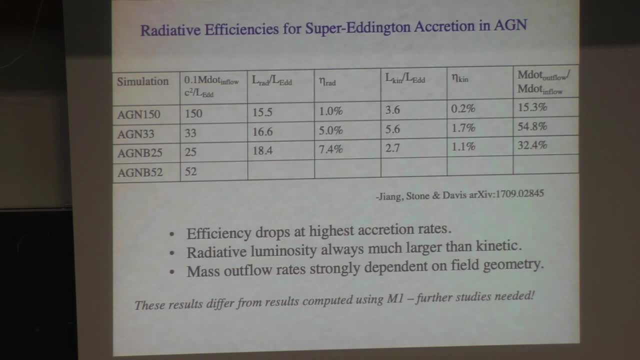 efficiencies tend to be very, very low and go down as M dot goes up. so that's sort of the general trend that's emerged immediately from these calculations. so what about sub-Eddington accretion? I focused on the super-Eddington case, but you still get radiation dominated flows. 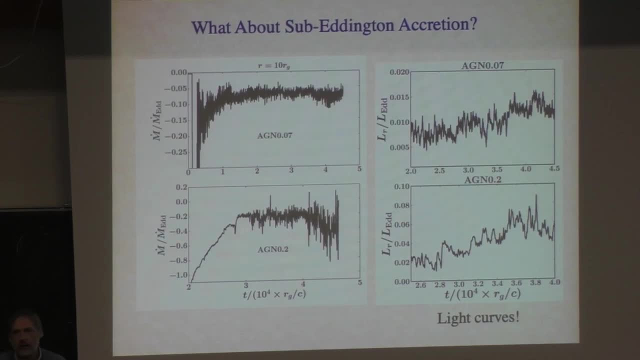 even when the luminosity is, say, only 10% Eddington. and so what about the physics in that flow, in that regime? so we've also done a bunch of models where we have lowered the initial surface density of the torus and given us mass accretion. 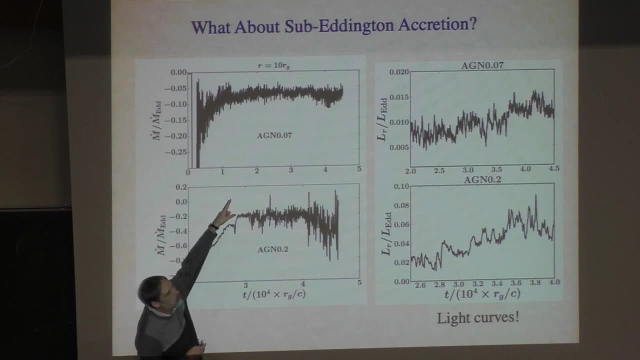 rates that are only 10%, and we've also done a bunch of models where we have only 0.2 of Eddington in this case and 0.07 of Eddington in the case above. again, after some initial transient it settles into a relatively steady state. 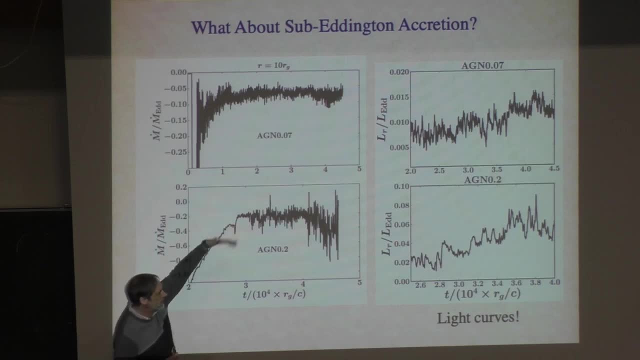 accretion flow, from which we can then diagnose the properties. what's very interesting is that we can measure the output, luminosity, as a function of time. so here it is, between, you know, a factor of 10 to the 4 and light crossing times across the black hole. so that's roughly 10 to the 4 orbits at the inner edge of. 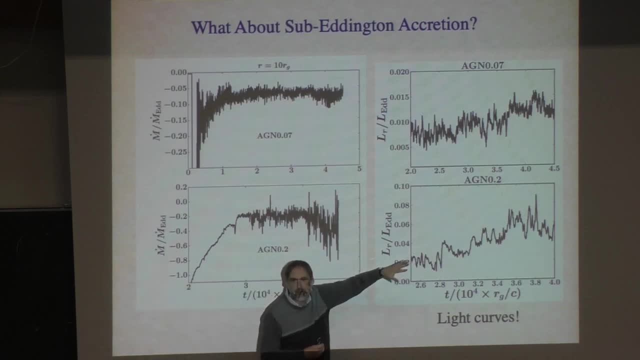 the disk, and so these are the actual light curves in the x-ray that you would measure for these sources. if you had an x-ray telescope and you were watching the inner part of the disk, this is the light curve you would. you would actually observe, and that's very exciting, in my opinion, to be able to now be able to. 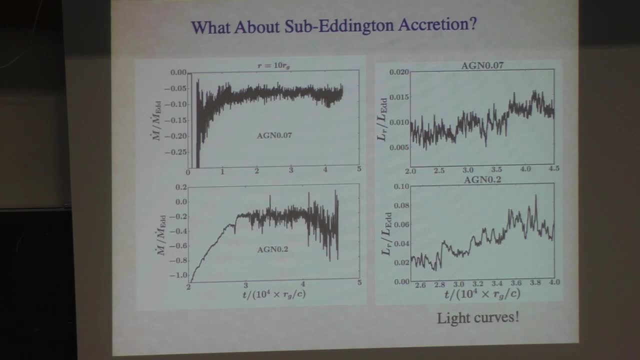 connect directly between a theoretical calculation what's actually observed. many people have used the mass accretion rate as a proxy for the light curve. they've just assumed the instantaneous mass accretion rate gave you the instantaneous luminosity and you can look at the two and you see that. 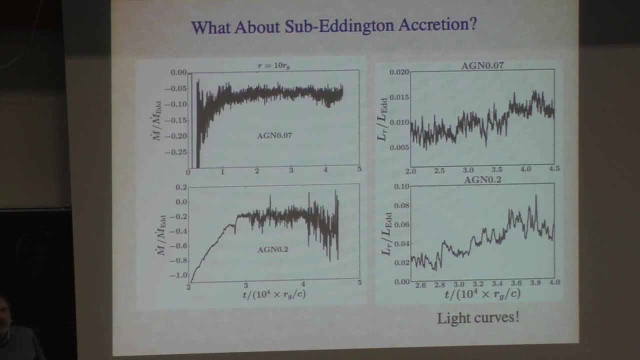 they're totally different. that approximation does not work. you really need to compute the Eddington or compute the radiation dynamics to get the light curve, because it does not follow directly from MDOT. so- and it's another advantage of including radiation in these models and other models is we'll be 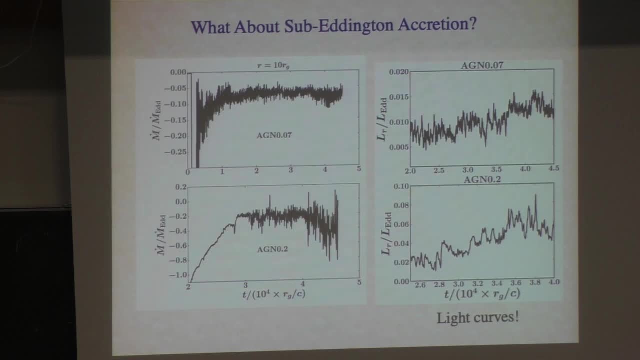 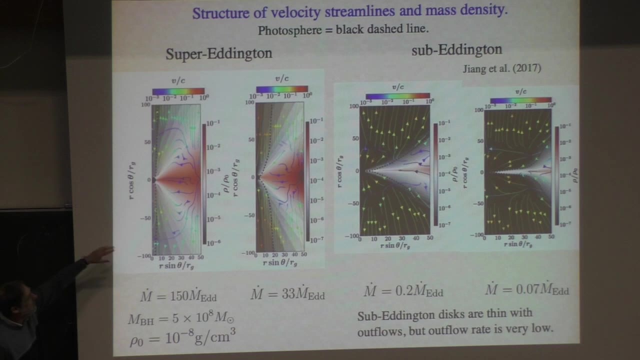 able to make direct connection to the data. so these sub-Eddington flows now are much thinner than the super-Eddington. so here's a panel of four different models. this is the time averaged and azimuthally averaged. structure of the flow. the colors of the. 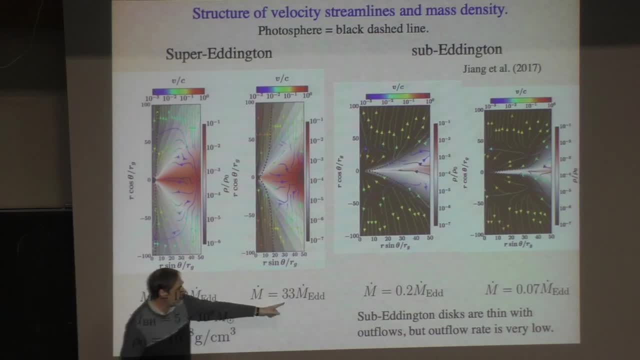 density for the 150 Eddington, 33 Eddington, 0.2 and 0.07 Eddington. as you see, as the mass accretion rate gets lower and lower and lower, the disk gets thinner and thinner, and thinner. with adaptive mesh refinement we're still. 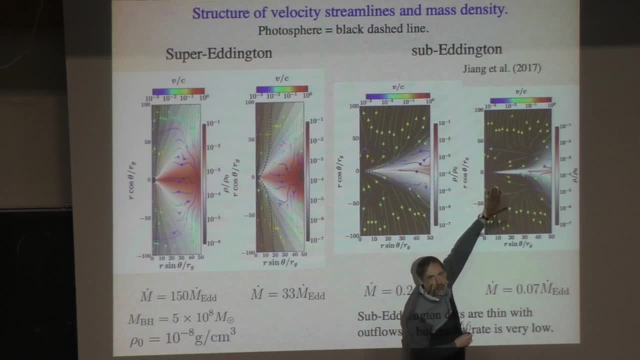 have many grid cells per vertical scale head here, still resolving the MRI in the disk midplane here. but it's geometrically much, much, much thinner than these super-Eddington flows and the corresponding mass outflow rates and winds driven by the radiation field are also much, much lower. and, remarkably, these disks are very thin. they're very. 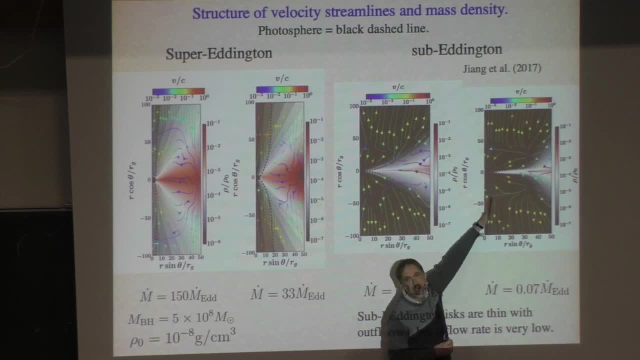 strongly radiation pressure dominated and yet we see no sign of thermal runaway. remember I said that local shearing box calculations using full transport methods had shown thermal runaway exists and radiation dominated disks. they don't appear here. these disks and these global models don't show any sign of thermal runaway, even though we're using the same. 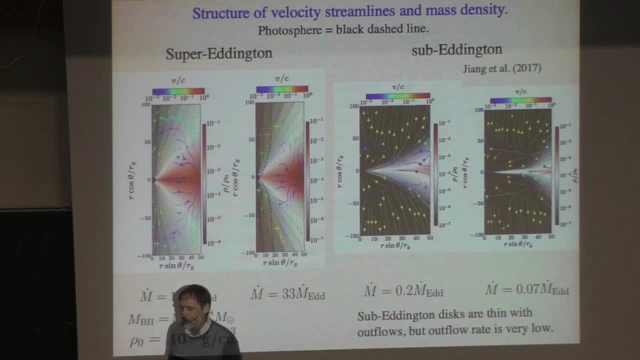 techniques that we used before to model them. so we should be able to capture it? and I think the answer is because a these disks we have very strong magnetic fields and their midplane, and that helps support their thermal stability and, moreover, there's very strong radial fluxes which are not included in local. 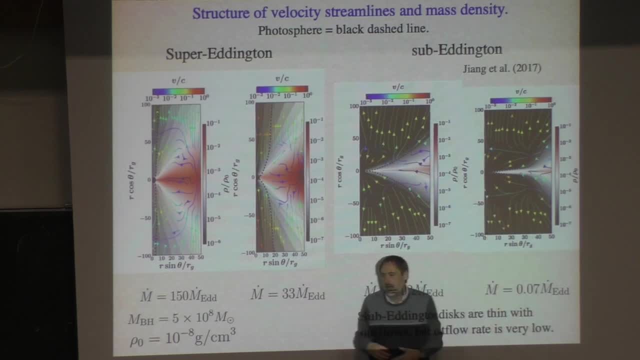 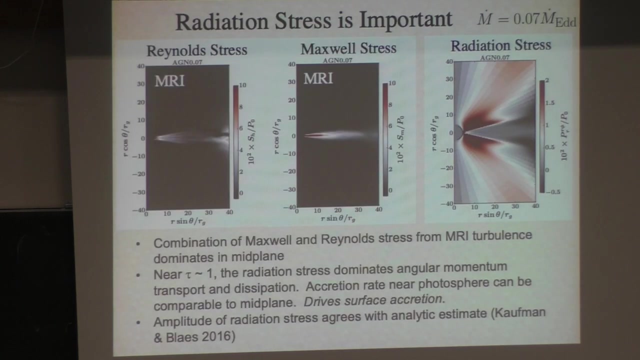 shearing box models and these radial fluxes can can just eliminate the thermal instability. if it was, some region tries to to cool down and collapse, it just simply heats up by radiation from the neighboring- neighboring radii, and that's probably presenting these thermal runaways and then two more quick. 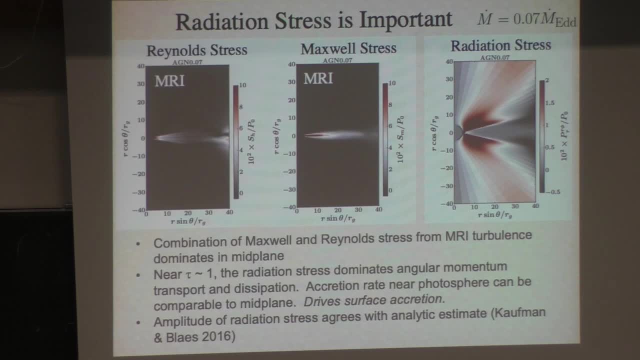 results. another sort of surprising result is that actually radiation viscosity is extremely important in these subeddington disks. so this is the. this is the r5 component of various stresses in the flow: the Reynolds stress, that's the fluid dynamical stress due to velocity fluctuations. the Maxwell stress. 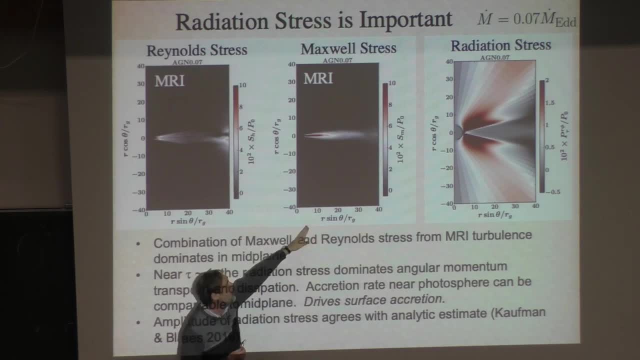 that's the torque through the magnetic field which drives accretion and this is the r5 component of the radiation pressure tensor, which you would associate with photon viscosity. photons can scatter, transport angle into, from one place to another and in a fully three-dimensional system that includes off diagonal terms. so if you're not in 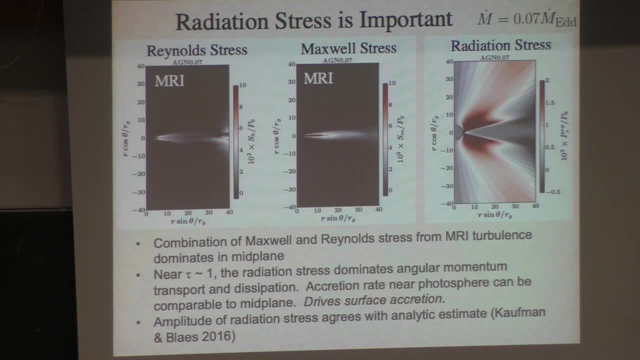 the diffusion limit and the radiation is anisotropic. you get radiation viscosity and so this is plots, all scale to the gas pressure, and you see that in the midplane it's all MRI. so for these very, very thin subeddington disks, accretion in the midplane is all being driven by. MHD turbulence, as you might expect, but remarkably above the disk there's significant transport due to radiation stress. there it's optically thin. photon mean free path is very large. photons are scattering across a very large range of radii. that's producing very large torques as a photon emitted in the inner region. 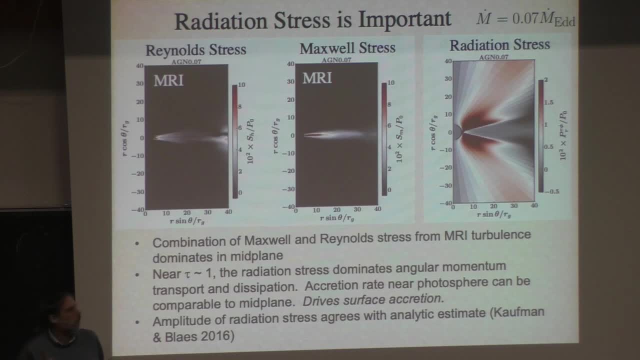 transports angular momentum and scatters off a photon or a particle farther away, and that actually produces an interesting coronal accretion flow due to radiation stress- again something we didn't expect, but emerges self consistently in these subeddington flows. it doesn't occur in the supereddington. 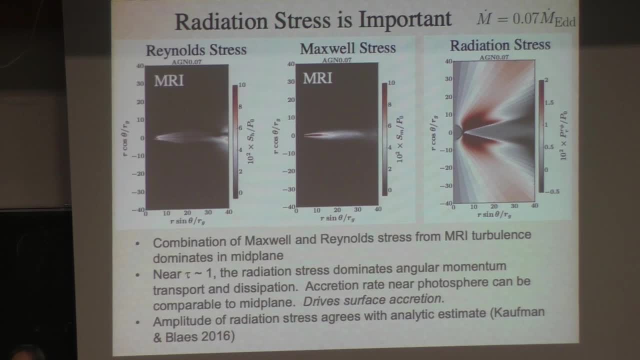 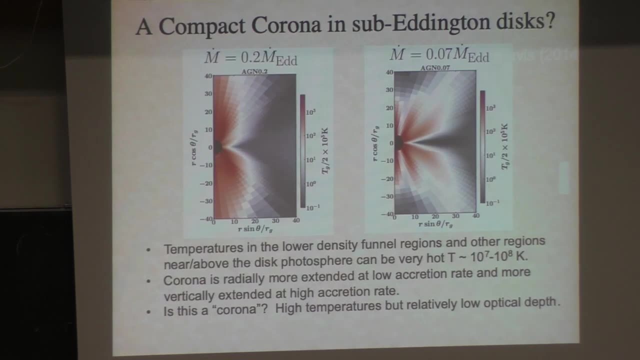 flows because they're so thick there's nowhere where it's optically thin enough for the photons to contribute to the stress. and then, finally, I mentioned these corona again, in these subeddington flows: 0.2 and 0.07. so this is now the 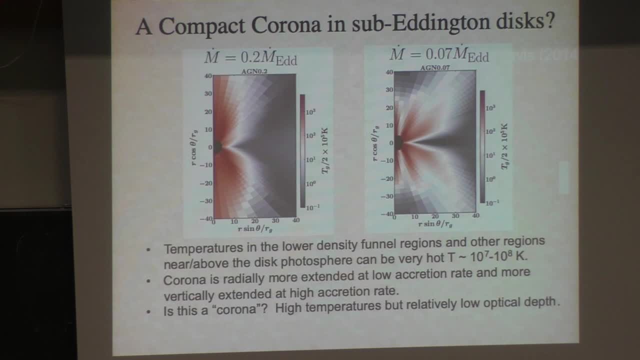 temperature in the, in the plasma averaged over time and azimuthal angle, you begin to see, over a factor of 10, 20 and radii, a very, very hot plasma emerging above the mid plane, above the photosphere. so you're generating temperatures that are orders of. 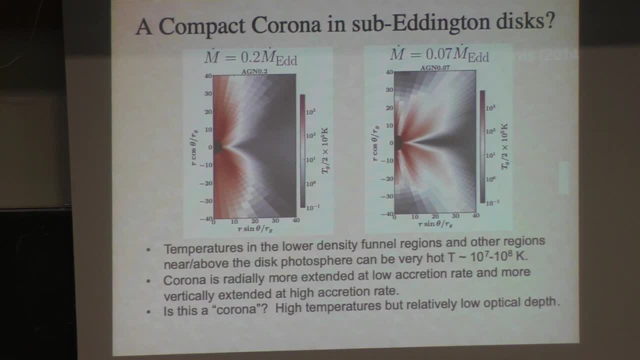 magnitude higher in the corona and the in the low density upper regions of the disc. then you are in the mid plane. and why is that? it's simply because there's still turbulence and dissipation in the upper layers. but because it's optically thin, it can't radiate, can't cool down. so whatever energy you're pumping in to the 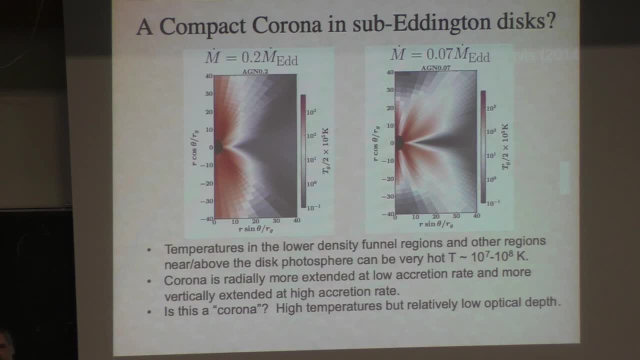 plasma due to dissipation of MRI turbulence. it just keeps heating the plasma up, it can't radiate it away and it results in an extremely hot, you know large radius corona extending for a decade or more in radius. and again, we didn't put this in by hand, it's just. 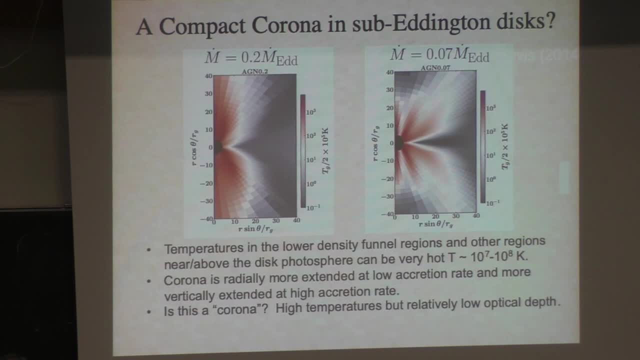 emerging self consistently. when you have this very, very thin disc turbulence above the mid plane with the density is extremely low, it's above the photosphere- can't cool. it gets getting very, very, very hot and it turns out that actually is presenting or resulting in these non thermal spectrum. 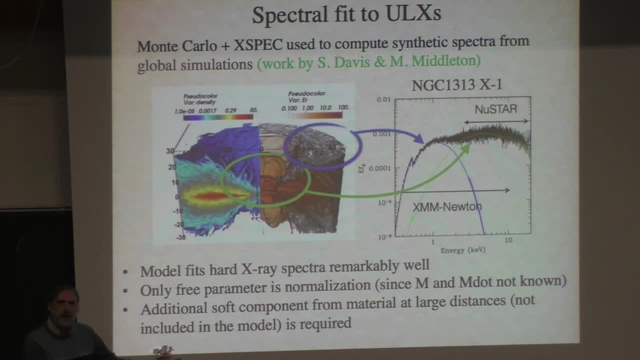 so we'll put those famous examples over some more time. OK, so two of them. an experiment out of that whole kind of city from in the middle radio revelation: majority in Exodus of sa. and so we take one of those models, we feed it into a Monte Carlo ready Birds solver to compute the frequency dependent transport. 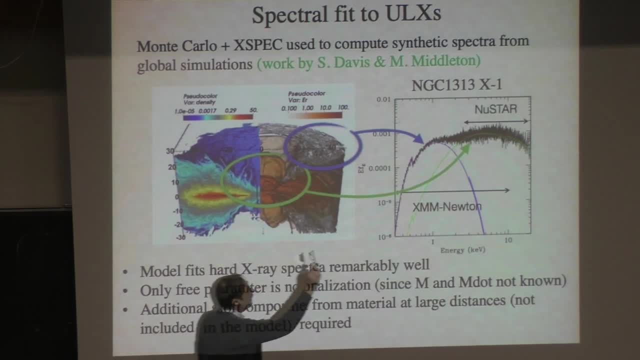 to compute spectrum and then we then passed that through response function of detectors on using X speck and compared to observed. so here's New Star and XMM observations of a very particular it works. source: you with the phone number on top, and then the wiggly line is the observed data and 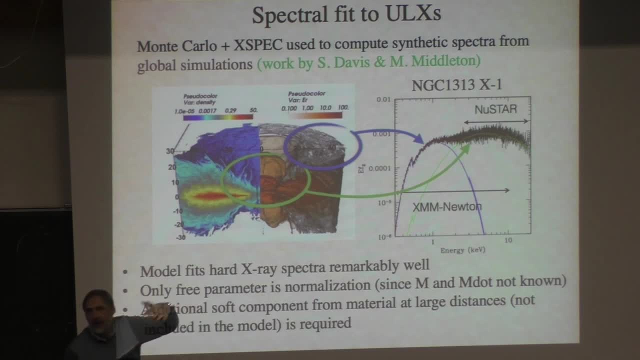 So help us when you're mad, we do some multi throttle data from То cook你可以 line goes through those points extremely well and that's the, that's the spectra that emerges self consistently, with this green component coming from this very hot corona above the mid plane and the blue part being the central disk, which 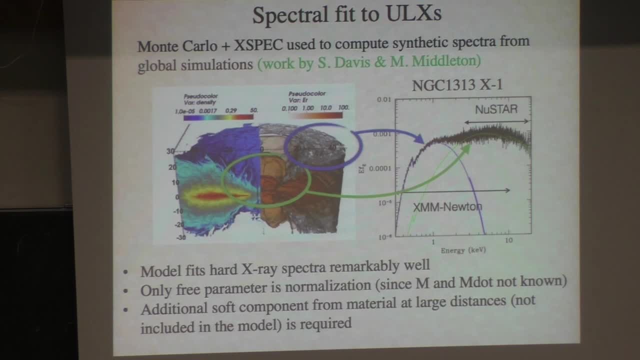 is more thermal, and so it's very encouraging that we get actually remarkably good fit to the observed spectra for these sources without really doing much of anything except just post processing the flow. there's really no free parameters in terms of being able to change the spectral shape, it just 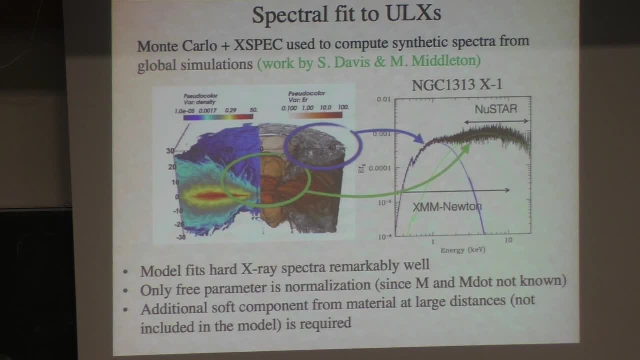 comes self consistently out of the density and temperature field that we get from from the simulation. so it's an encouraging step that maybe we're on the right track to understanding these corona. for example. there are still issues because doesn't work in all sources. I'm showing you sort of the best. 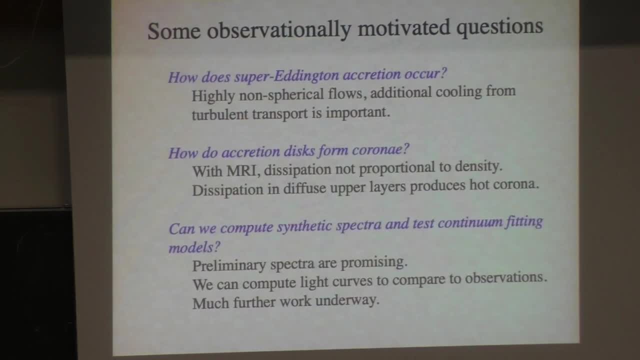 example. so I began my talk by some observationally motivated questions. how does super eddington increase you to occur? it occurs because the flow is non-spherical and most of the radiation is non-spherical, and most of the radiation is non-spherical and most of the radiation is. 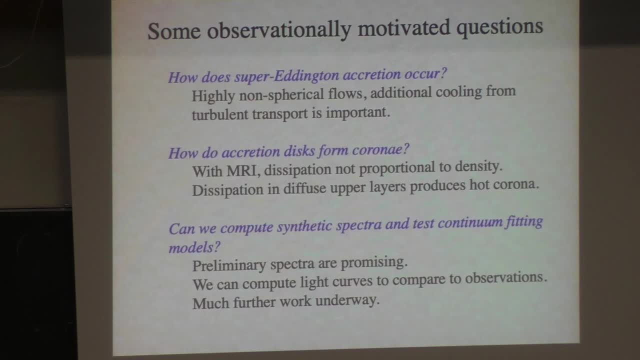 coming out the poles, and that allows the material equatorial plane to accrete inwards at super eddington rates. how do accretion just corona form? corona it's from dissipation, of turbulence, but in dissipation and optically thin regions above the mid plane where it can't cool down, it gets very, very hot and just the. 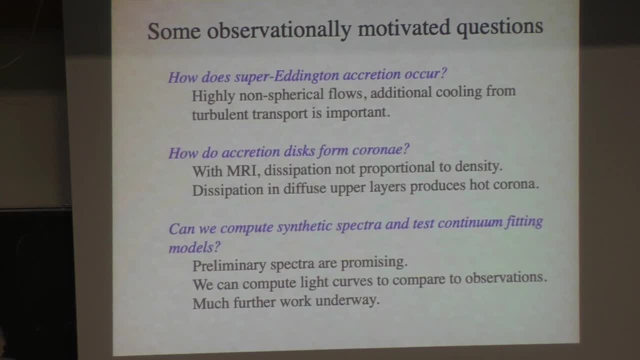 thermal heating from the turbulence alone is enough to create these apparently non thermal spectrum which are actually just a sum of many black bodies over a wide temperature range in the corona. and can we compute? synthetic spectrum test can fit continually fitting models. our first attempt at doing this is very 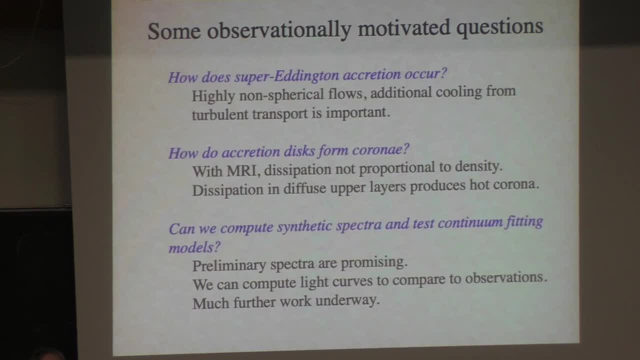 encouraging, but we're still a long way from computing general spectra all the way up to the optical and UV. that's much, much farther out in the disc than the central regions were considering, which is really only the x-rays. so in order to compute a broadband spectra that includes UV, optical, we're a long way to. 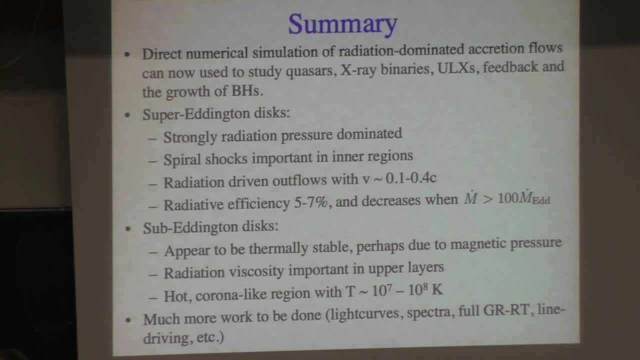 go, but at least we're on, I think, on the right track here. so so let me summarize just to say that, you know, I think we're now in the era of doing full radiation hot in the mix in three dimensions, incorporating radiation field as well as an NHT, and that enables all sorts of new problems to be tackled in high. 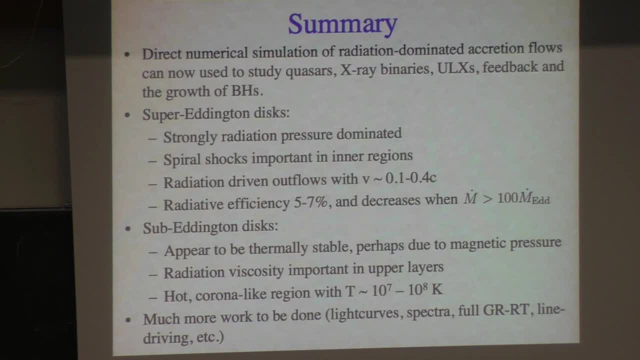 energy, astrophysics as well as other fields, were, you know, rated of cooling? maybe momentum transport, not important by photons but cooling candy. and these techniques can be used in other regimes as well, and I talked about black hole. accretion is one example. I told you about the various results for Super. 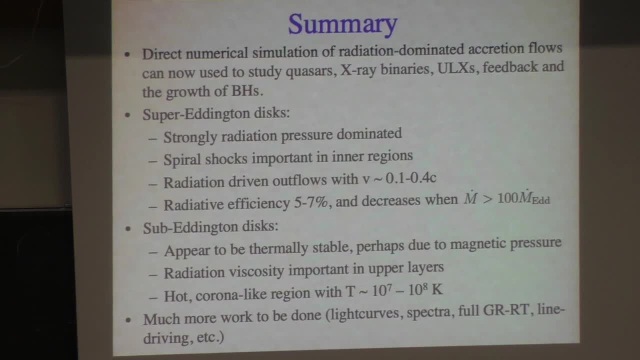 Eddington and some Eddington discs. I will go over all the results again, but just to say I think This is a start of an exciting era where now we can actually compare directly theoretical calculations with observed light curves of spectra and so on and understand the interaction of radiation matter. 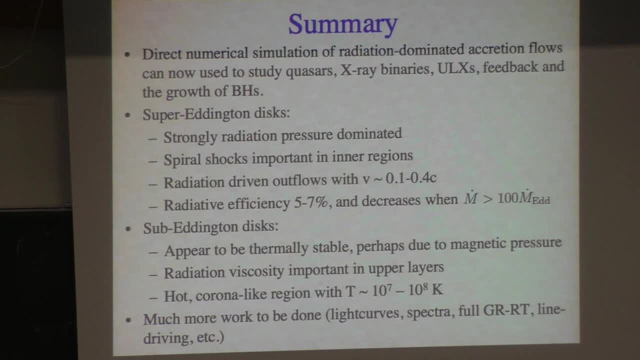 for many, many astrophysical systems, And this one's sort of interesting because it's so extreme. but there's many more to come. I think, and I think you'll see a lot more work in this regime in the future. And with that I think I'll close. 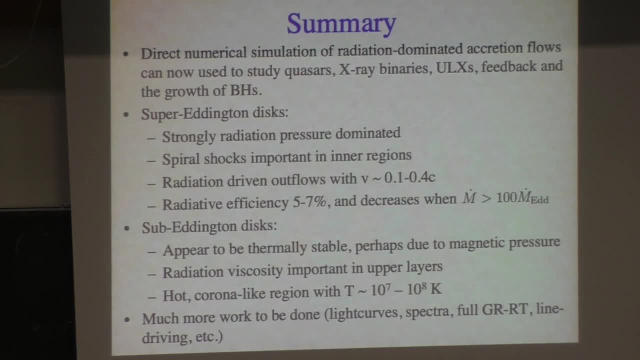 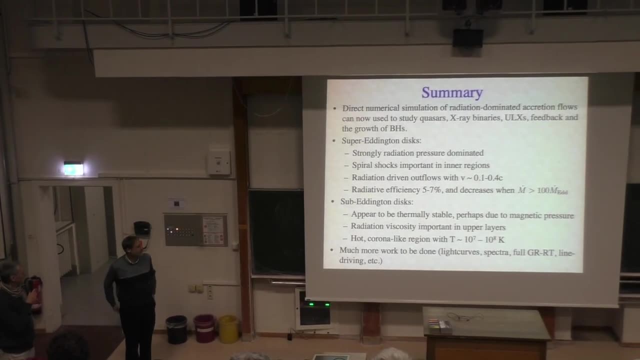 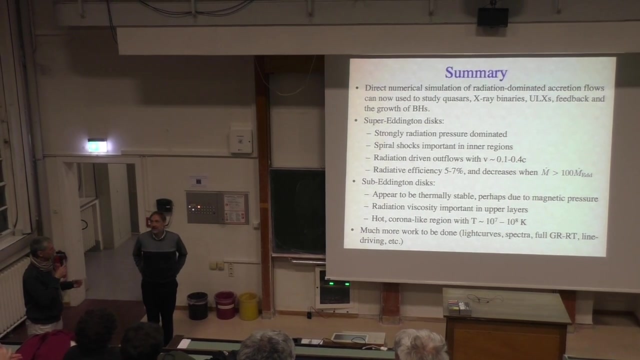 So thanks, Jim, for this fantastic talk about what we can learn about accretion disks around supermassive black holes and smaller objects from really good and high-precision and high-physics numerical approaches. We already had some questions, but there must be more. 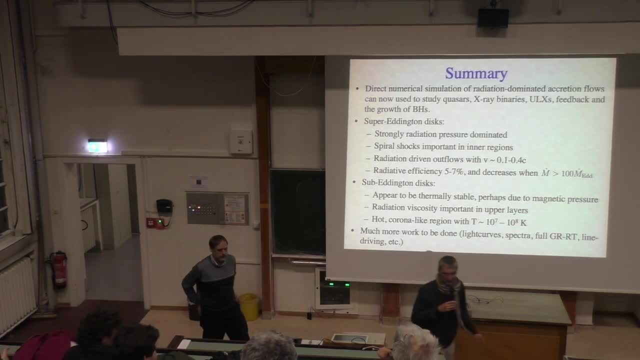 Yes, I'll start with Stefan Jordan. Yeah, very impressive talk. You know, you told us that when we have not so high temperature, also iron ions are important. I guess that's an extreme NLTE iron. so how do you? 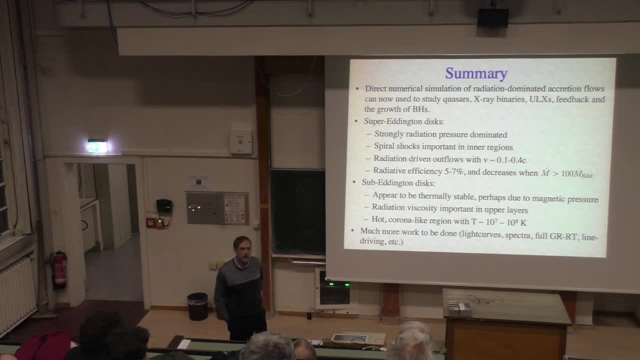 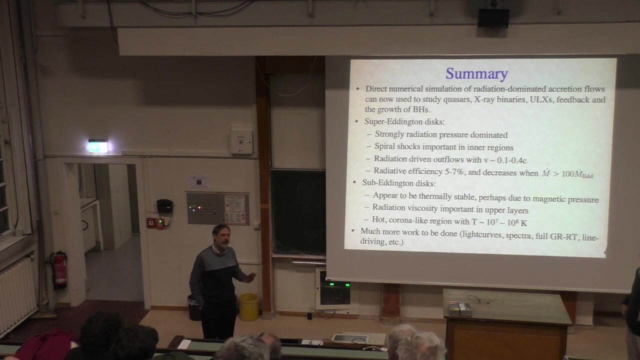 do you consider NLTE effects in the calculation of the spectra? I guess that would be extremely additionally expensive to the otherwise very expensive code. Exactly So at the moment we of course, only include LTE and we're using opacity tables that are being pre-computed for plasmas at these temperatures. 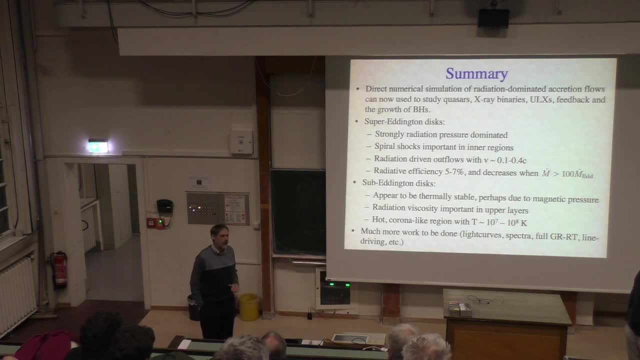 and typical solar abundances and so on. But you're absolutely right, There's many circumstances where the plasma is probably non-LTE. So, for example, in the upper layers of the disk, where there might be a wind, it's probably going to be non-LTE. 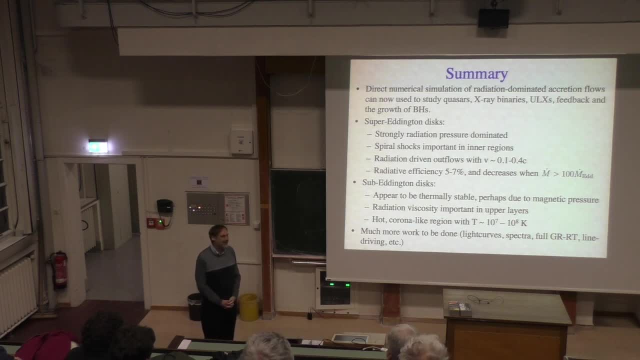 like a stellar atmosphere, But incorporating that it both scares me and, you know, excites me. I hope there's lots of young people here interested in following this, because I think it's going to require their generation to figure this out So ideally in the future. yeah, it would be wonderful. 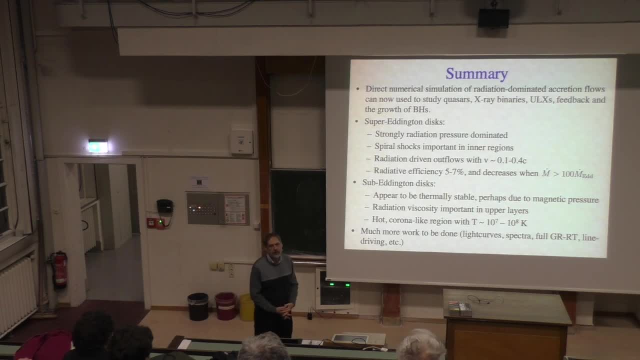 if we could incorporate a basic model for non-LTE processes, because what we've learned- I mean I didn't show you the x-ray binary results- so the differences between the solutions with different opacities, but they're actually quite different. 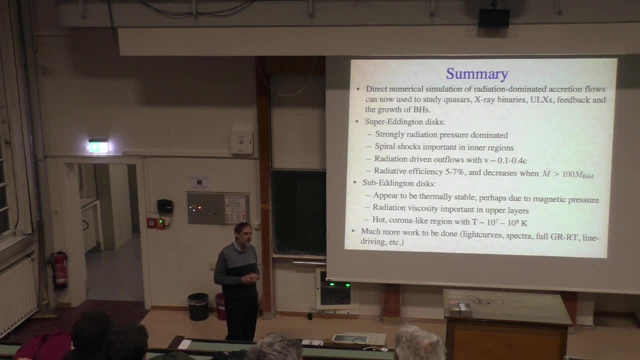 So opacity really matters and therefore, probably in the future, getting the non-LTE effects when they're important is going to be crucial for interpreting some So much, much, much to be done down the road. After reading the abstract of your talk. 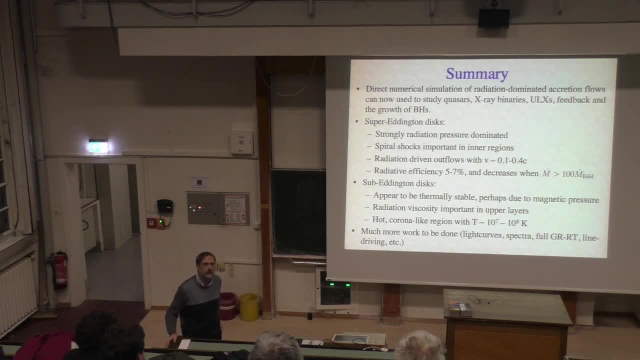 I was expecting a convection term in the radiative transfer equation, but that wasn't there. This is why I was asking for this n vector. Ah right, So if you were, But you explained that convection is important. Yeah, if you were to take the moments. 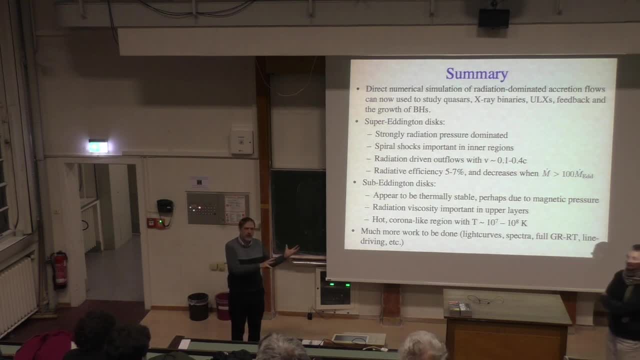 of the radiation transfer equation, then you would see things like the the convective terms appearing, because then you would be transporting energy, density and flux tied to the Eulerian mesh, But instead we're just treating the radiation field as a specific intensity. every grid point in space. 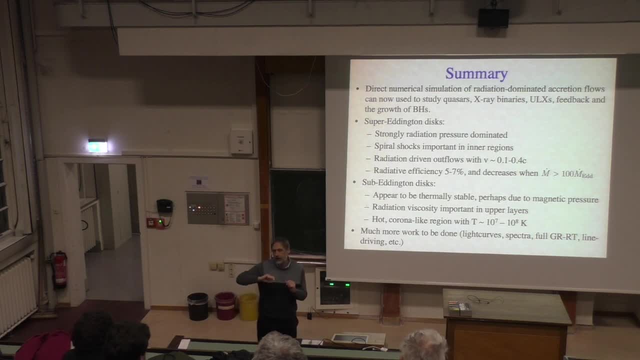 The photons are not being. you know they can scatter and and interact with the matter and therefore be transported in that sense. You know, the only interactions between the photons and the matter are captured in the source terms on the right-hand side, and that's. 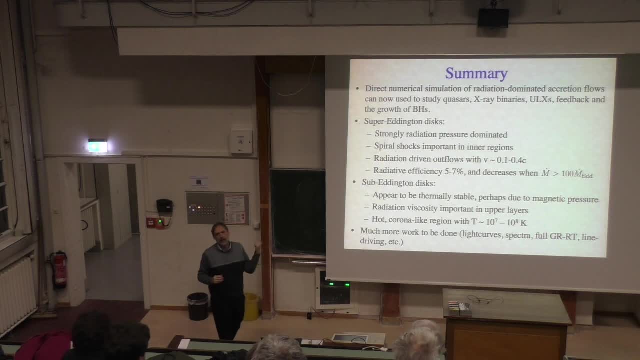 where the convective parts come in. So so they're not in. they're not in the transport. The only transport is. photons are emitted in one place and they travel somewhere else, and then they get scattered again or absorbed, and then they do the same thing all over again. 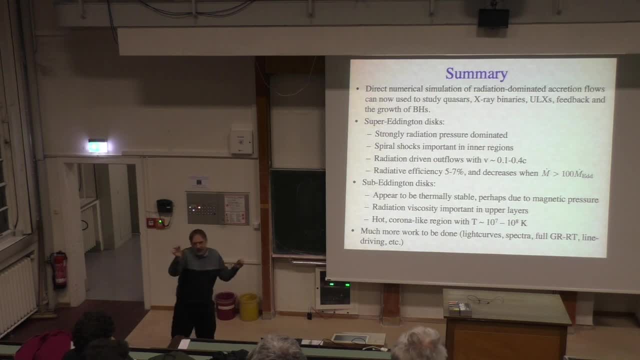 And if they're in a moving medium, then the scattering process apparently moves along. and then that, where's that next transport? But that's all buried in those scattering absorption terms when you're solving the equations in this form. So, Christian Fendt, 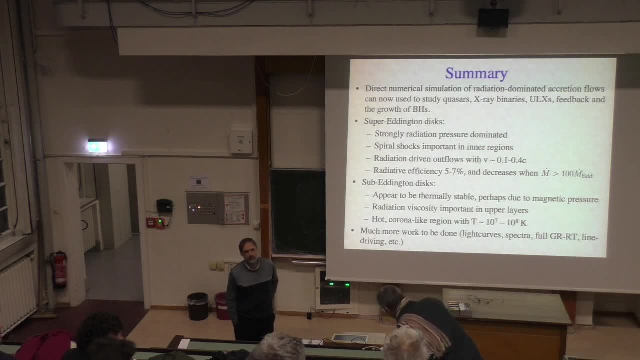 I have a very basic question. So you remove angular momentum from the inner disk by the MRI, So where is that deposited? So the the outer disk should be super-Caballarian, maybe at some stage. That's right. 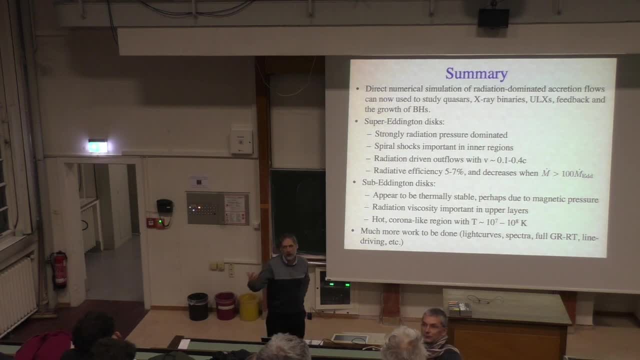 Is that true? So yes, absolutely right. I mean, the angular momentum is conserved, It's got to go somewhere. So these boxes are very large, three orders of magnitude, and I only showed you the inner 300 gravitational radii. 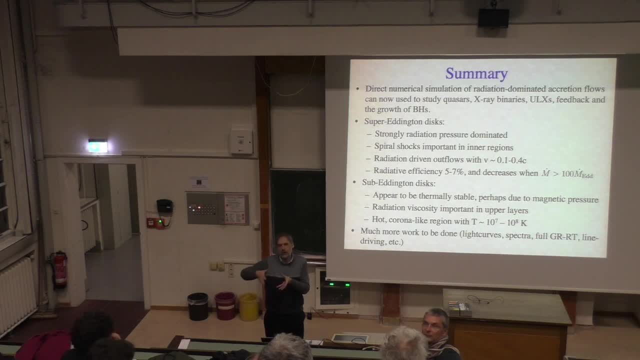 and the outer part, the outer edge of the torus is slowly moving outwards. you know, because angular momentum increases rapidly with distance, It only has to move a little bit to, you know, suck up all the angular momentum that comes in. I mean it's a little more complicated because there is an outflow and a wind. So you know a problem near and dear to your heart. there's a jet and there's magnetic torques and there's angular momentum fluxes carried away by that. It's not. these winds are not magnetically driven so they're not sort of like protostellar jets. They're mostly radiation driven but nonetheless they still carry a little bit of angular momentum. So the overall angular momentum budget it has many contributions. 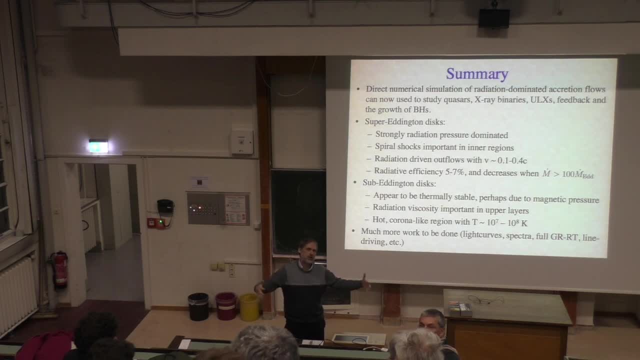 and one of them is slow expansion of the outer part of the torus. So who's next? So maybe I can inject a question. I was wondering about non-ideal MHD effects. Do they play no role at all in these conditions? 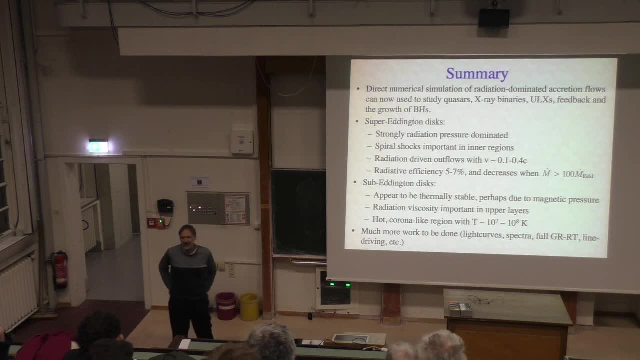 or is there something to worry about? Or more physics that needs to be, that needs to be included at some point. So I can say, I can say yes and no. The no answer, non-ideal, MHD, is not important. 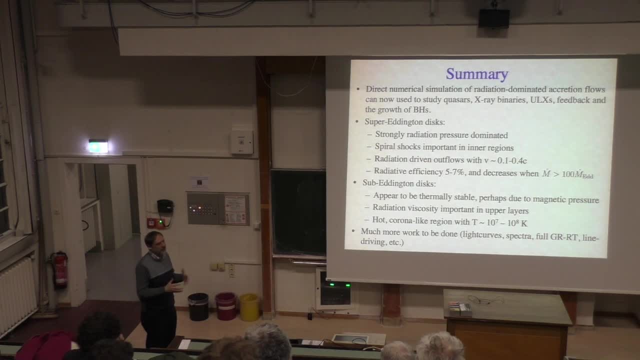 is because these things are sort of the poster child for fully ionized plasmas. These are million degrees Kelvin, you know, even iron is fully ionized. that's really hard, And so in principle there are no neutral species left at all. 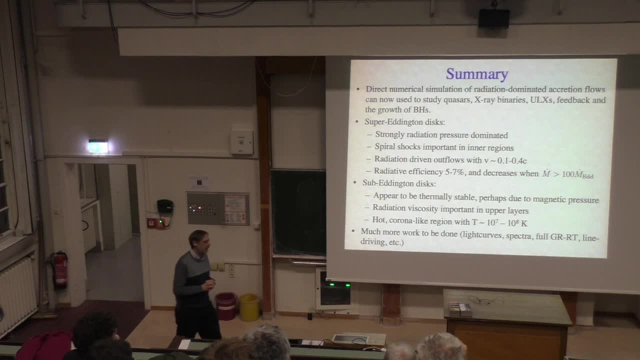 and you shouldn't see any non-ideal effect, MHD effects. That's my no answer. My yes answer is well, well, well, actually, there's a radiation field which is strongly interacting with the electrons, but not the protons. 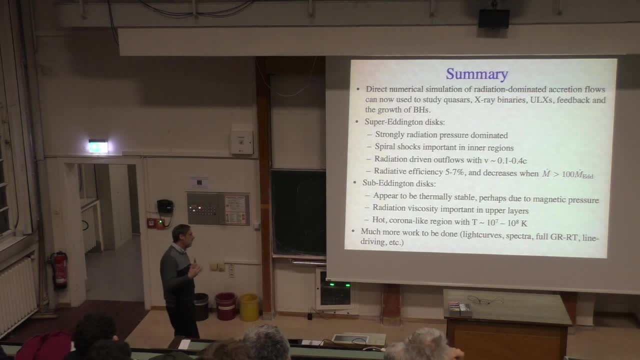 And at these energy densities you can begin to get weird radiation resistivity effects where the electrons begin to drift relative to the ions because of radiation forces, And that's a whole high energy phenomena that we haven't tried to incorporate in here. So there may be some non-ideal MHD effects. 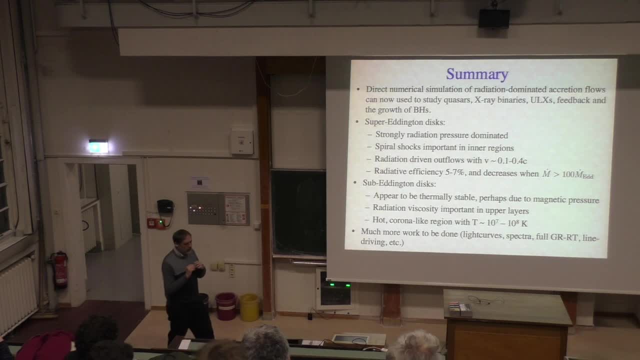 that are important in extreme, extremely extreme regions of parameter space in these flows, but we haven't tried to explore them at all. It's probably not important at all in the mid-plane of the disk, where the optical depths are so large. the resistive scales would be very, very tiny. 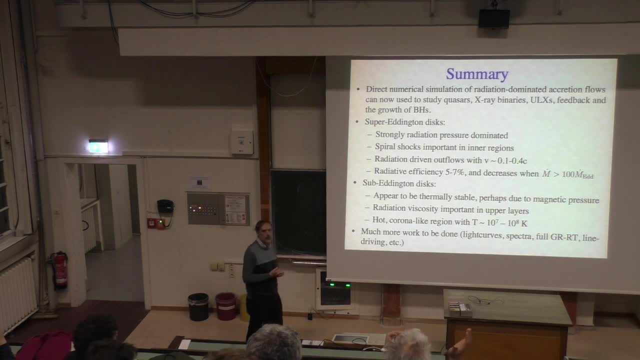 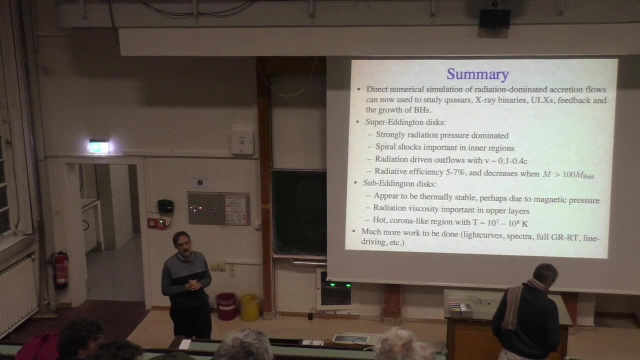 Okay. So second question by Christian. It's another basic thing. You showed the system of equations you're solving. There was no equation of state, but it's kind of incorporated. Yeah, For addition pressure and gas pressure. what do you assume? 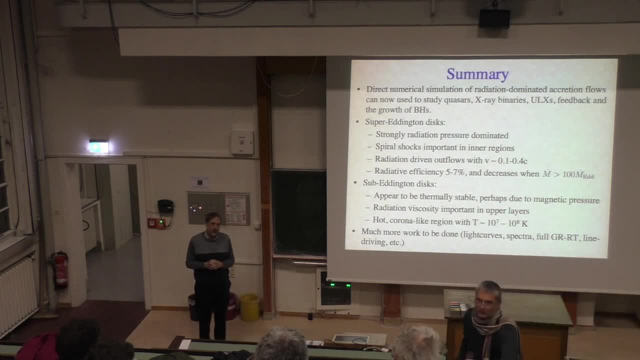 So we need a closure relation for the gas pressure. and that is just an ideal gas, Again, because it's fully ionized and it's non-relativistic, you know it's not degenerate or anything like that. We don't. so an ideal gas law will work very, very well. 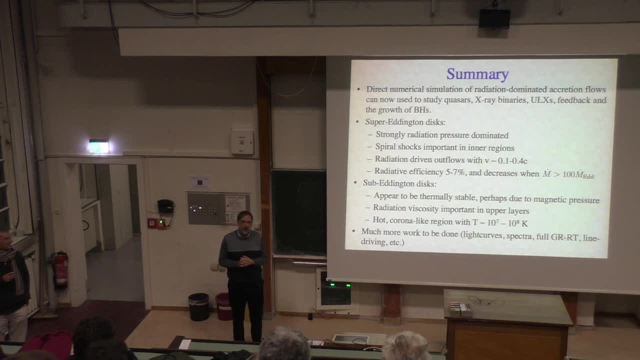 So that's the simple one, And the beauty of solving the transfer equation directly is we don't need some closure relation for the radiation field- There's no radiation moments- and we don't need a relationship between radiation pressure and energy density. and that's what FLD is. 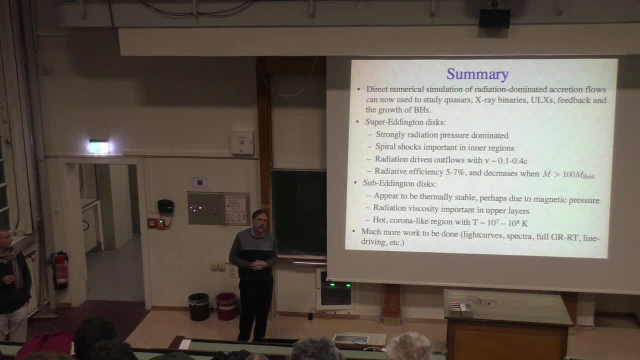 That's what M1 is, But because we're solving the transport equation directly, it's basically the Boltzmann equation for photons. we know what the distribution function is, We know, you know we can take its moments to compute the forces and so that actually simplifies. 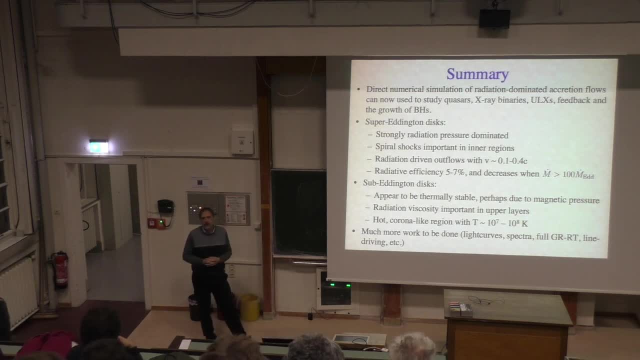 the problem in that you don't need to make some assumption, some arbitrary assumption about what the closure should be. And that's the great challenge of radiation hydro is. there is no closure that works for all flows and in all circumstances. Just simply not true. If it's optically true, 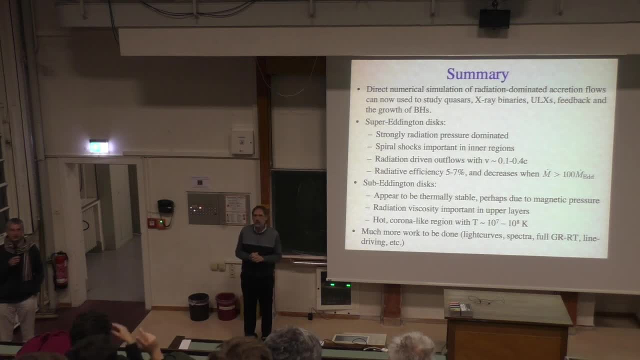 If it's optically thin. Okay. So next question, Ben, and please forward here. So I'm curious: with the major rewrite you did, how much of adapting to new architectures was explicitly including things like AVX 512 instructions versus writing. 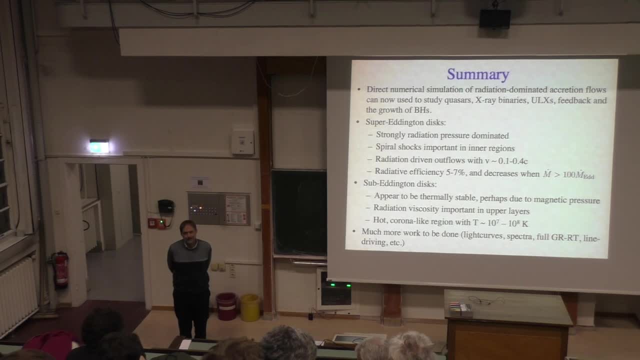 things in a way that automatic vector authorization could work and you just stay out of the compiler's way, Right? Very good question, And our philosophy is: I don't want to have to embed SSC instructions. I don't want to embed machine code in my source code. 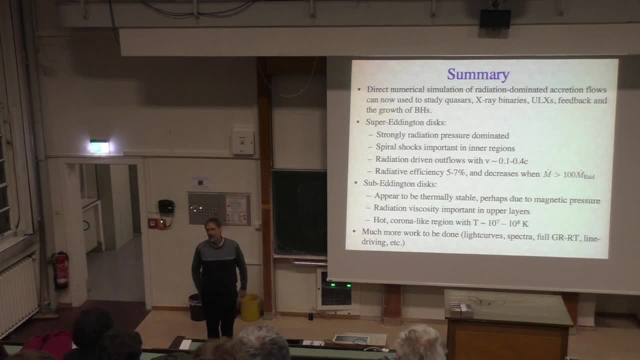 because it's just way too hard and I don't have time. So if the compiler can't do it, then it's not going to work. So the key is to enable the compiler to auto vectorize, And the key for that is to write data structures. 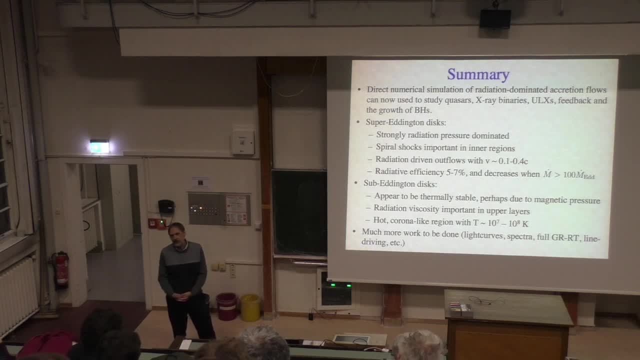 and loops that the compiler recognizes as being simple enough to vectorize. So that's what we spent our time was figuring out what data structures would automatically vectorize easily with the Intel compiler suite and then adopt those for the entire code rather than trying to embed explicit SSC instructions. 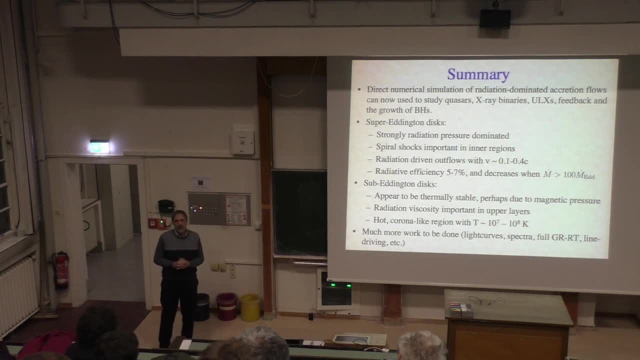 or AVX instructions function calls in the code. I mean, there are many people who do that and I admire them because they're way smarter than me. They know how to write code like that, So let's see, Thanks. I'm just wondering: you put the full GR? 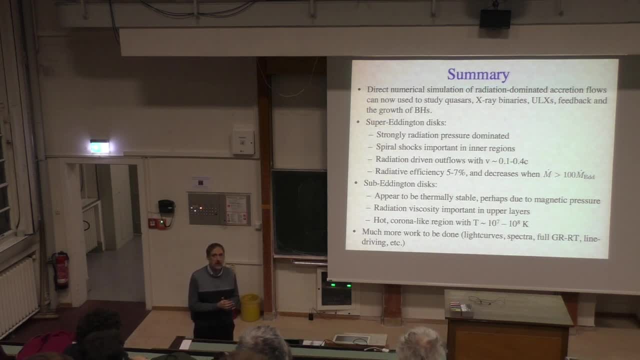 in the much more work to be done. Do you have any clue what would happen for like a spinning black hole instead of like a non-spinning one? Say that again. If you assume that the central black hole is spinning Right, So that requires, as you say, putting in the GR. 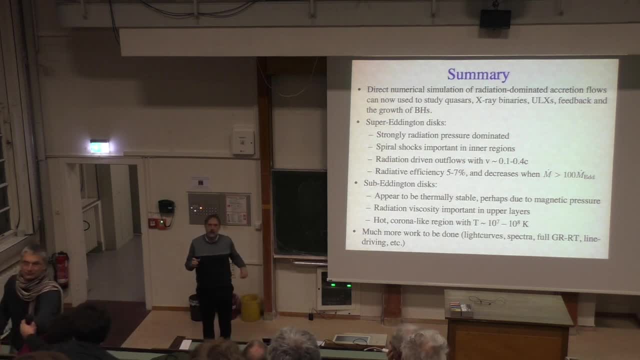 And there will be a big difference between. so there's been a huge amount of work in studying black hole accretion flows without radiation And especially focusing on the production of jets, And there it's been discovered that you certainly need a spinning black hole. 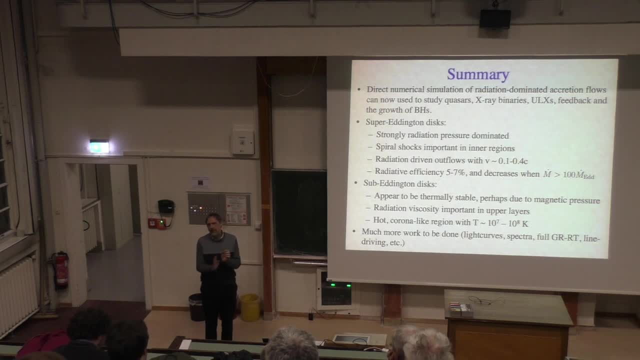 to produce relativistic jets And, moreover, you need net magnetic flux on the horizon so that you get the, you know, the spinning magnetic field lines which then drive pointing flux and a relativistic jet beam. So you need those two things to get relativistic jets produced. 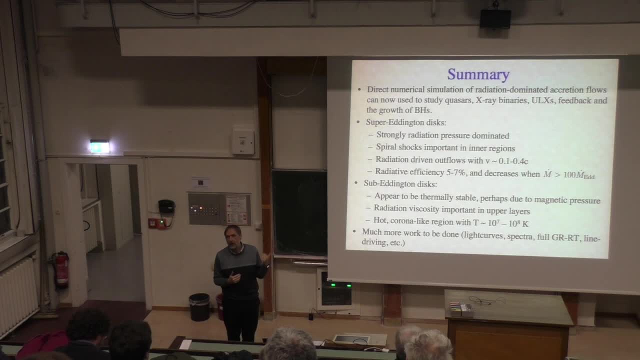 Of course that doesn't appear here because we were not doing the full GR. We now have a a full GR version of the radiation transport. It's much more complicated because that little N dot grad I term is now following photons along geodesics. 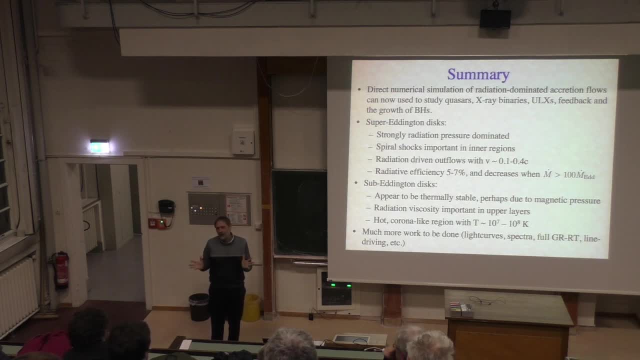 which are no longer straight lines, they're curved. But it took us a little while but we figured it out and we can do geodesics in curved space time. So one of the next projects is to repeat this with spinning black holes in the middle to look at the formation. 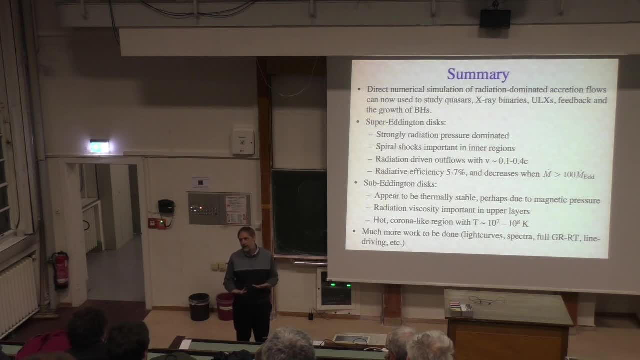 of jets and to understand the interaction of the radiation field with these relativistic beams that you're generating. For example, you can get radiation drag. You know, you might think radiation accelerates outflows, but in fact you're already accelerating the stuff. 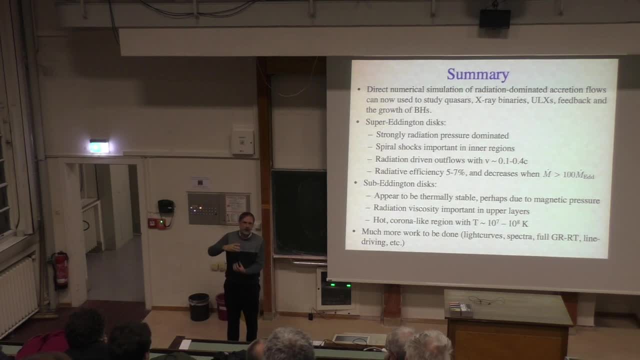 to relativistic speeds through MHD and that's going faster. In that sense, the photons are actually a background medium that produces drag and slows you down. You're trying to move through this very dense radiation field and that slows you down because the Doppler shifting. 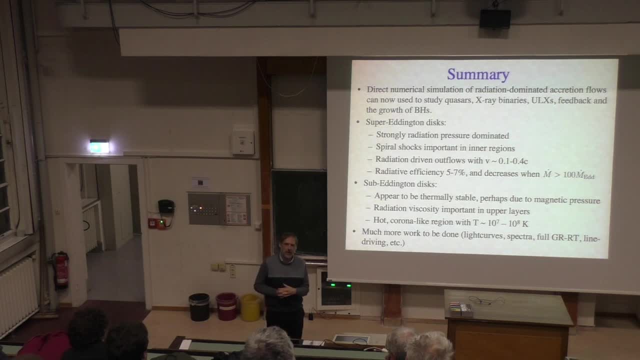 And so we want to understand how much that affects the production of collimated jets in these. So yeah, we're looking forward to doing the full GR calculations in the next couple of months actually, So maybe I had a second question. 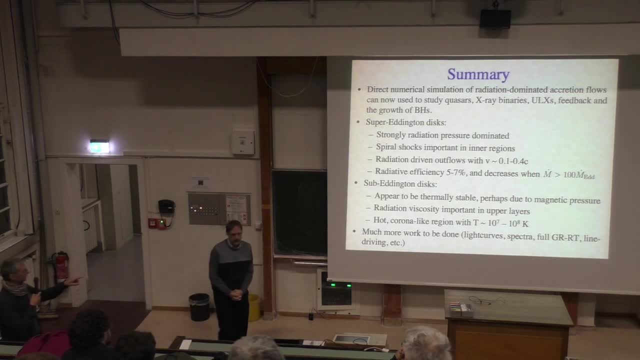 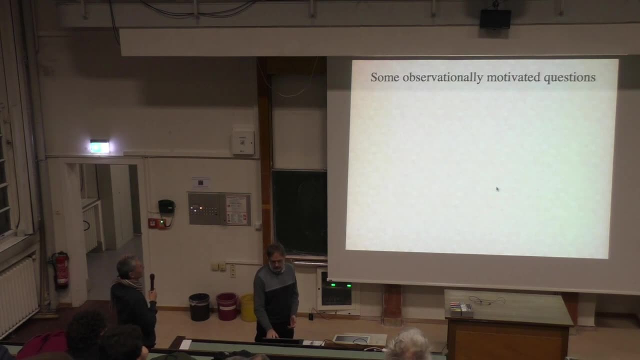 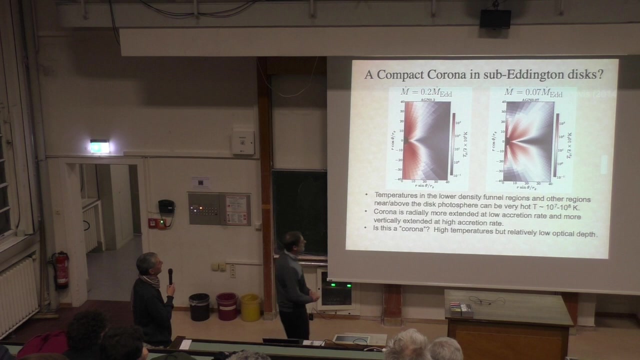 In the- I think one of your last slides where you have shown the no one further, There were strikes, radial stripes here, on this one on the right hand side. Why are there radial stripes for the In the red? In the red? 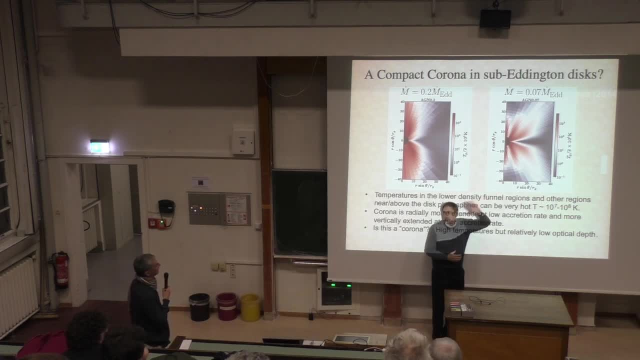 So remember, as we get towards the poles, our resolution is extremely low And, moreover, this region is extremely low density because of the angular momentum barrier that prevents material from getting to the poles, So I would be cautious about interpreting the temperature there. optical depth is extremely small. 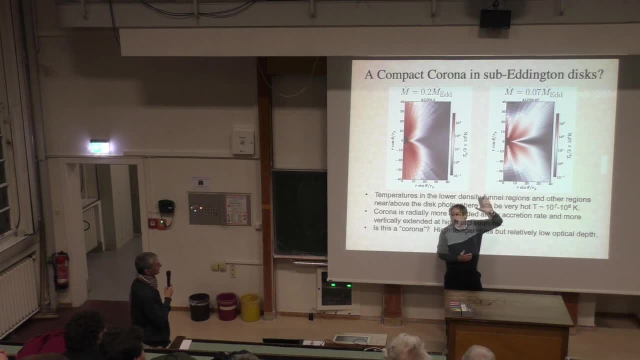 There's almost no material there, so it basically doesn't contribute to the radiation field in any way. So even when you It's not included in the spectrum, It doesn't generate anything. It's this stuff over here which is resolved in the mesh. 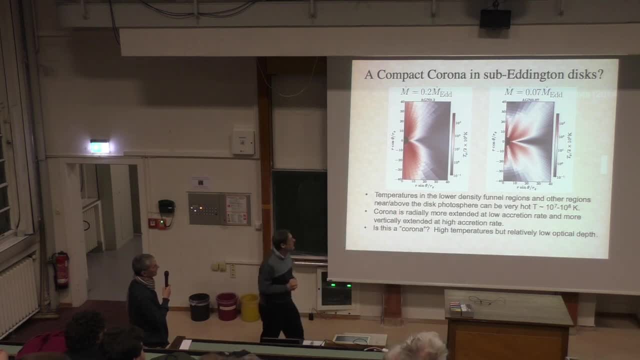 that I would believe, And that stuff is what's producing you know the. Now the other thing is: you know this other feature here. I don't know. I mean, remember this is some time average And so maybe it's the particular orbit we chose. 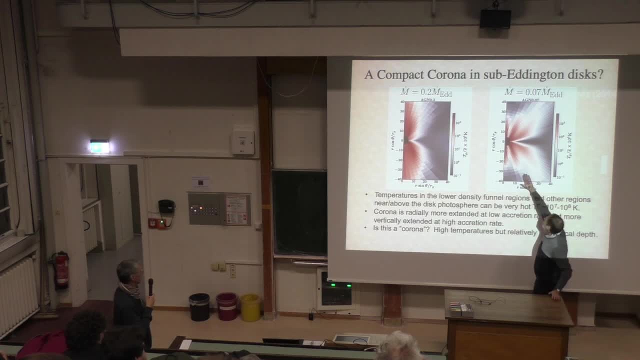 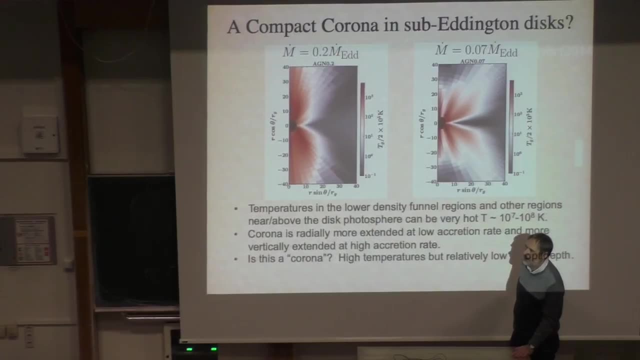 If we did another 10 orbits, would it be the same? I'm not sure. I mean, I don't put much stock in the small scale structure here, but rather just the emergence of this corrosion. I mean, you know, it's a little bit of a corona. 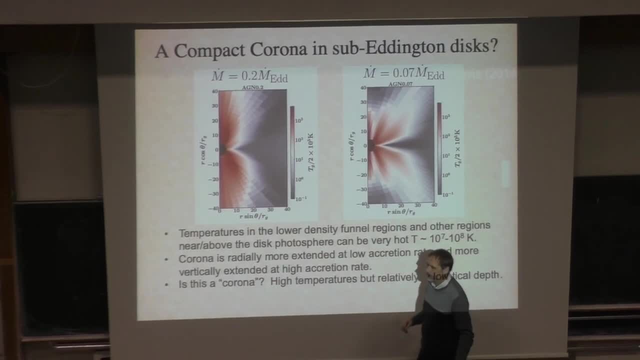 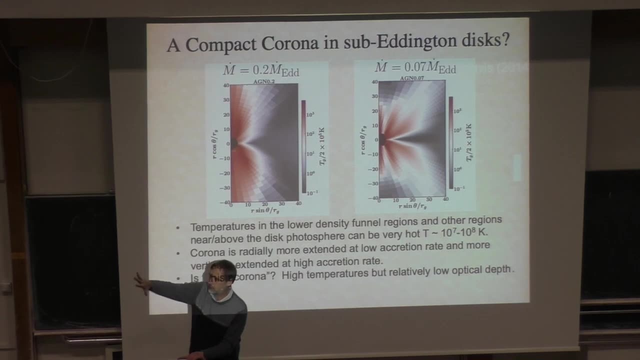 which doesn't go away, no matter what snapshots we look at. Okay, So it could be little blobs that just Could be filaments. I mean, one really important thing to realize when you look at this data is if you plot the photosphere. 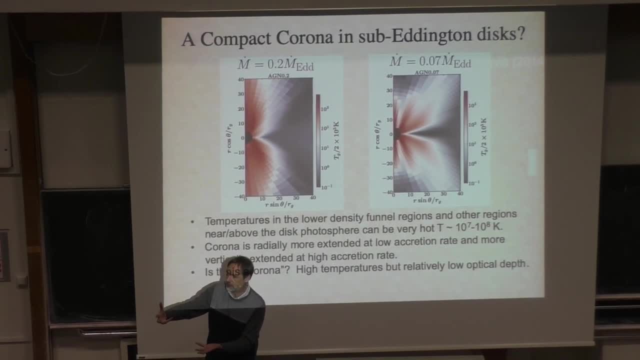 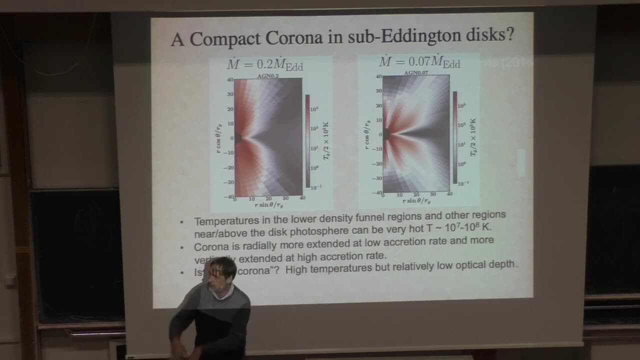 it's not a smooth surface. This is turbulence with large amplitude density fluctuations. It's Swiss cheese with blobs of optically thick plasma that are well above the photosphere and holes that go deep into the photosphere And in a very time evolving way. 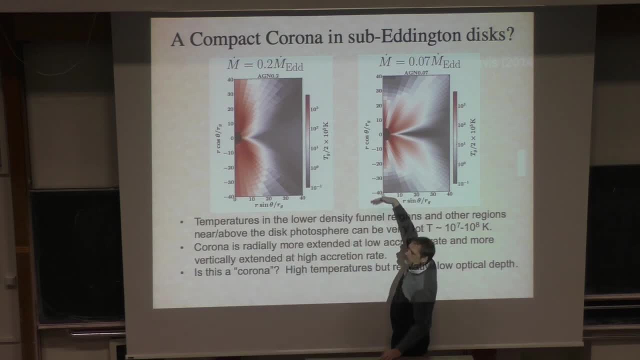 This: every snapshot looks slightly different. It could just be blobs that were for some reason a little bit higher and lower, and you know it makes simple, simple spectrum modeling kind of hard, because it's actually very, very complex geometrically. Good Thanks. 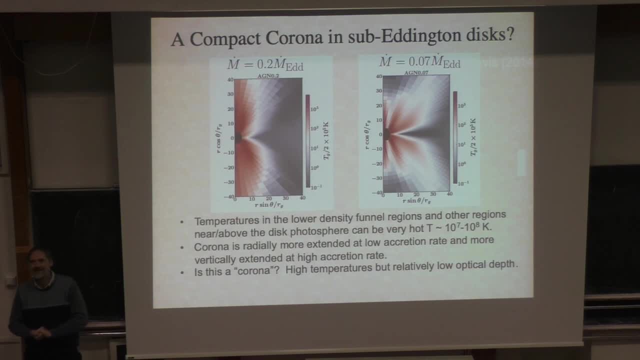 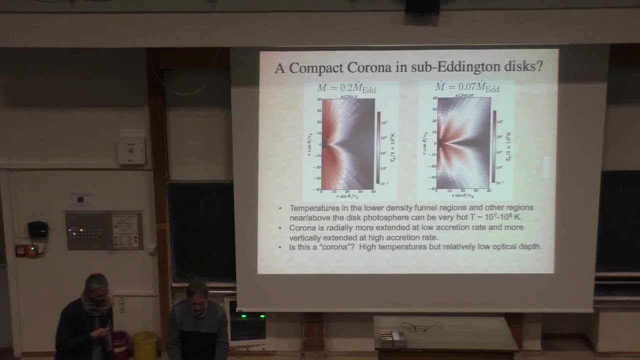 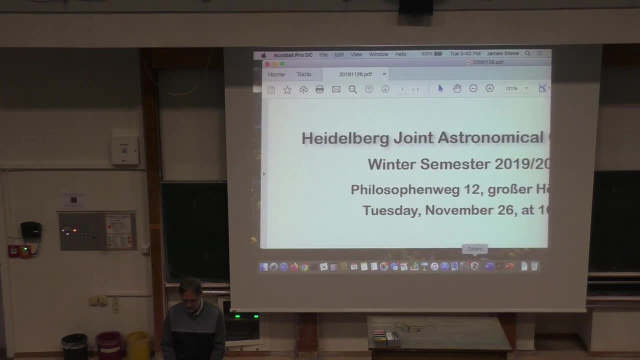 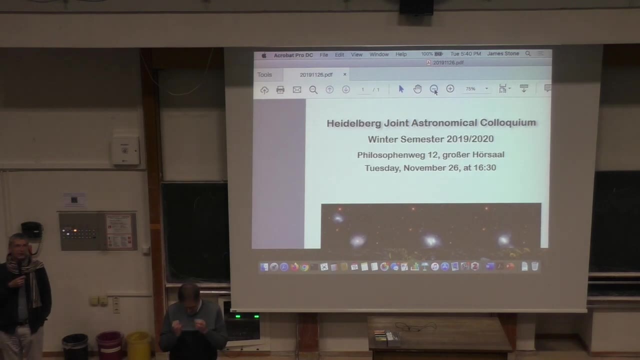 A, we have a question. We go for the conference, not conference for the colloquium dinner now after this, And it would be good to get a quick hands up. who would be interested in joining us? So one, two, three, four, five, six, seven, eight.